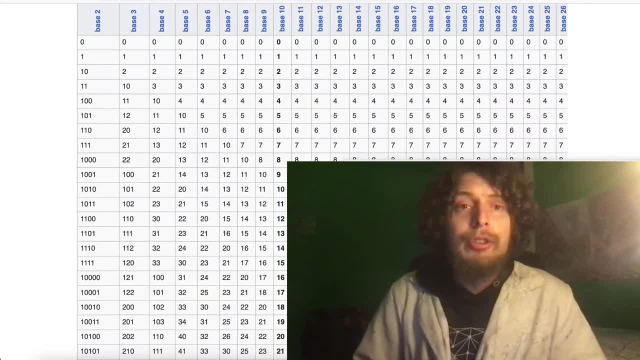 other alternate ways and another theme: to play with numbers. So if you're thinking about things in alternate, unconventional ways and playing with numbers, one of the key things to think is that you're going to have to think about things in other, alternate ways. So if you're thinking 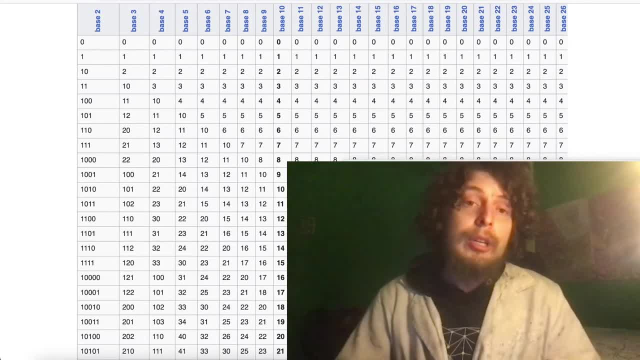 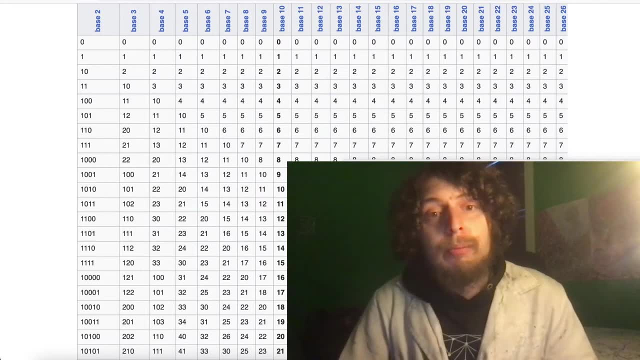 maybe we could have counted or written our numbers differently, which will affect certain traits that we discuss here, Not all of the traits. we can, in fact, categorize some traits as base independent, meaning that they exist, even if you were counting numbers on a pile of rocks. however, 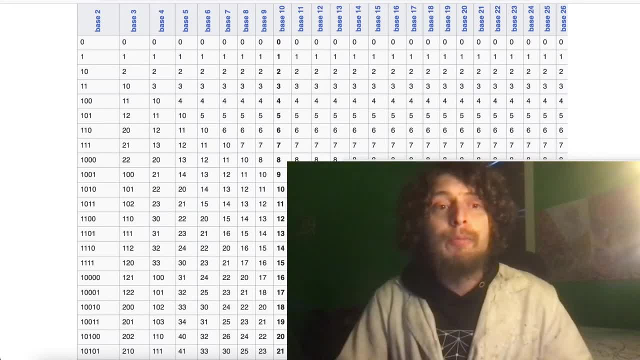 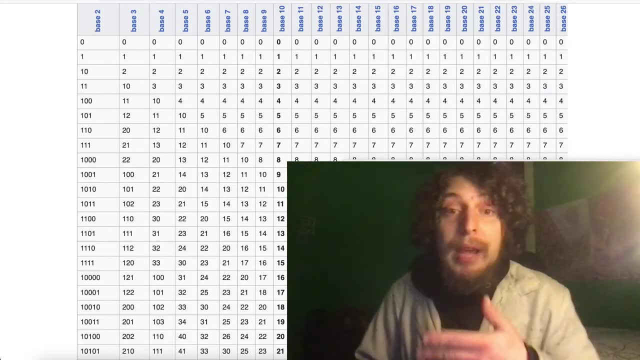 you wrote those numbers. For example, something's prime factorization for a whole number which primes make it up, is something that's base independent or whatever. If we consider numbers in this base independent, No matter how I decide to write these numbers, some of them are going to be primes. 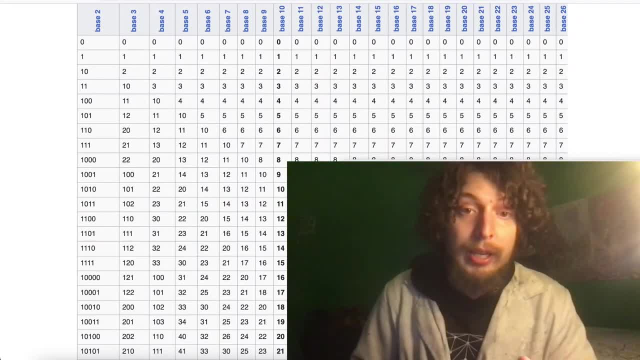 others of them are going to be composites that have unique prime factorizations. A lot of the other traits that relate to divisibility might also be something that doesn't matter what base you're in, But if you see divisibility related to something like a digit sum, then suddenly we're in. 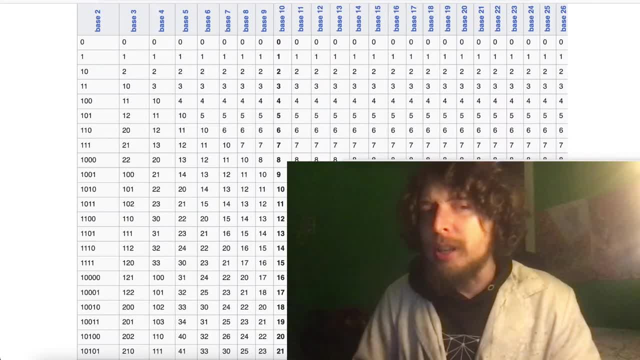 base dependent territory, Because when you hear the word digit, it gives you a clue that that would be different if I wrote the digits a different way, And so traits that relate to what digits a number has, or what those digits add up to, or what their collection includes, can be fun, But you may 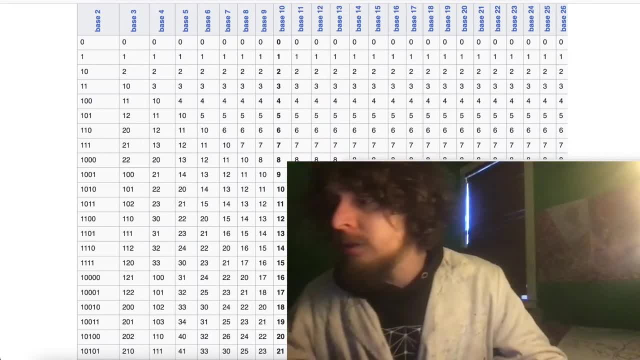 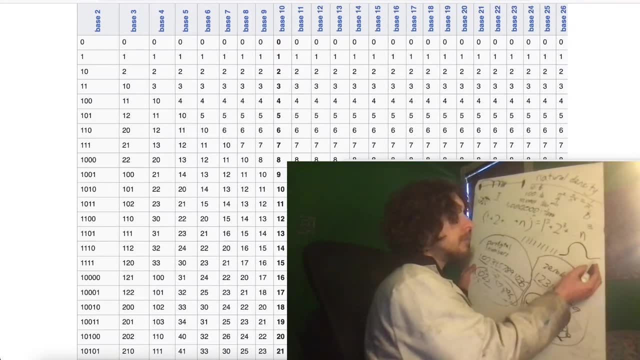 first. it's sort of like one of those joke memes where there's a curve and like the really dumb person and the really smart person came to the same conclusion and the middle person, who was, came to a different frustrated conclusion. And this lower conclusion and upper conclusion might be, if you don't know much about. 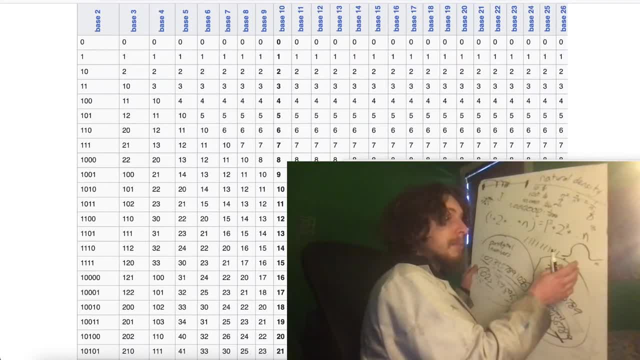 numbers. oh, it might be really cool that this thing is divisible by its digits or something. If you know a medium amount amount about numbers, it might be like: oh well, that's not as cool because that relies on the system we count in. 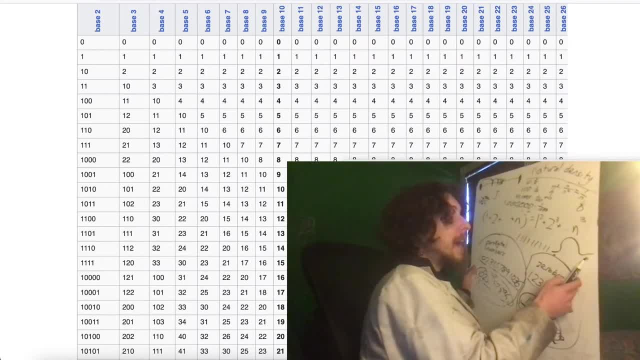 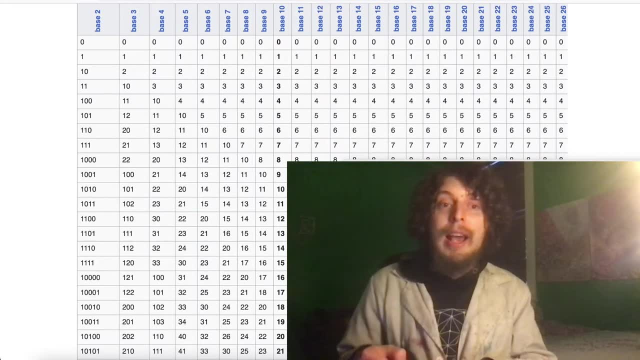 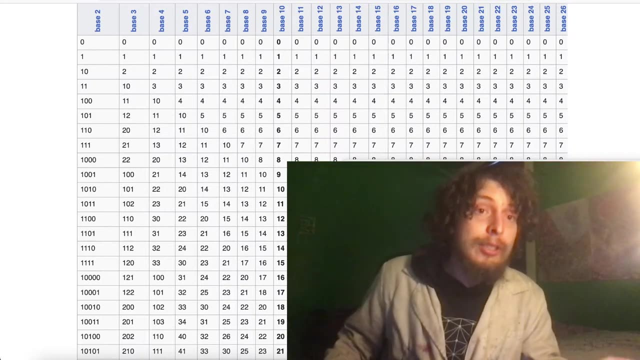 But if you look at a lot of stuff about numbers, it might go back to being like that's interesting because you can compare the traits to other ways. we could have written the numbers and see ways that certain traits maintain themself over many or even infinite ways. we could write numbers And of course we could get super abstract and 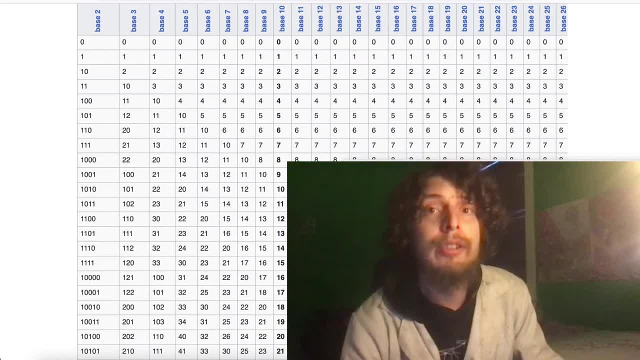 write numbers in a completely different way. There's no end to the possibilities. And if we encountered some alien, there's a good chance they would count in. and if we encountered some alien, there's a good chance they would count in. and if we encountered some alien, there's a good chance they would count in. 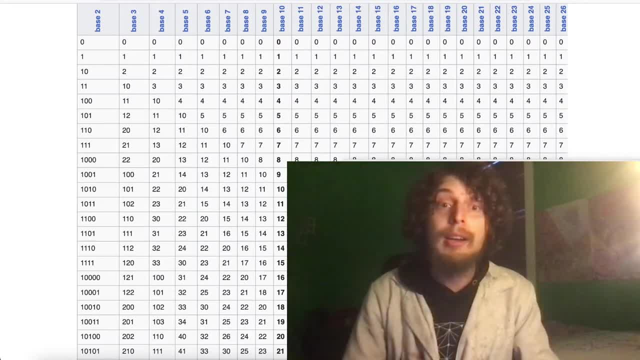 a very significantly different way. That might not be a positional numeral base, where most of the bases that we've played around with, even the strange ones, have this trait called a positional numeral base, where you're putting the same set of digits in different positions and the different positions have different values. So, and within that, a lot. 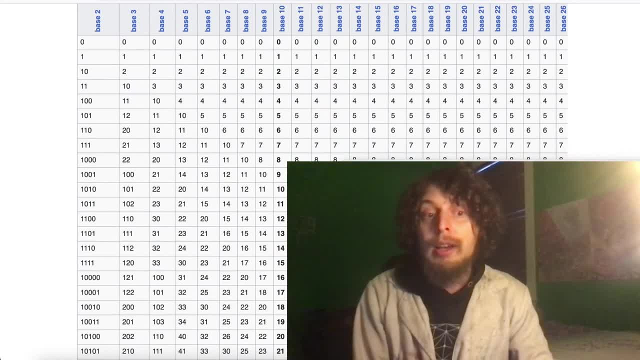 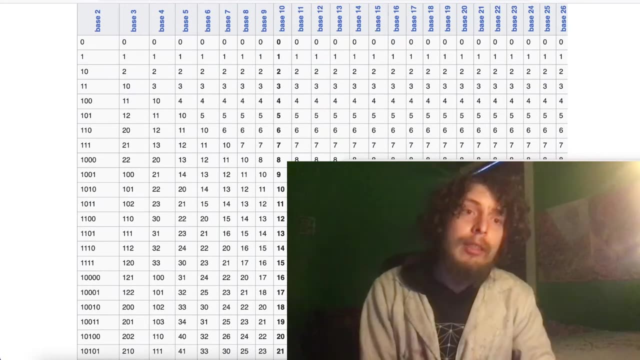 of the ones we've done. pretty much all the ones we've done so far even have those values, just be powers of a certain number. but within those tweaks we can find a lot of crazy stuff, and it is one of the logical ways to construct numbers. so it's not impossible to imagine that there could be another. 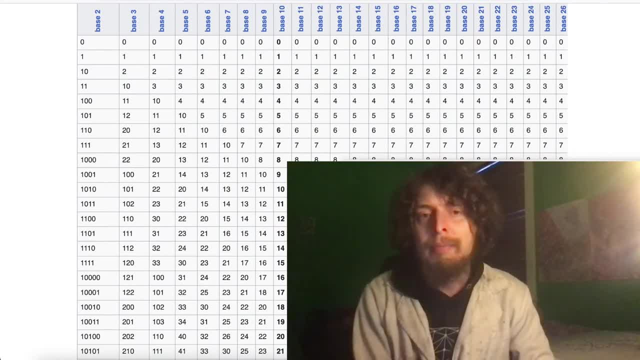 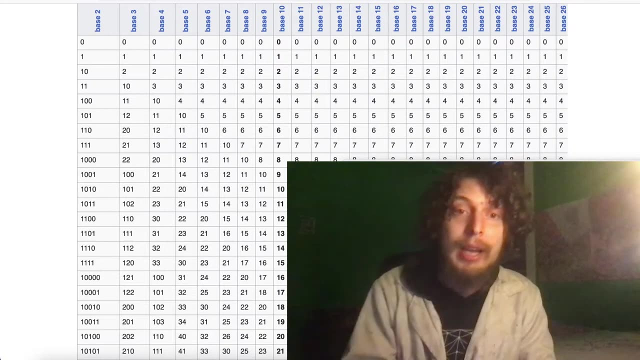 alien that counted in another positional numeral base and if there was, they probably wouldn't have settled on base 10 unless they happened to have some important 10 like trait about their body. like how we decided the 10 fingers was the important thing about counting as opposed to. 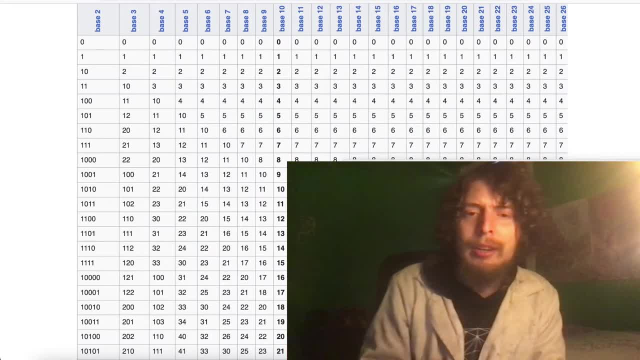 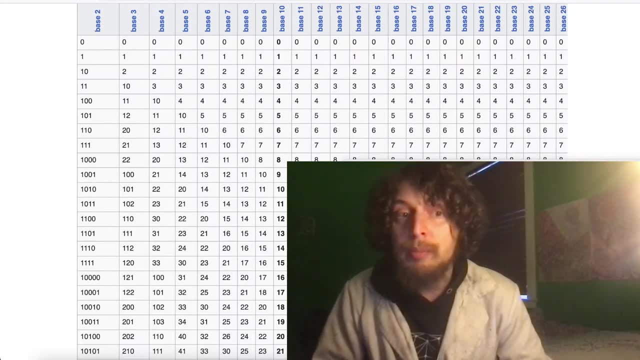 something like the finger joints that come in threes that we could have in some societies have counted on instead, and so if an alien was, say, counting in a different one of these bases, maybe they have their own pan digital numbers that contain every digit, maybe they have their. 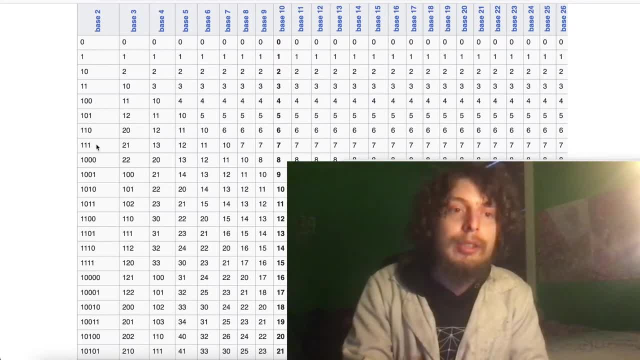 own hyper 11s, or what could be called generalized rep units that are only the digit one. maybe they have their own numbers that look round by. a round number is a name for when you have a bunch of zeros at the end and so on. so what traits do things like that have over the course of many bases, and are there some? 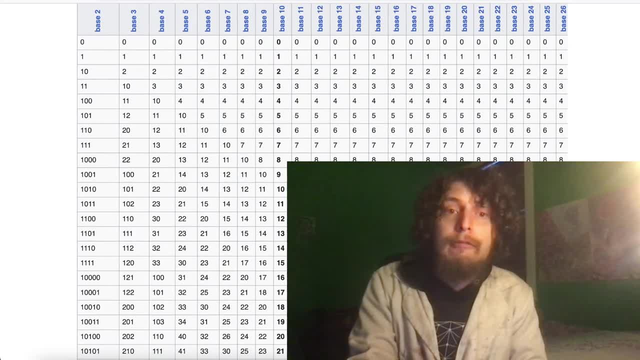 numbers that have traits that happen in every base, or traits that happen in more or less bases than the average number would. well, yeah, there's a lot to investigate there, and- and we'll start with a few families of number that we've looked at in the past and 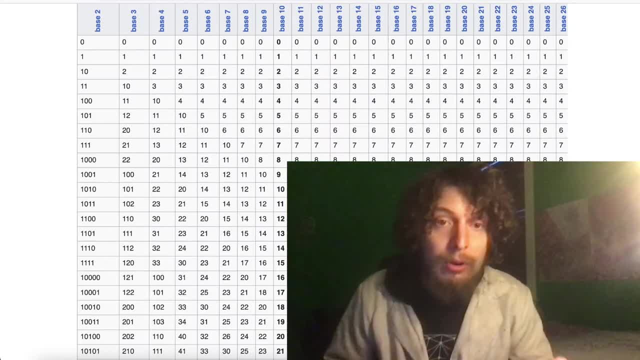 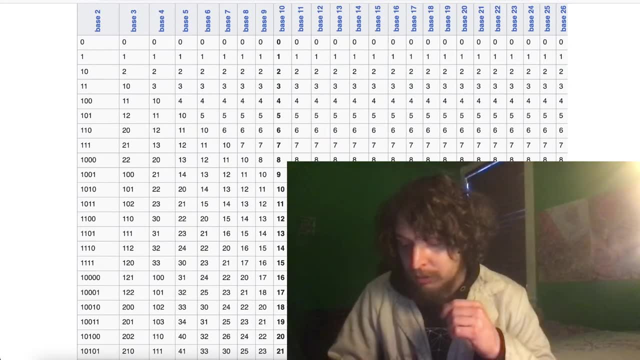 let me also take a peek at the comments real quick before i jump down many rabbit holes of things i want to talk about and share. thank you to everyone who's joining me and whoever has to go and watch us later. that's all good. i'll even add time stamps later of the chapters. so 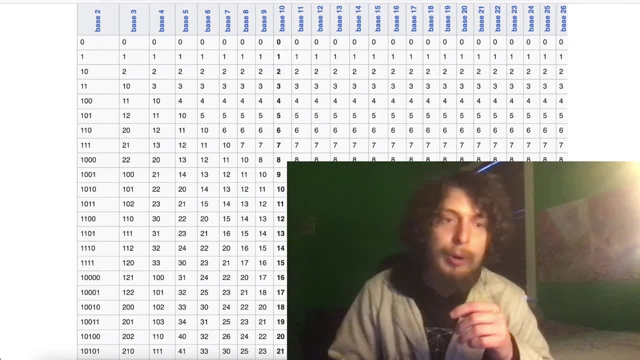 people who can only watch part of it later can see what other parts they want to catch up on, and all of you are awesome. thanks for joining this. what we're going to first start with is one of the most obvious ones, which is what numbers would be round, as you might say in. 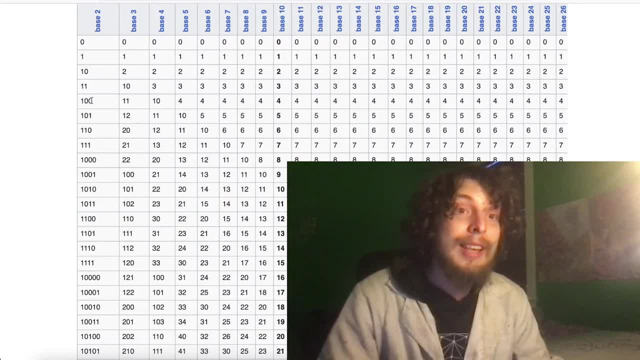 a given base- which is a term for the numbers that usually applied to our base- have a bunch of zeros on the end, and it doesn't have to mean something like one thousand. two thousand could be considered still more round than like 21, 35 or something, and the numbers are. we could. 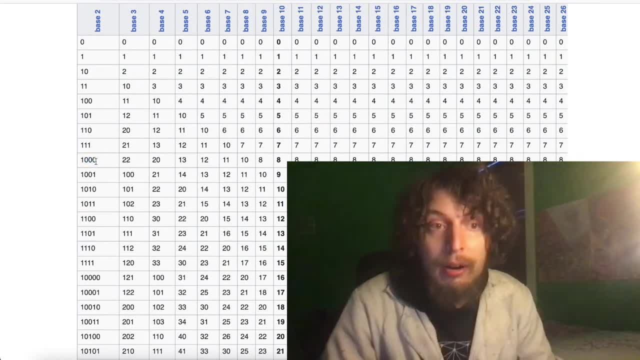 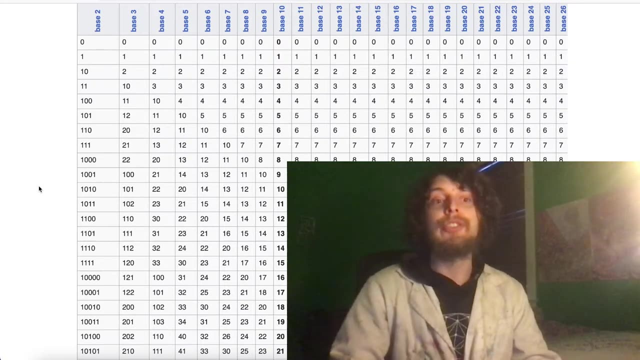 categorize how supposedly round they are based on how many zeros they have at the end, which in our base of course means how many powers of 10 are included in them. and what that really means in our base is that the prime factorization of the number has that many twos as well as that many fives. 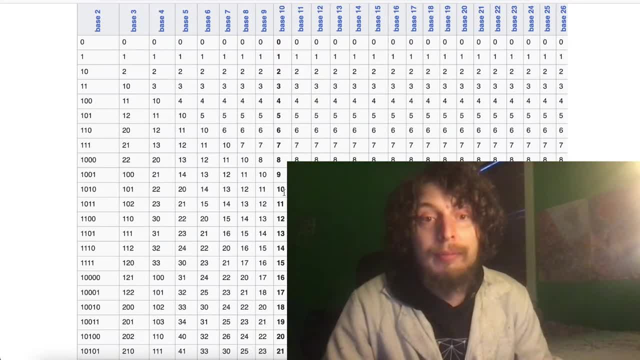 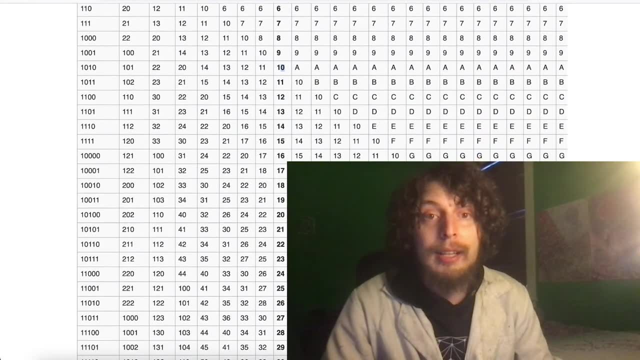 so, for example, the number 10 is the first number in our base with any zero at the end, not counting zero itself, and that's because it has a two and a five in it: 100, the first number with two zeros, or any number with two zeros at the end, has amongst its prime factorization at least two, twos and at 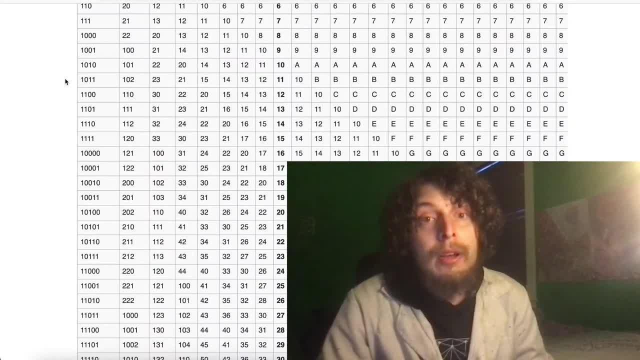 least two fives. now in other bases it's just going to mean it's round based on having more than one number. so, for example, if you go to the first number of a prime factorization, you could have two zeros and a five, and it has one and a five in it and it's a two and two zeros in the. 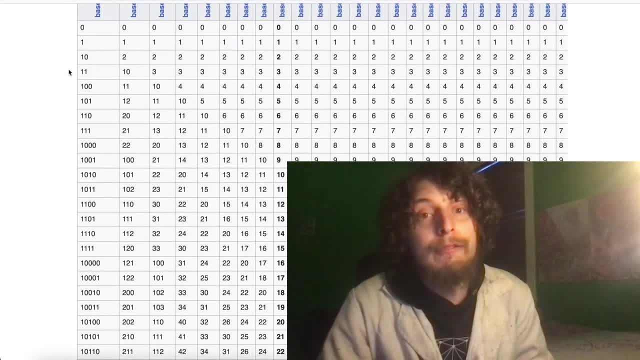 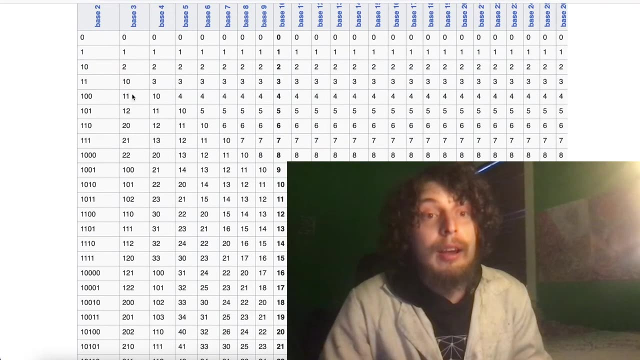 prime factorization. and if you go down to prime factorization you could say: whatever primes make up the base number. so in binary, for example, a zero just means it has a two in its prime factorization, two zeros means it has two twos in its prime factorization, and so on in base three. 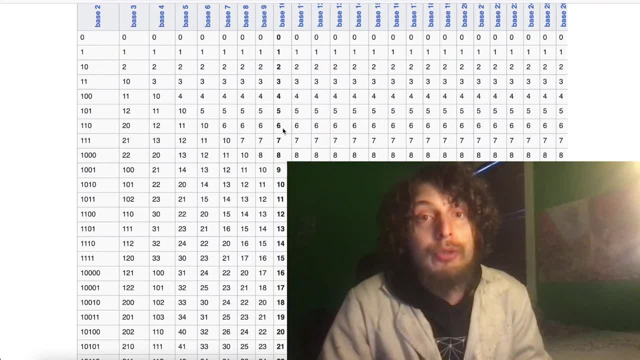 we would say: oh, these numbers 10 and 20 have a zero at the end because at the base 10, you know, bolded one here just for a reference point for you to understand. their amount is four of a thing or eight of a thing. uh, oh, that was base four. the base three: 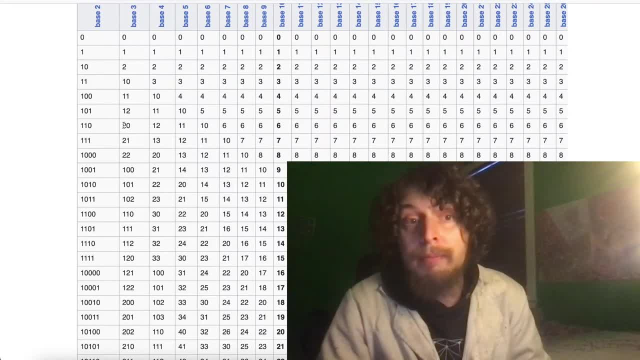 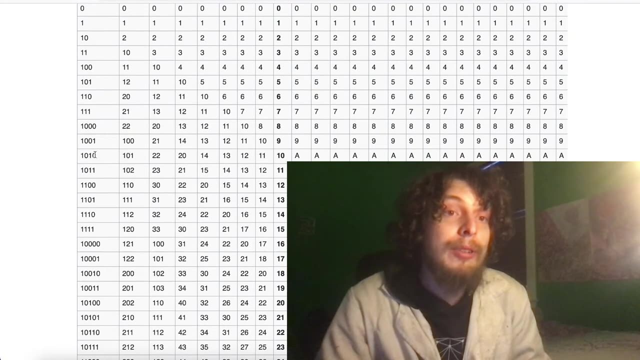 ones. their amount is three of a thing, or six of a thing for 20.. that's because those are multiples of three. oh, and here look, you get two zeros at the end because we're at nine, which is two times a three is in its prime factorization. so the round numbers are pretty clear. they're how many times? 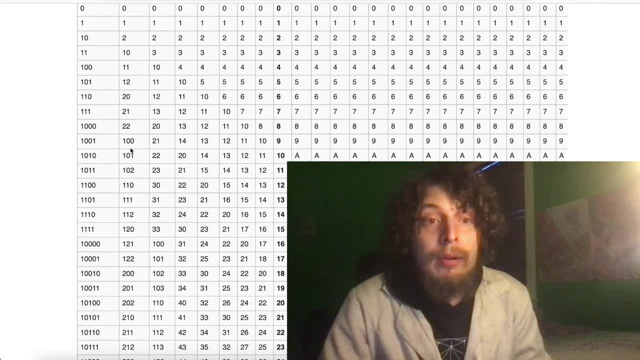 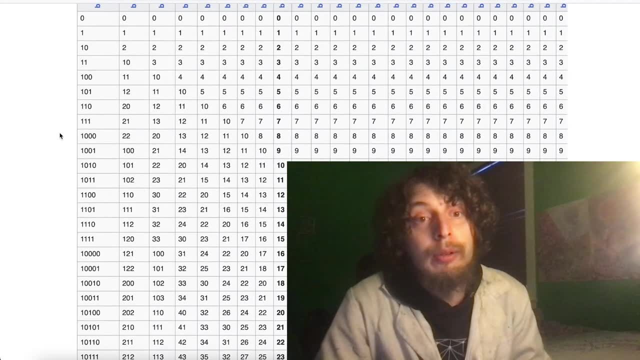 the base number is a multiple in there. but what about the numbers that aren't like one: zero, zero, zero, zero? the numbers that are only ones that some would call a generalized rep unit? i like to call a hyper eleven, those numbers we could say: have one one, then one of. 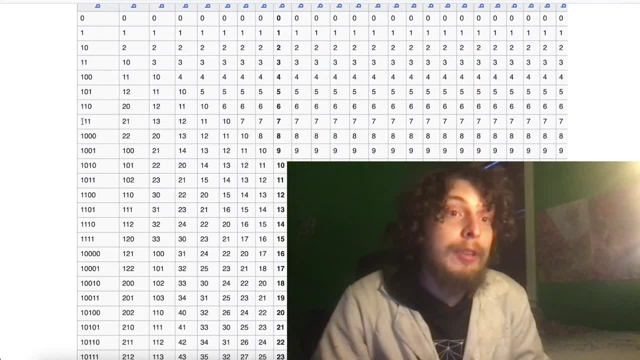 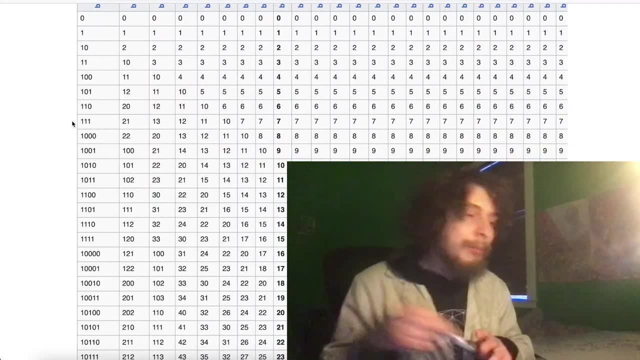 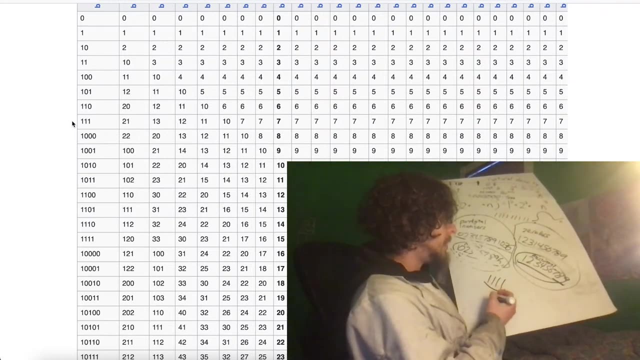 the base number and then one of the base number squared and then one more of the base number squared, and so on. so like, basically, the number of one, one, one one interpreted in different bases is going to be numbers that can be the result of one plus the b number plus the b number squared. 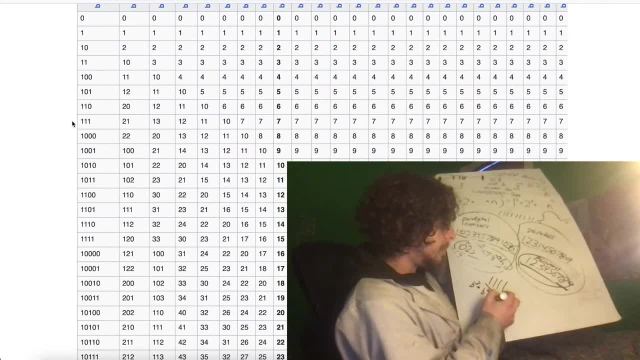 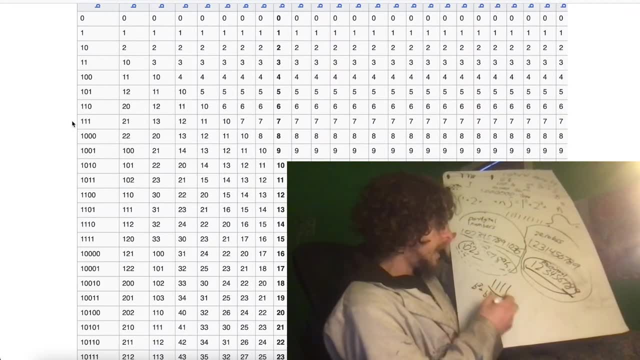 plus the b number cubed, which these have 1 as a coefficient. but we don't need to write the 1.. And for example, in base 10, if I plug in 10 in there, I get the number that we write like that: 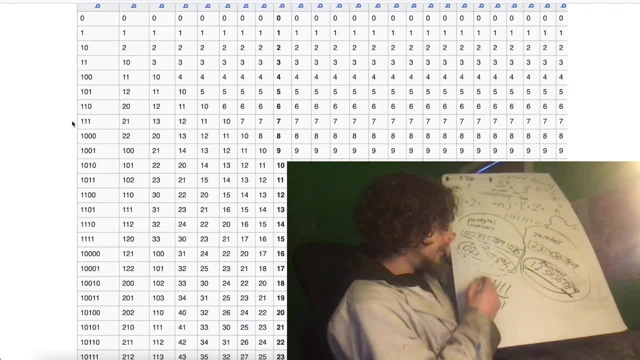 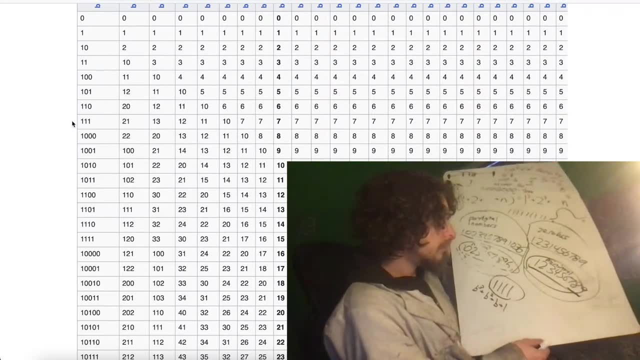 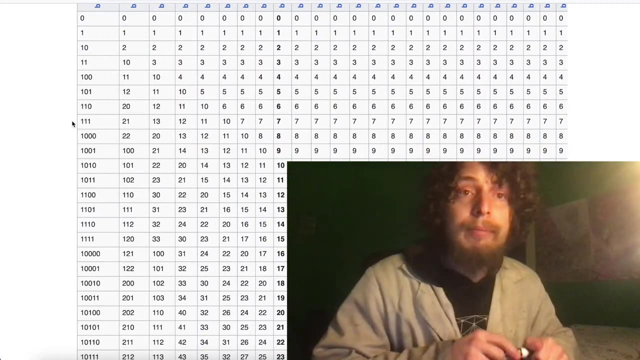 But if I plug in 2 in there, I get 8 plus 4 plus 2 plus 1 is 15.. And that is how binary writes 15.. Now with the hyper-11s- although they have a formula, and they in fact have other formulas- here on the OEIS, where they have some cool tables we'll look at. we can see the generalized rep unit numbers. Their formula can be simplified to this: to b, to the n minus 1 over b minus 1 for a base number b. 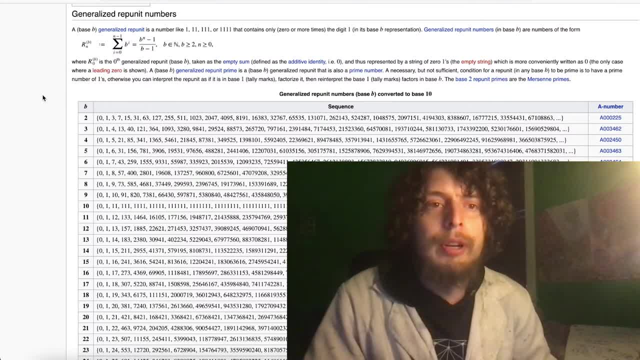 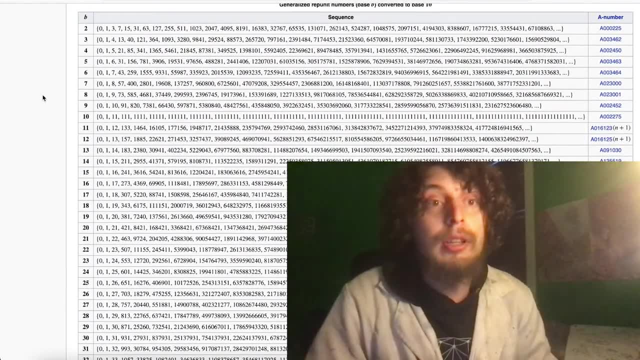 And although they have some simple formulas we could write them in, they have a lot of cool patterns and mysteries. The ones that are primes are very investigated. There's a lot of sequences noted down, Like if you go on Wikipedia for rep unit. 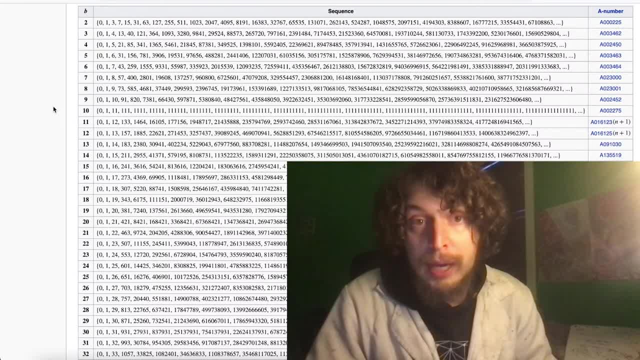 they talk all about hyper-11 primes in different bases And that's partially because the prime ones in base 2 include the biggest primes ever discovered. So 9 out of the 10 biggest primes ever discovered and the top 8 include some of the biggest primes of all time. 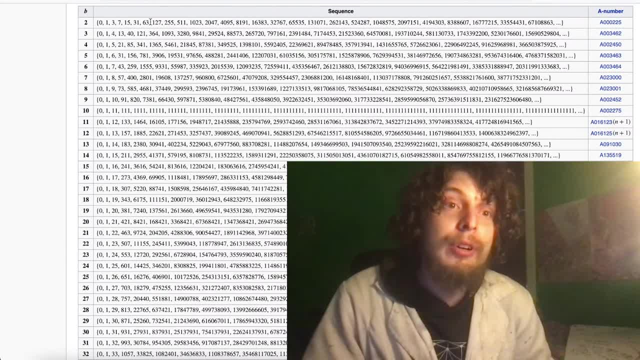 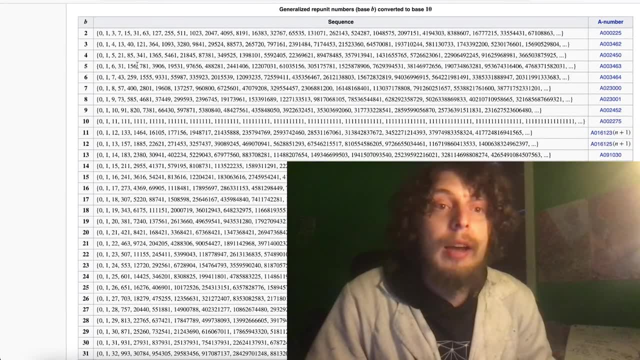 So that's why they're called hyper-11s. Now let's take a look at some of the hyper-11s that we've discovered, Our hyper-11s in binary. Now, in this list they're showing us: converted to how base 10 would write them which numbers are hyper-11 in that base. Now, first you get 1, after they put 0. also because 0 technically fulfills the formula, although it doesn't count for our definition. 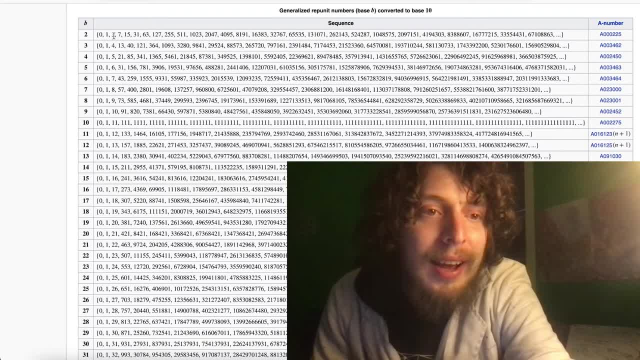 1 is 1 in any base here And this column is 1 more than the base number because that's the 11 in any base. The number that the base would write 1, 1, comes out to 1 more than the base number. 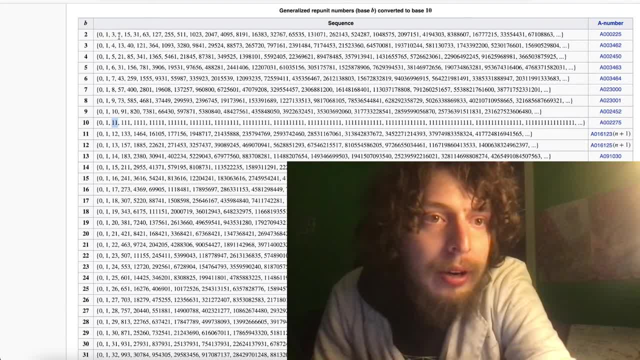 Then the third or fourth, if you count the 0 number. here is what 1, 1, 1 would mean in these bases. We can see: base 2 has 1, 1, 1 at 7.. Base 3 has 1, 1, 1 at 13.. 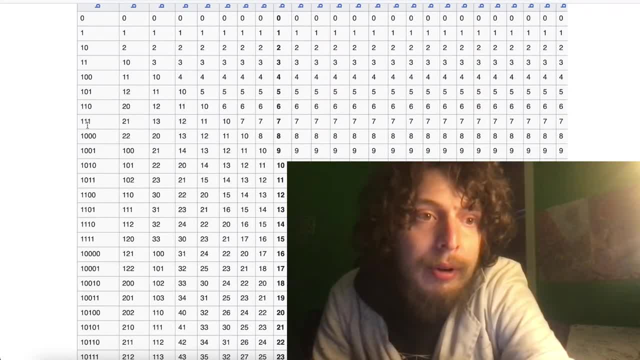 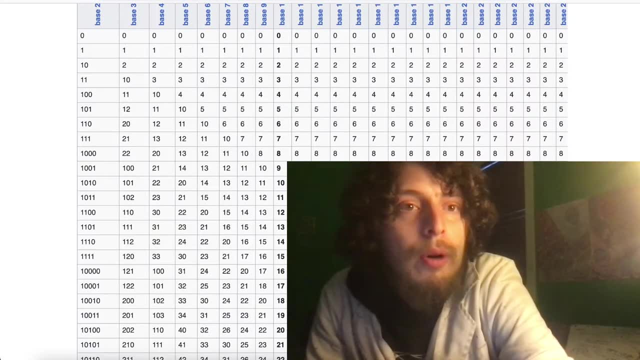 And going back to the table, we can see that's true. 7, we write 1, 1, 1 in binary 13, we write 1, 1, 1 in base 2.. Now one question you might have is: 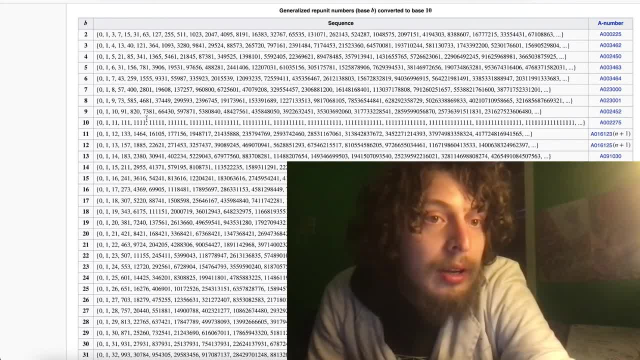 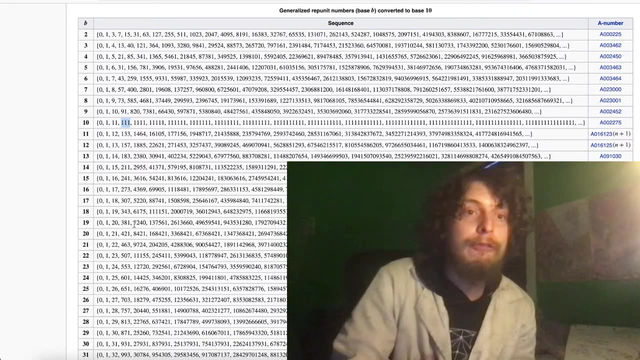 are there any numbers that show up on multiple of these lists, not counting the sort of a trivial 11 one? Are there any that are the third term, not counting the 0 or further, that show up on multiple lists? And, like I have mentioned before, it is conjecture. 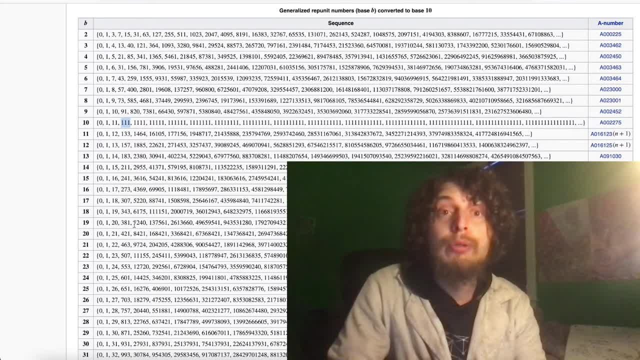 But not proven, that there are only two numbers of that sort. The numbers include 31,. which 31 we can see is which term is that Is 1, 1, 1, 1, 1 in binary, And we can see 31 is also 1, 1, 1 in base 5.. 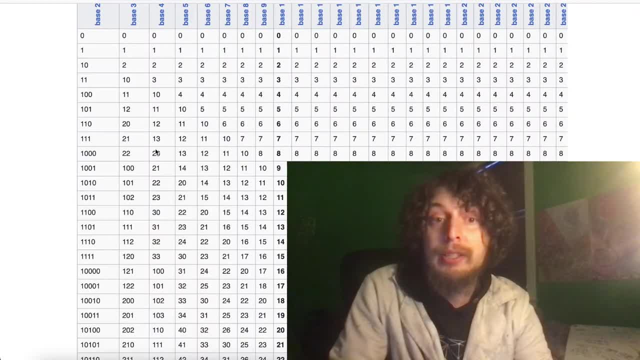 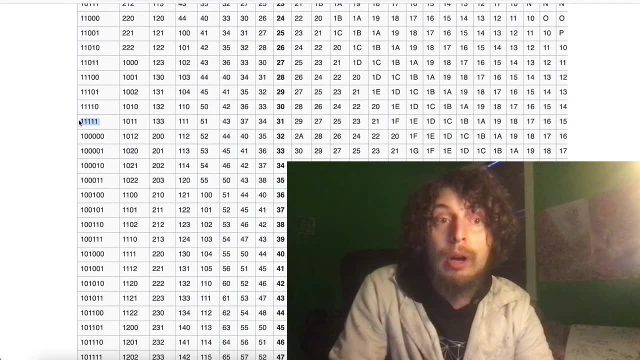 Now let's see that on the table of bases, If we go down to 31 here, it has 1, 1, 1 there and 1, 1, 1, 1, 1 there. And if we look up the conjecture real quick, 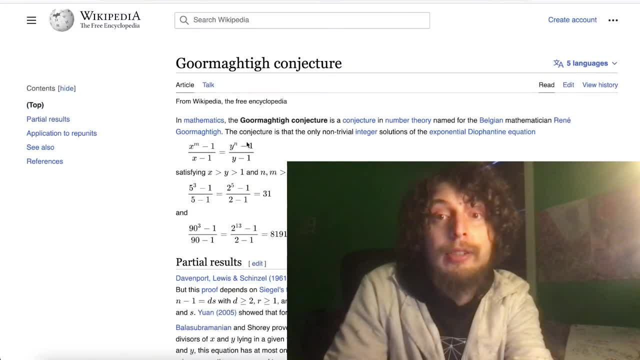 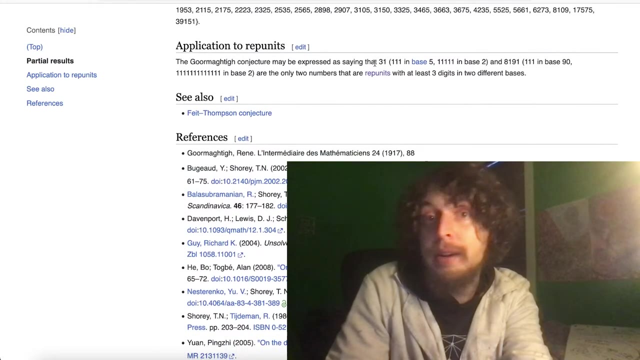 we can see that it's written in terms of that generalized equation. They're saying the only non-trivial solution to this are 31 and 8,191.. And we can see that it also may be expressed as saying that 31 and 8,191 are the only two numbers that are rep units. 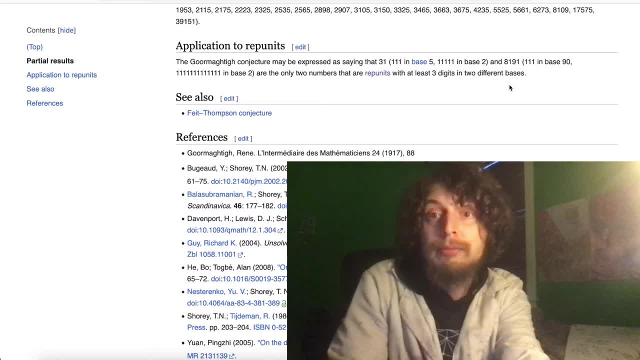 with at least three digits in two different bases And this wouldn't show up in our chart there because they didn't include it. They didn't include base 90, but that's the other one. Hasn't been proven yet, but it's a very interesting question. And it is conjectured, because they've tested many numbers and they have some reasons to think it could be true that amidst the infinity no others line up in this way. But staring into infinity, sometimes you can prove things and sometimes it's hard. 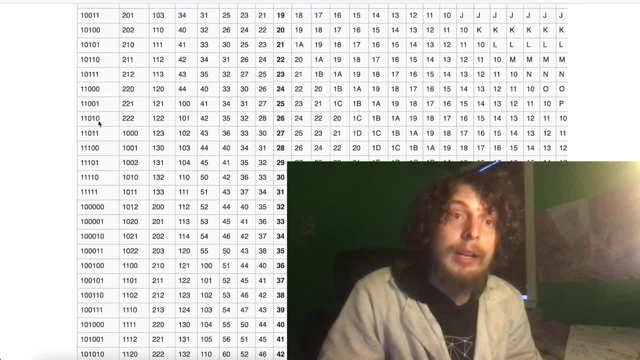 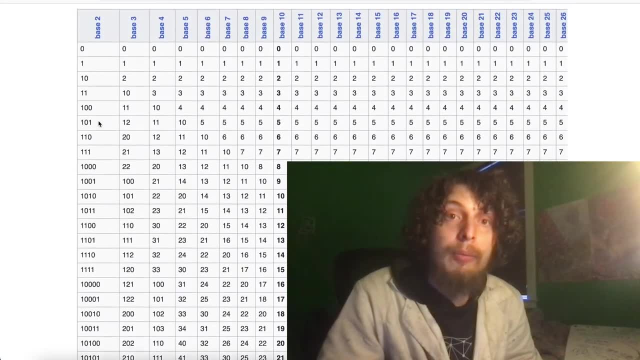 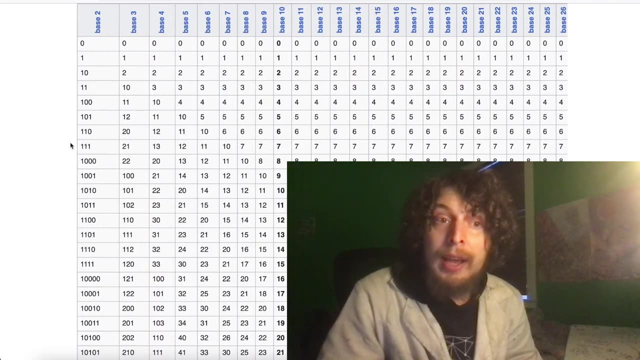 So back to the table of bases. There are a bunch of bases here. There are many other open questions about these hyper-11s, Some of the main ones being, like I said, are numbers, that in how many bases, or multiple, and whether which ones are prime numbers. 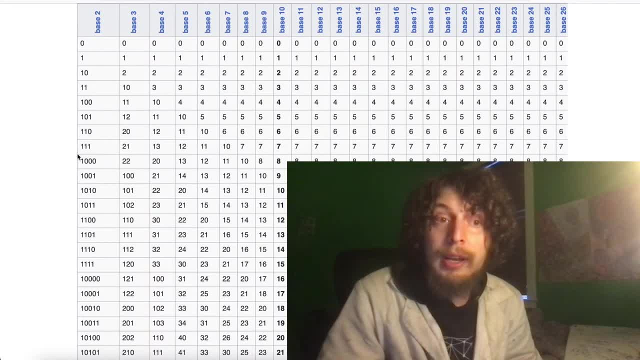 And you could find other interesting traits, of course, to investigate, like I have and like I will, because these hyper-11s keep showing up in all sorts of different episode topics, even when I don't plan for them to, And the other topics that I'm going to talk about today. 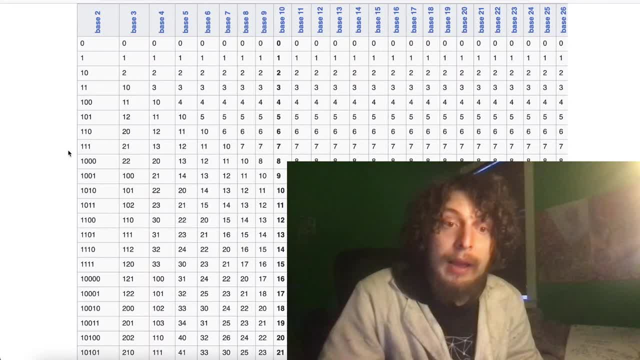 and the other topic we could talk about number-wise here is pandigital numbers. Pandigital numbers are the topic that is in my newest episode on my main channel And, without spoiling the end thesis of that, because this will cover some other topics here- 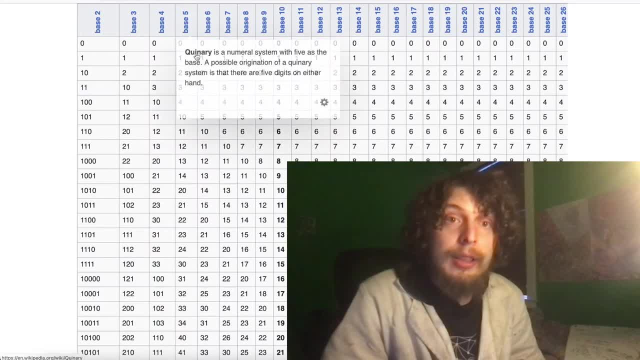 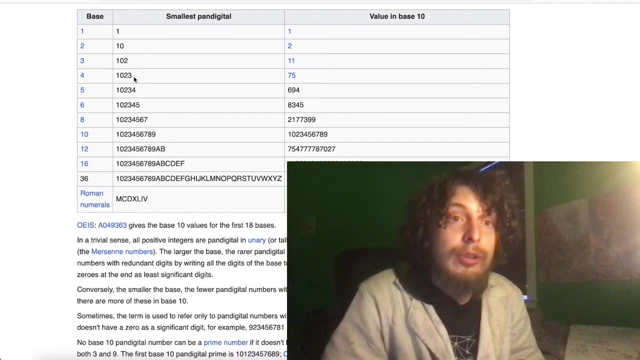 pandigital numbers contained every digit in the base at least once, And here on Wikipedia they have a table of the smallest possible pandigital number in a given base translated into base 10.. Now we can see that in binary 1, 0 fulfills the conditions. 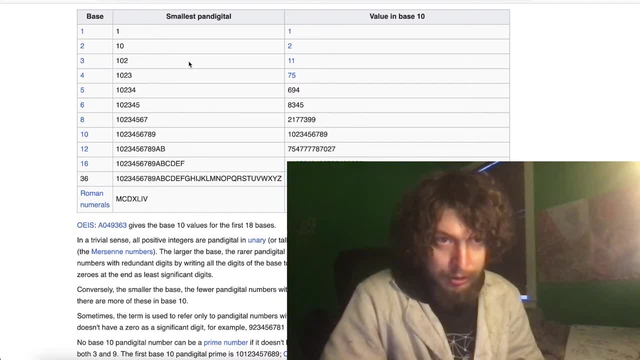 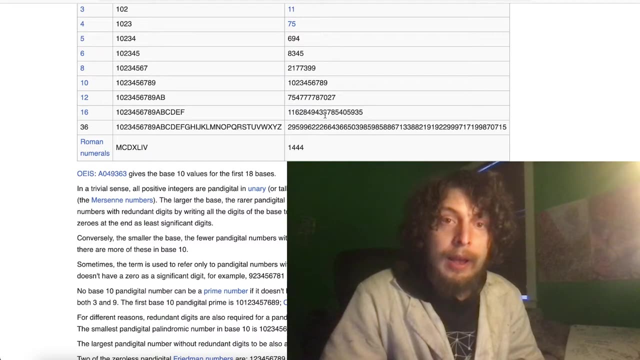 and that's 2.. In base, 3, 1, 0, 2 is the smallest, which we would say is the number 11. And then 75 is the next one. So this is an interesting sequence, And we also could look at all sorts of traits. 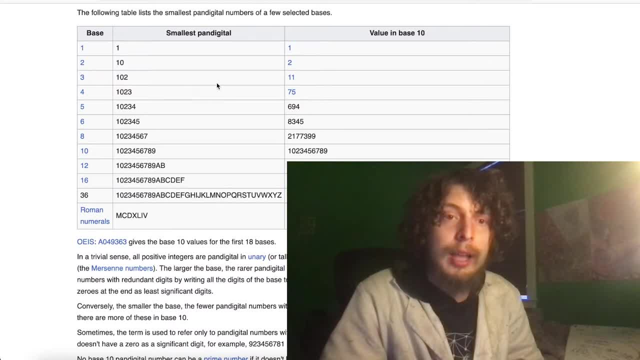 of which numbers can be pandigital and line up with a certain property, And we covered many interesting properties in the first, maybe third, of the episode of my main channel where we just looked like in base ten. here are some interesting numbers and some traits they can have. 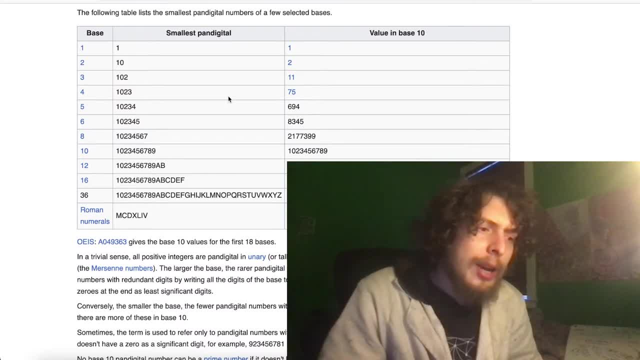 One trait to note was I mentioned something called persistence or persistence Persistence, where pan-digital numbers can generate new pan-digital numbers with their multiples, where twice the numbers still pan-digital in the base, three times the numbers pan-digital in the. 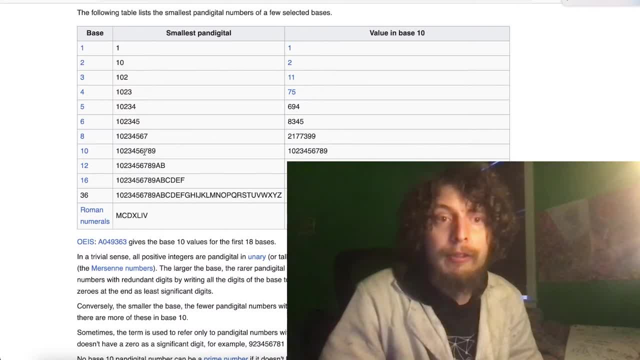 base And it's been proven that in base 10, you can have persistent numbers of an arbitrarily large persistence. So you could have, like a million persistent number that its first million multiples are pan-digital, but you can't have an infinity persistent number because that would 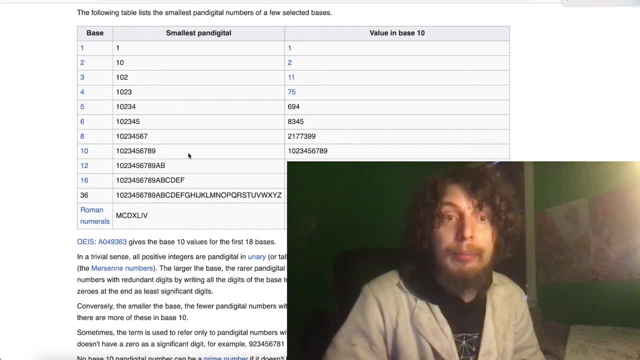 mean that you never will hit a multiple that's not pan-digital. So, strangely enough, you can have numbers that their first 1 trillion multiples, or any number you pick, are pan-digital, but eventually, on their way to infinity, will hit a non-pan-digital. However, a comment pointed out: 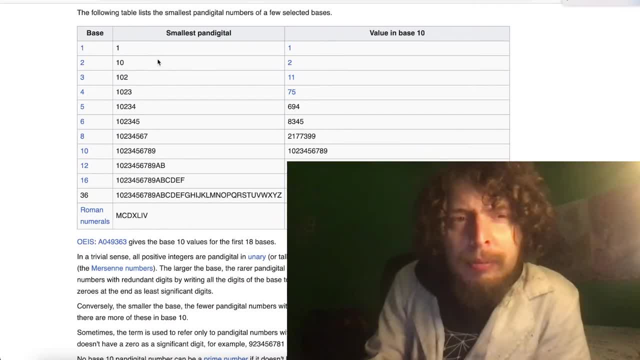 in base 2,. maybe that's not the case And it took me a second to realize, but yeah, maybe in base 2,. when you have numbers like this, this number should be infinity persistent, because if I multiply it by two, I'll still have a zero at. 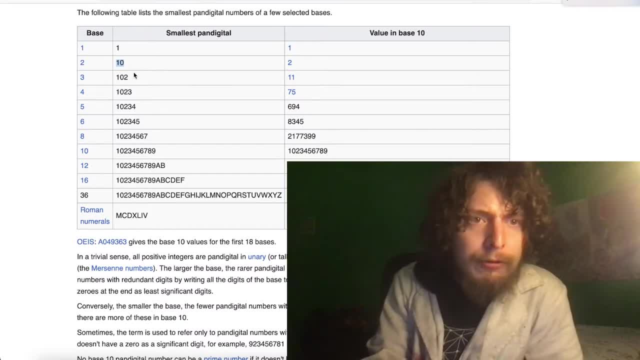 the end And no matter what I multiply it by, it will be a multiple of two and it will keep a zero at the end And it will also have a one because it's not just the number zero. So I believe that comment may have been right that in binary you could have infinity persistent numbers. 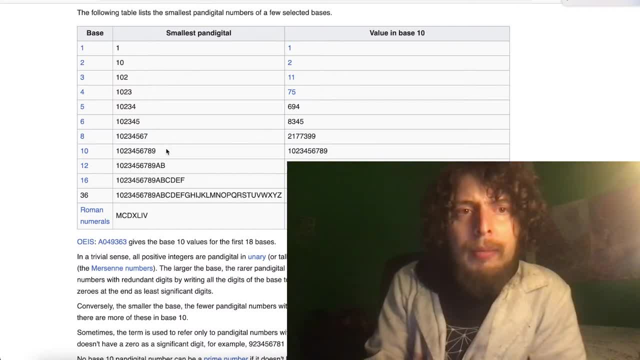 even though that was proven impossible in base 10.. It makes me suspect that in base 3, it would follow the same property as base 10, but I haven't looked into it yet. So if anyone looks into persistence, which we will call pan-digital persistence- around here, 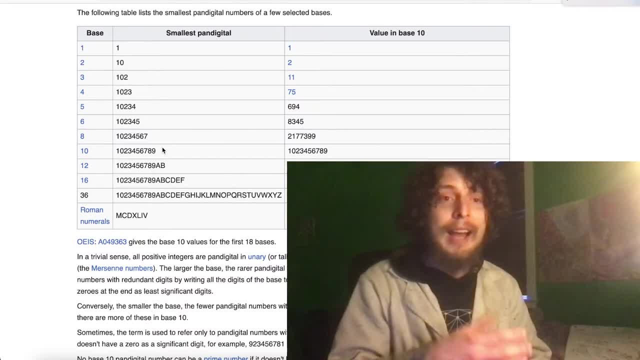 because there was other types of persistence, like ones called additive and multiplicative persistence will show up in a future episode, So we'll call this pan-digital persistence. If anyone looks into how other bases behave with that, let me know Other things that any people 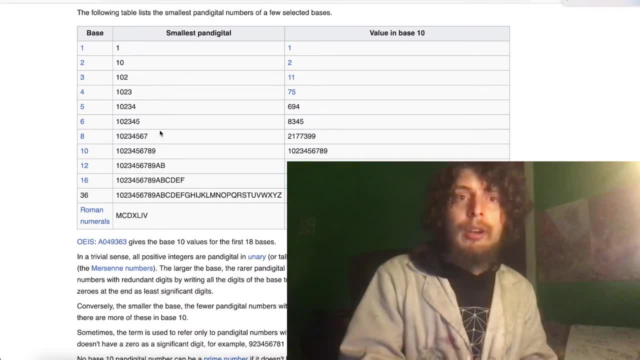 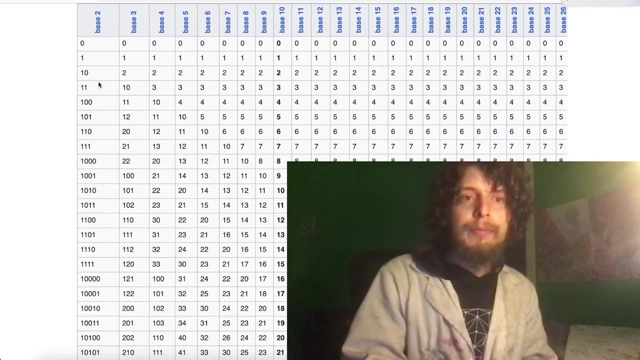 could look into. that I'm interested in is: could we classify highly pan-digital numbers, sort of like we classify highly composite numbers, meaning on our table of bases? If I look at the number two, that's sort of the first non-trivially pan-digital number. 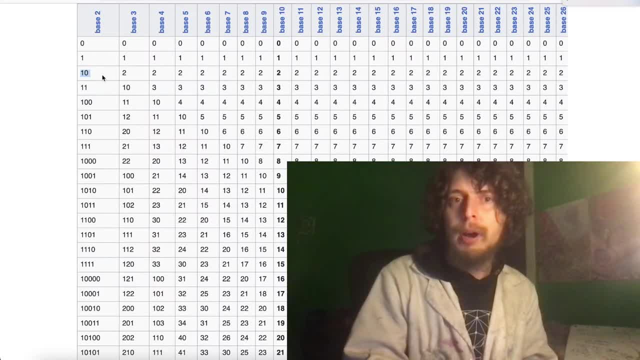 We're going to say it needs to have multiple digits for this particular part. Let's say it needs multiple digits and needs to have all the digits in the base. So we're not including what they all, these ones here, you know. so in base two, that's pan digital, but we're not going to count the 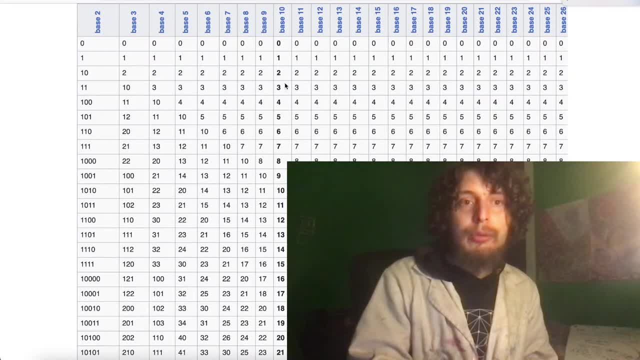 single digit ones here in base. three, of course it is again because they all will be one oh, in some base. but when we get up to four, that's pan digital in- well, no, that's only. uh, let's see, it's only pandit- well, no, let's see. three: isn't pan digital in any, actually, this is just a trait. 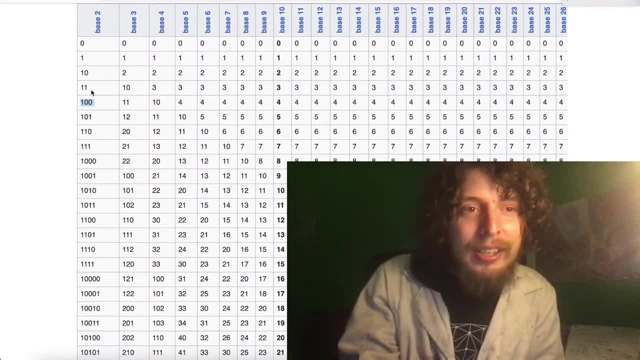 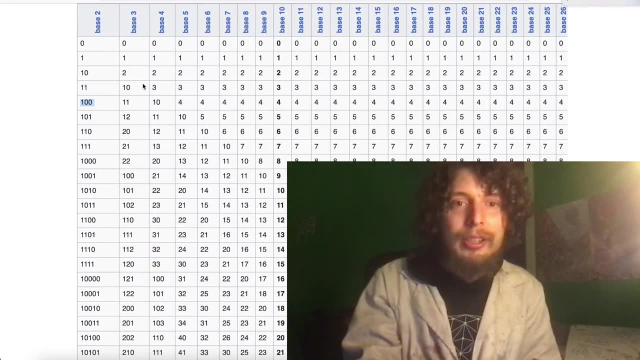 it's not in the episode that i was looking at today. three would need a two in these in base three or need a zero there. so three is actually pan digital in less than two, if we're not counting the infinite amount of single digit ones. four is back to being pan digital and binary, but not these. 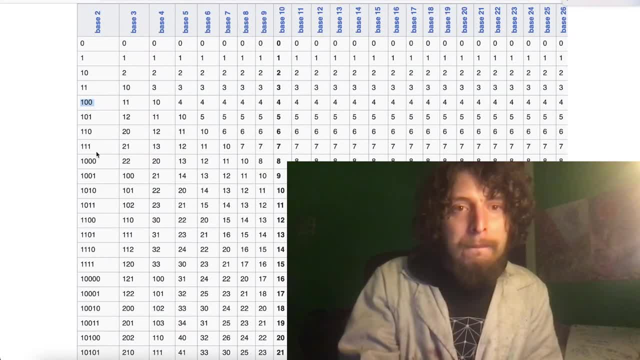 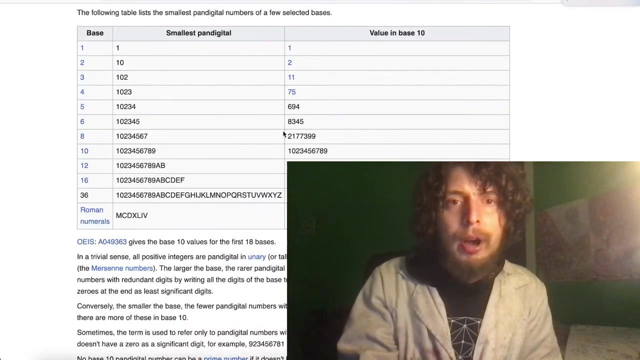 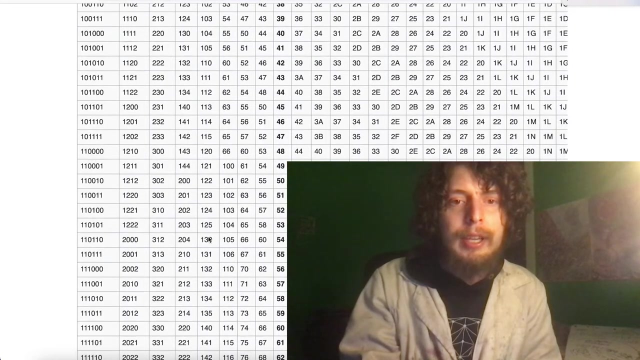 five is also pan digital and binary, but not these. where are our first numbers that are pan digital in multiple bases? for example, here: 11 was pan digital in base three as well as base two. i guess we'll have to refer to this list and see that possibly 75. it'll take that to be panned digital in base four. we have to check if 75. 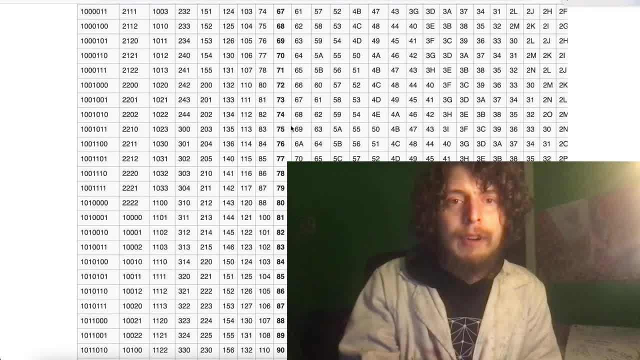 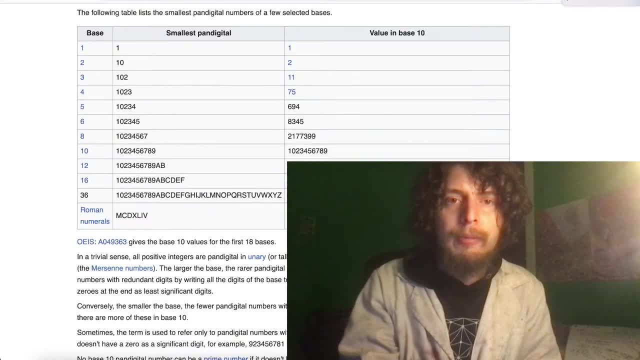 is Pandigital in the others as well. 75 is Pandigital in binary base 3 and base 4.. We don't have the guarantee just from this list that these are Pandigital and all the bases leading up to that base. So that's something I was curious about. if any programmers want to mess around with, 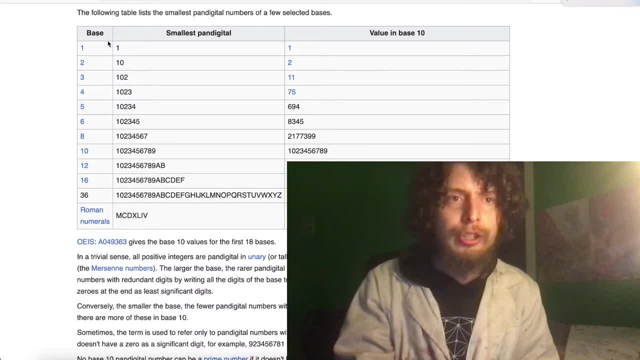 Could we classify a series of highly Pandigital numbers? May have been looked into before- I haven't looked into it much yet online, but just a question that popped into my head today. Could we make highly Pandigital number lists of numbers that are Pandigital? 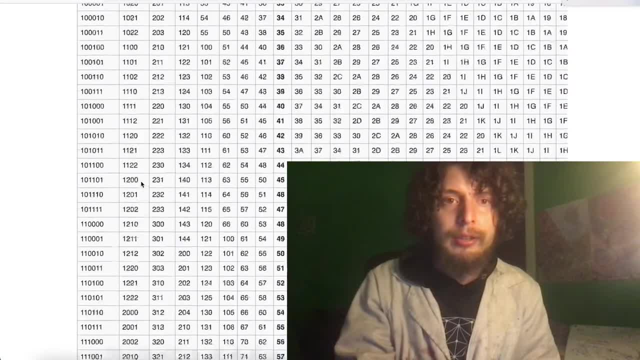 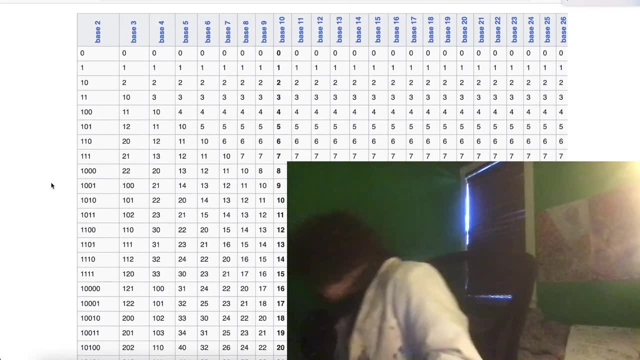 with multiple digits in the most amount of bases for any number up to their size. And let me plug this in: My computer is getting low. Got to keep the stream alive. Now I'm going to take a peek to look at the comments again and then we're going to move on to 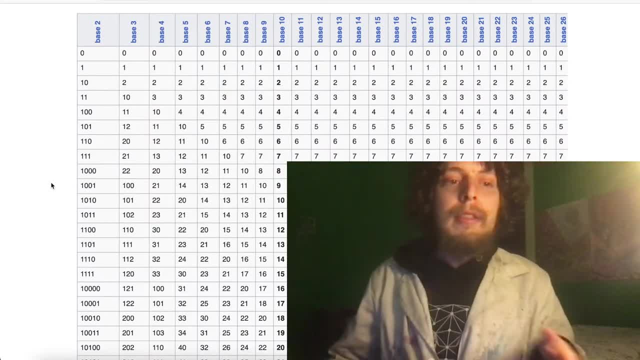 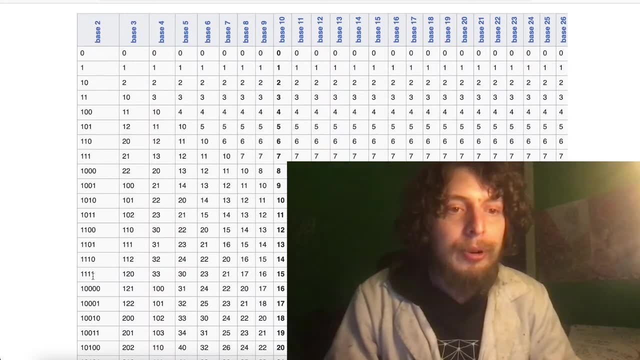 those are some ideas. first, about things that a number trait could have if we're looking for like: am I Pandigital? Am I Hyper11?? Am I this round type of number? And, as you will see in my full episode on my main channel or, for those who have already seen, that which is linked in the 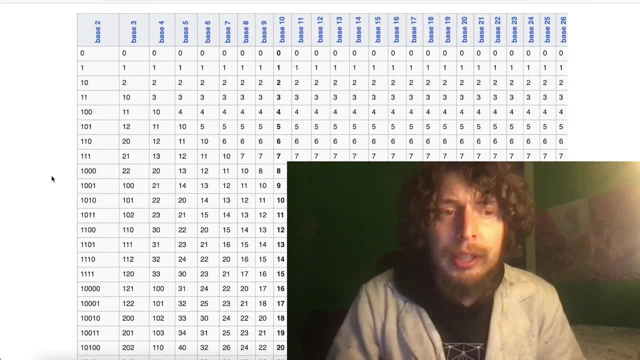 description here. the Pandigitals actually in a way have a certain type of extra importance that these others don't have in terms of how sort of fundamental they are on the number line of any base. So the Pandigitals, I've learned, have extra rare, you know, a large presence but all of those are 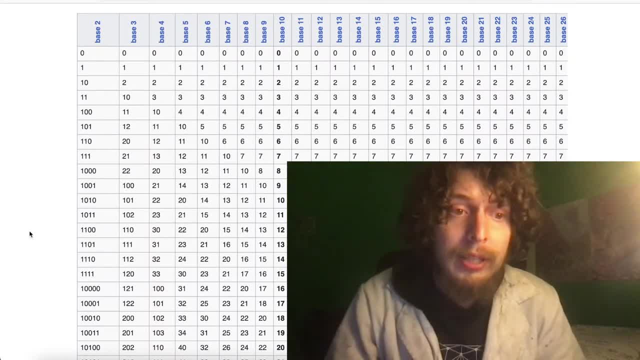 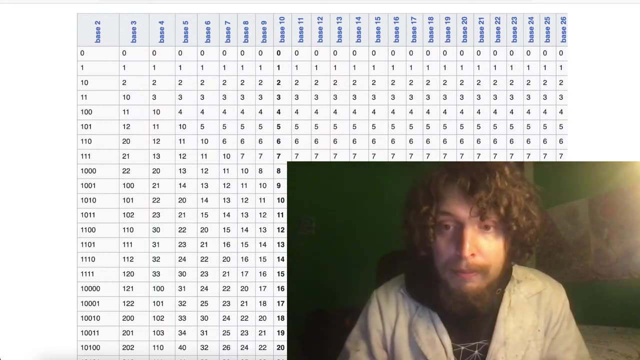 fun types of numbers that will come back in future episodes. You also could investigate palindromic numbers, which numbers are palindromic in different bases or look mirrored like 121 or 12321 or 52125 or whatever. So those are fun as well. And now I'm going to take a little peek at the comments before. 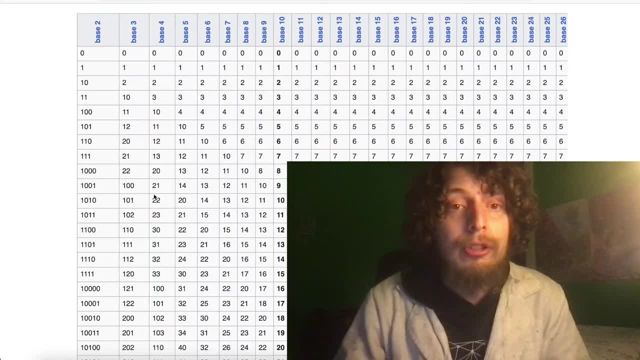 we switch over to another idea. Instead of looking at number traits that line up with different bases, we're going to look at particular number. Well, actually it's going to be another number trait first, but it's going to lead to a few numbers. 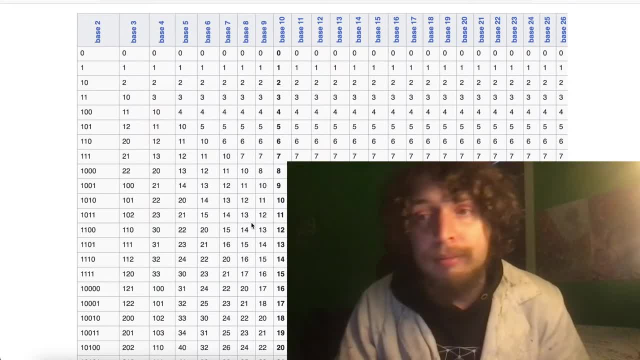 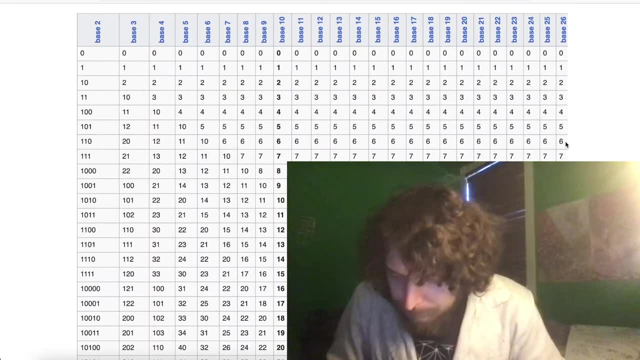 So let's take a look at the numbers that have a special property in every base. So thank you all for joining me here. People wonder what's this math for? Well, it's for you never know. It's for setting up in the 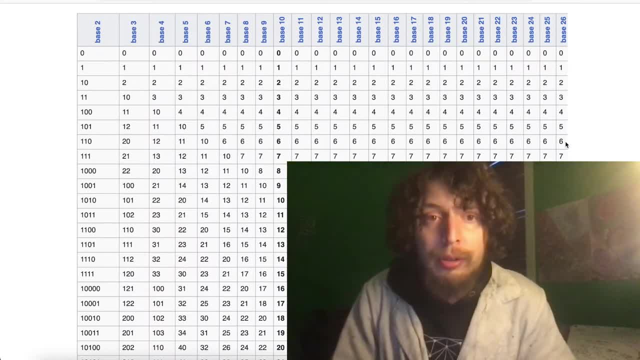 future of mathematics and thinking in general. you need to think outside of the box of the system you're in, And so this is thinking of how numbers would be written in other ways Of counting and which properties maintain, And I think that's very important. It's a recurring 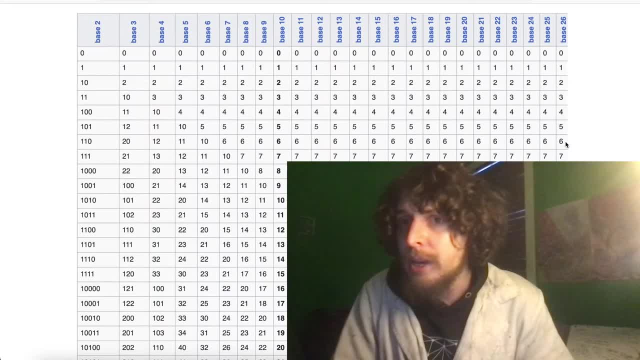 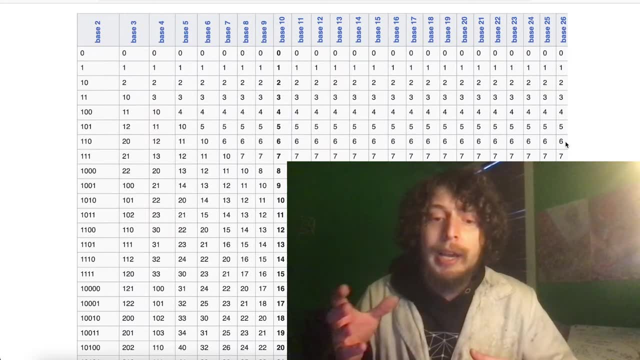 theme on our class different bases because, like I said, you know, if we're both like thinking of surreal variations to our current system, that could actually be better, and we like numbers. this is sort of on the mid ground between that. So these are all interesting patterns And 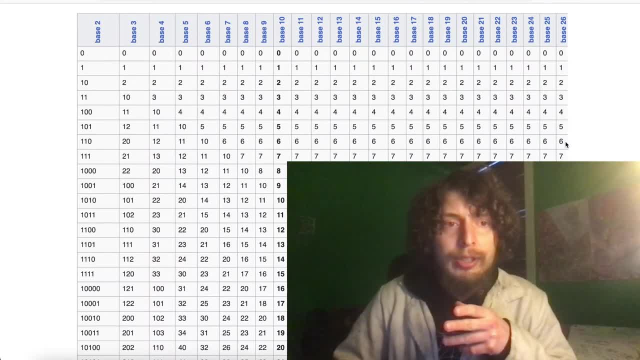 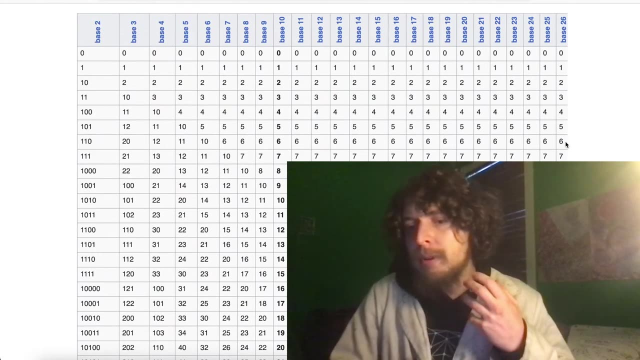 another pattern we could ask that starts out quite base dependent as well would be related to sums of digits. What happens when you add up the digits in a number, For example, we could note that in our base, if the digits in a number add up to a multiple of nine, the original number was a multiple of 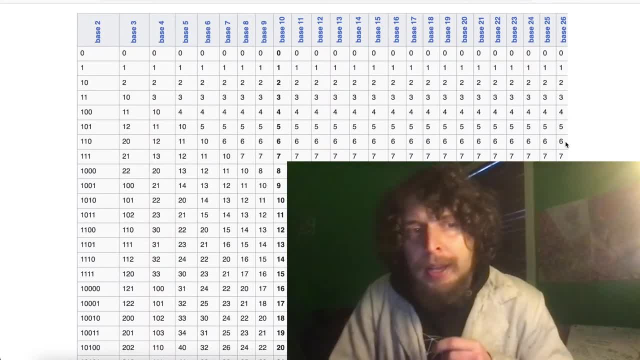 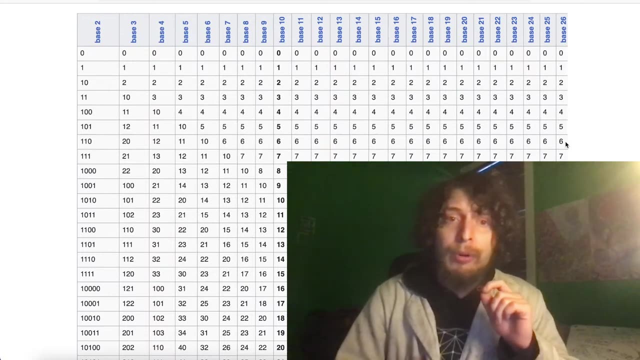 And you get a similar property for 3.. If the digits in a number add up to something threven a multiple of 3, the number itself is threven. Now, is that because base 10 is magical? No, that's because 9 is the number, 1 less than the base number, and 3 is a factor of that. 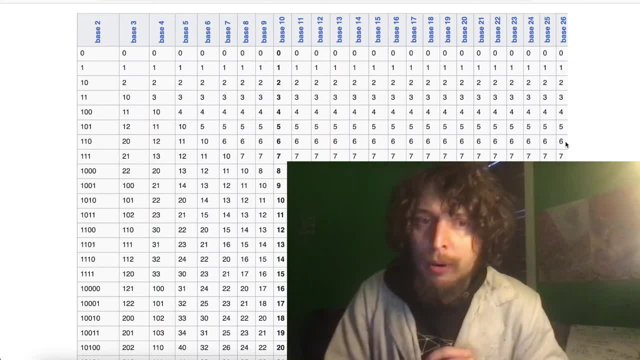 And so it turns out you get similar powers in other bases for the number 1 less than the base number and potentially for factors of that number, And you do get a superpower for the base number itself, which is it's the one that generates zeros at the end of stuff and is extra easy to spot multiples of. 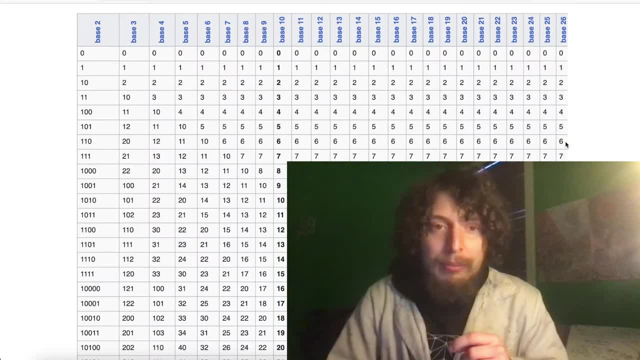 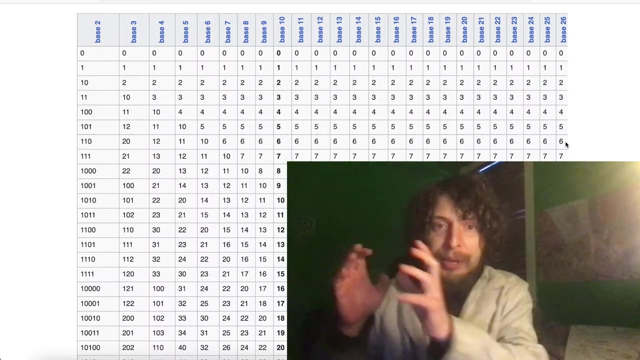 And other superpowers, like the factors of the base number will have the easy trait that evens. So a lot of divisibility traits will be these pure things that are true in any of these bases, as long as you adjust your caliber from talking about 9 and 10 to talking about b-1 and b for one of these. 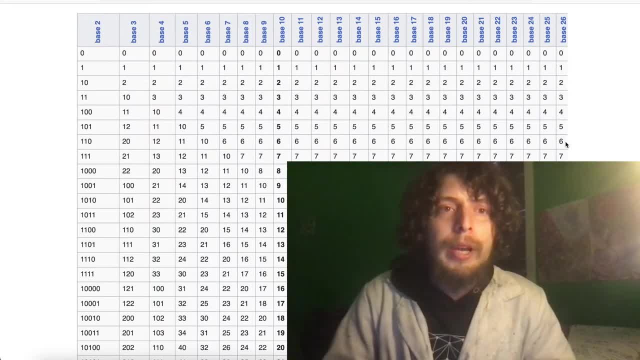 Also, as a quick clarification, we are starting on base 2 on this chart. That's where they started it, like I would have, Although many people often mention base 1, and when people mention base 1, they often use the digit 1, and we have to note that that wouldn't be following the same rules as this. 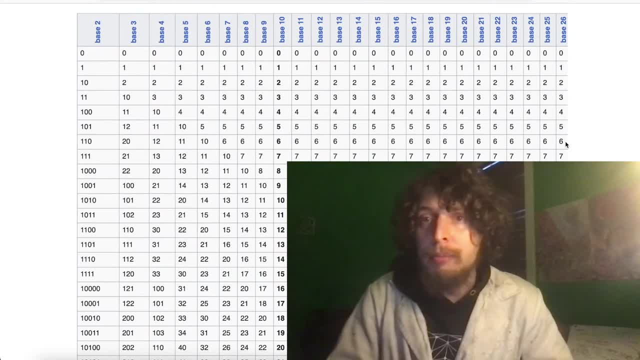 All of these bases are using a digit symbol for the numbers between 0 and 1 less than the base number. or in other words, they're using the base number's amount of digits, but including 0. And the base number itself is the reset. So if you made a base 1, that tried to match this. it would be only using the digit 0, and it wouldn't actually be able to express different things. Also, if your spots in a number are powers of 1, then they don't have different amounts than each other, and you could have stuck your digit wherever, whichever place you want, and it still should have just meant a power of 1.. 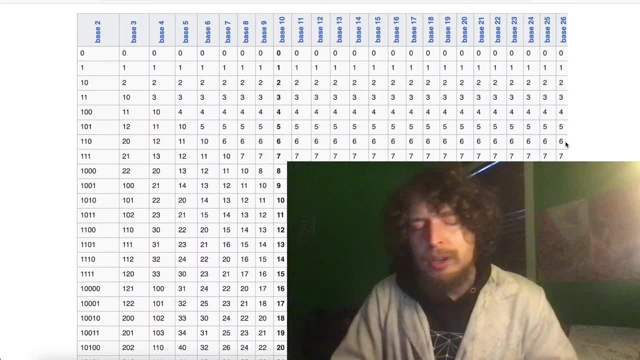 And so tally marks are not actually the same type of base. 1. that binary is base 2, you'd have to add some extra words in your name to say that you're using a different type of base. you can make something like that with other things called bijective bases or stuff. 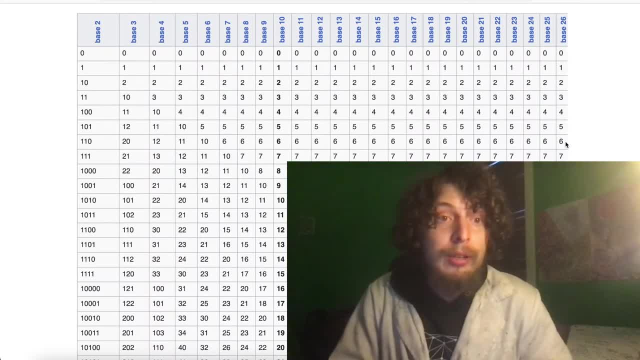 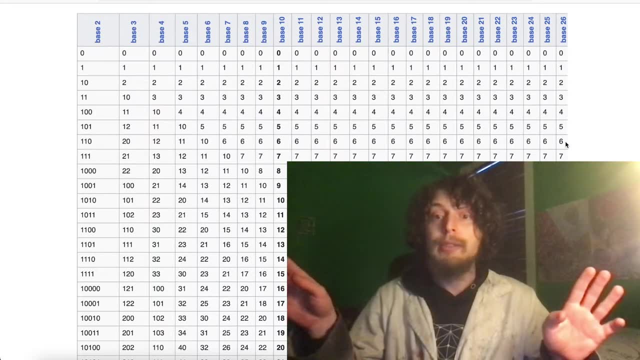 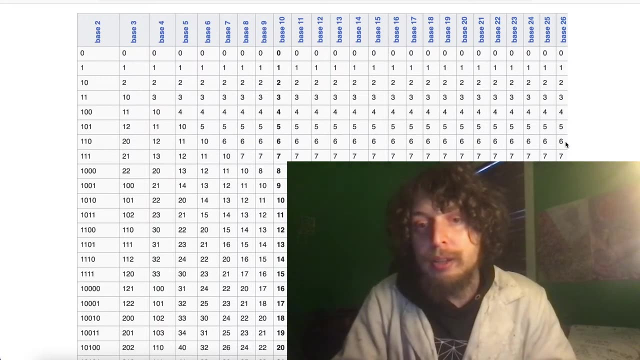 but if we're talking about these typical bases, following at least the rule that you're including a zero and your amount of symbols are your base number, no base ones in the house. base two is where it starts and that's why in some of the traits in the pan digital episode i was like extra. 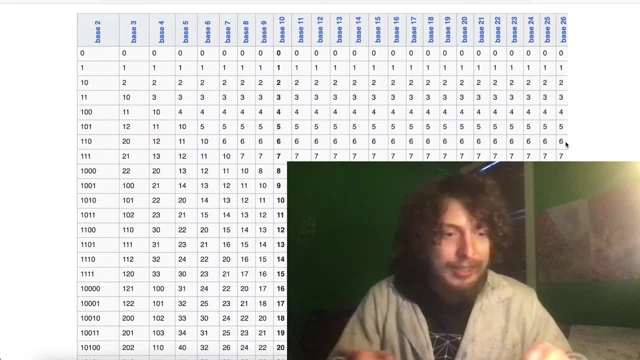 emphasized- for all positional base or for all regular bases: two and higher, integer bases: two and higher, because i've talked about a lot of weird bases on my channels and some of those may have the same traits as the traits i mentioned, but there were parts of the episode where i was 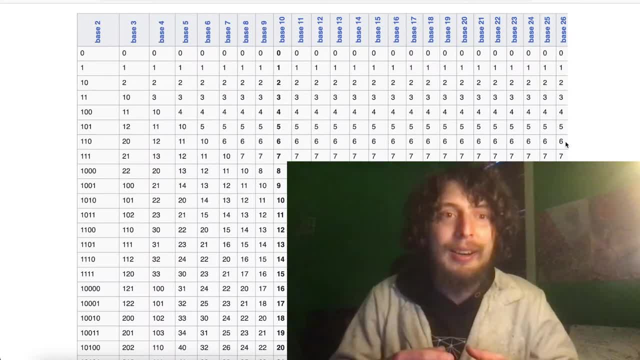 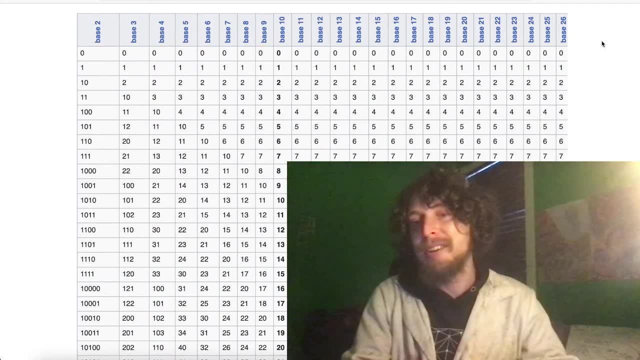 like this applies to all bases, and so i had to be clear by all you. i mean, you know, i've confirmed it applies to all of these bases and the further numbers that are integers two or greater. so these are the first realm of our extension of what a base could be. 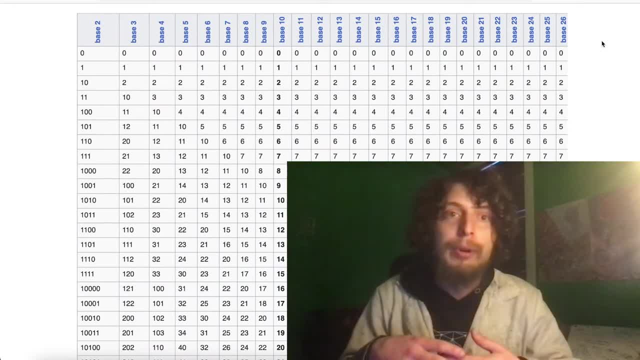 then you can go outside integers, outside positive numbers, outside various ways, like we've done in episodes on my main channel, and you also could completely abandon the idea of being a positional base with powers of a base number. but but even within that realm we can see there's a lot of cool patterns. 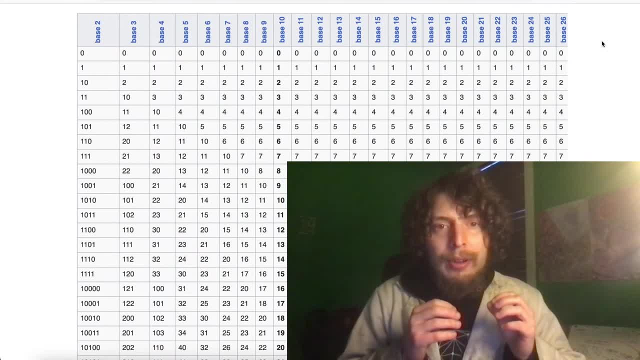 so the next thing we're going to ask about digit sums is going to be which numbers are divisible by the sum of their digits? now, we said that the multiples of nine were in our base. um, actually no, that's not true, because we said that the multiples of nine were in our base. 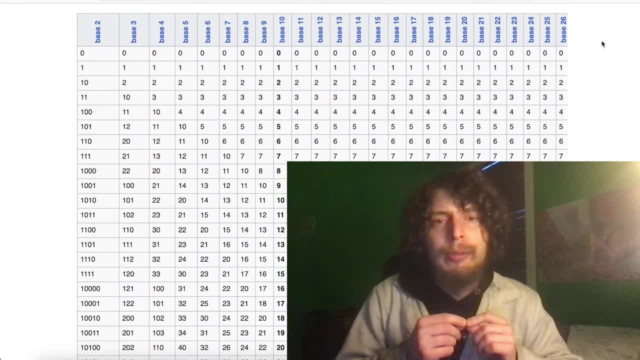 and that's not necessarily true, because, although the multiples of nine have a digit sum that is a multiple of nine, you could have a number that couldn't divide the specific larger than nine multiple of nine. that was its digit sum if we asked you if they could. 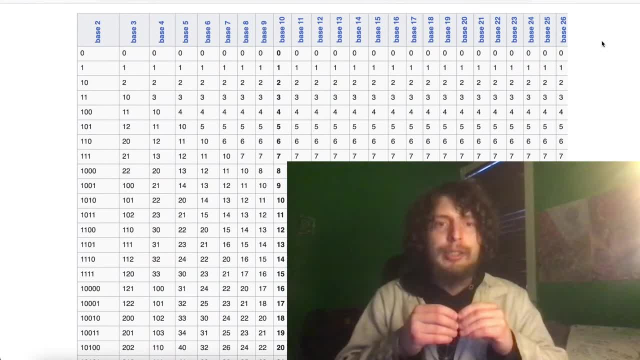 divide the digital root, which is taking the digit sum down to a single number, then any number could to divide the digital root. your multiple of three can divide their digital root, a multiple of nine can divide their digital route, but we're talking about digit sums, which numbers are divisible by the sum of their digits. 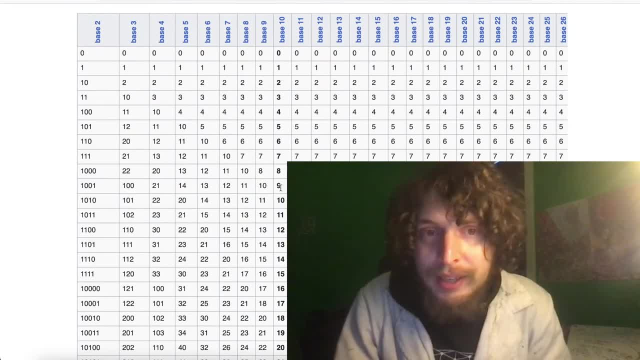 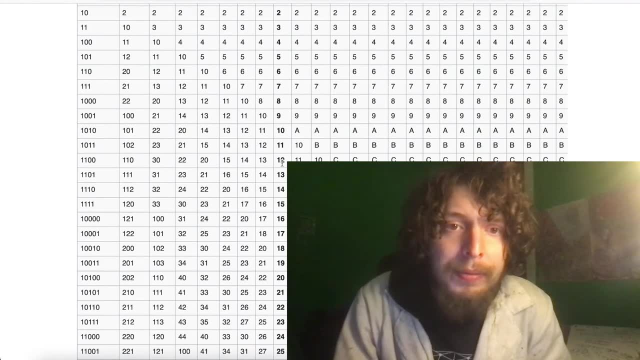 now, on a trivial sense, we're going to say one digit numbers can do that, they can divide themselves. going forward, we can see in our base: 10 is divisible by 1,. 11 is not divisible by 2,. 12 is divisible by 3. 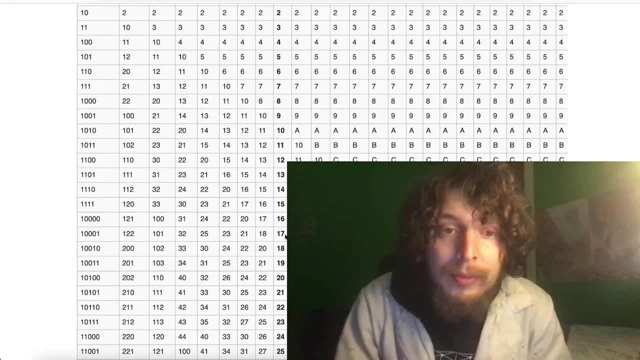 few are not divisible by their sum. And we get: 18 is divisible by 9.. That one, 20, is divisible by 2.. 21 is divisible by 3.. And so, which ones are divisible by their digit sum? Well, there's a. 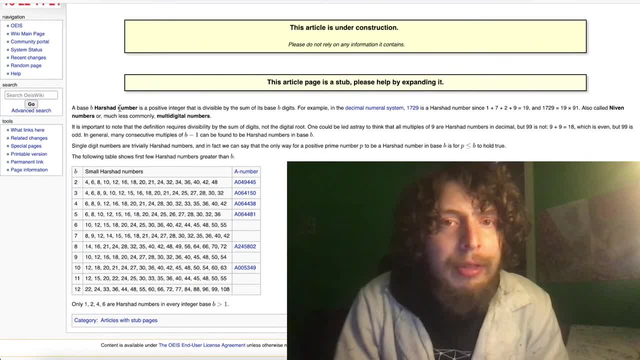 name for that. It's often called Harshad numbers. It actually has other numbers as well, But here's some other names for it. Like many things in math, they got a bunch of numbers. We'll call them Harshad numbers for now, And here they're noting. they say that this article is under. 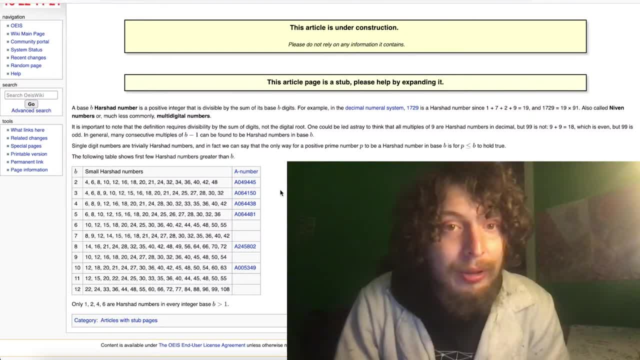 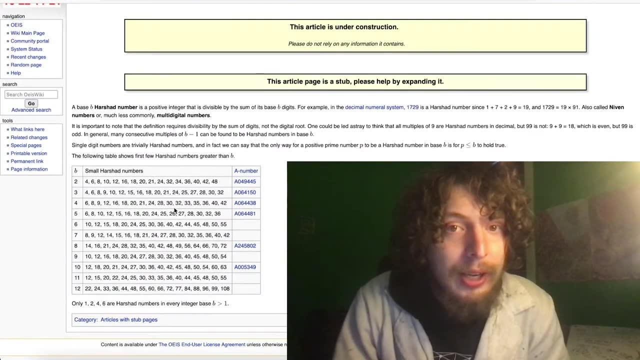 construction don't rely on the info. But I read through this real quick and it seems that valid Now going through here. I really love this site, the OEIS, So I'm trusting them, even though they say they're under construction. Luckily there's also a. 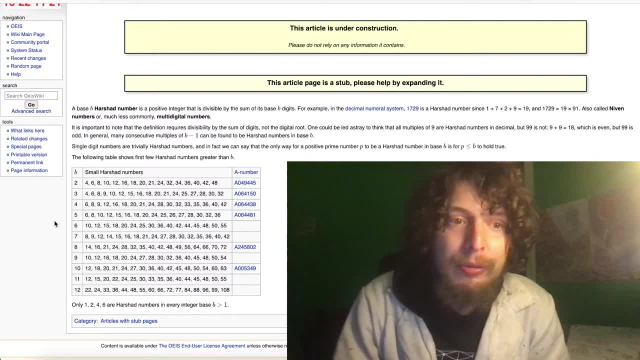 trait, So we can sort of verify ourself on an individual number scale. we can see that we can test them. Now it looks like maybe these are actually. are these written in the base or written in base 10? That's not super clear, which we could look into that. But looking here on our table, 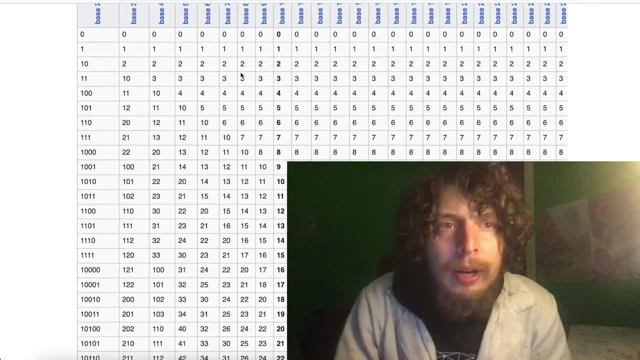 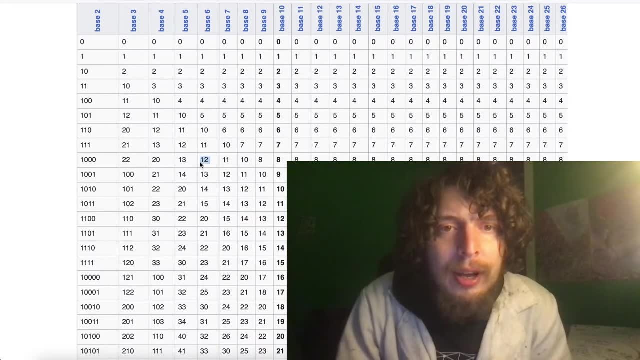 we can see that if we were in another base, let's say base 6,, well, this number represents eight of a thing, And we're just using base 10 as our reference because that'll help us understand it. And it's not divisible by three, This number 10, of a thing. 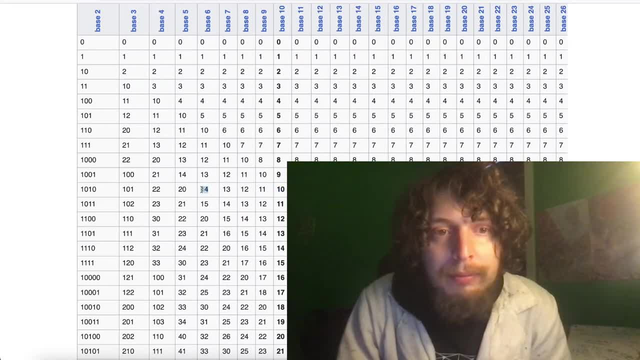 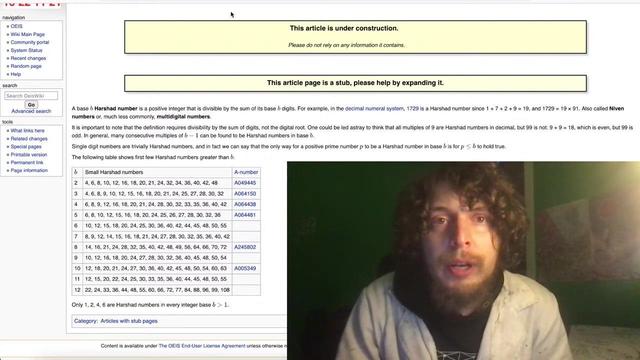 is divisible by one plus four, four. So we get some interesting. and of course six is divisible by one plus O. the one-digit ones are divisible by themselves and stuff in the base. But which numbers have that property? Well, let's see. also on. Wikipedia has a bunch of information about this And 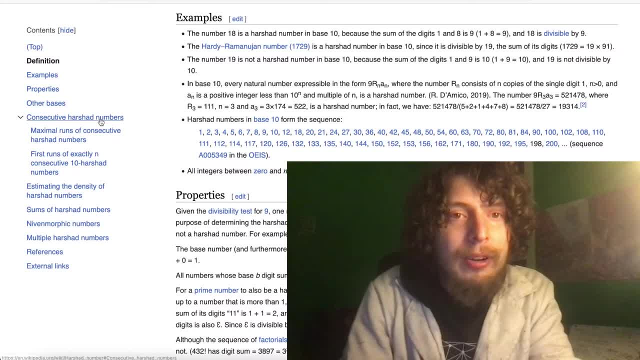 and of course, Wikipedia pretty much always could have that warning. This is under construction. don't fully trust this, but they're pretty good for math actually, And you know they're not flawless. Don't quote them in your paper, but they give you the seed of the info So you're able to 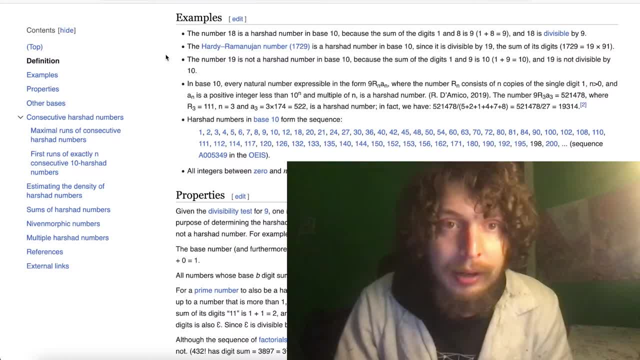 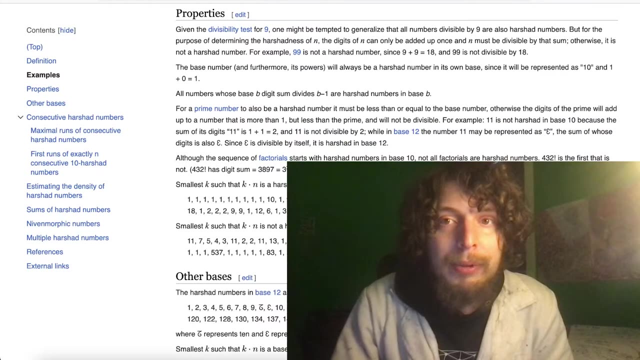 know some fun stuff to look up and research or try out later. So here's, for example, the list of ones in base 10.. Now there's a random example here. they're noting an example of what I said that you might be tempted to generalize that all 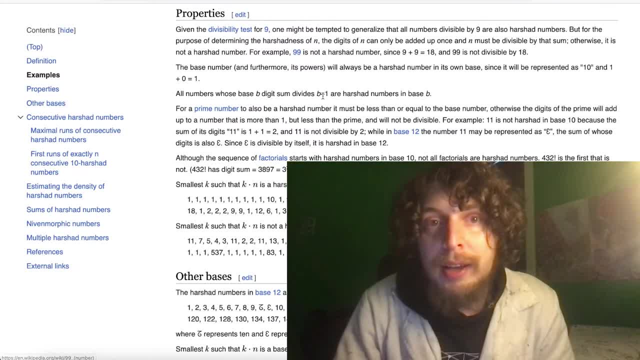 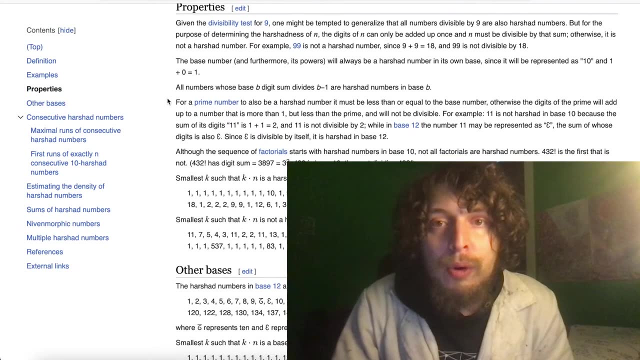 numbers divisible by nine have this property, but 99 is a multiple of nine, but it's not divisible by the sum of its digits 18.. It would be divisible by the root of the digits if we added it down to one digit. And so here's one I mentioned in a short. that's super trippy Factorials, look like. 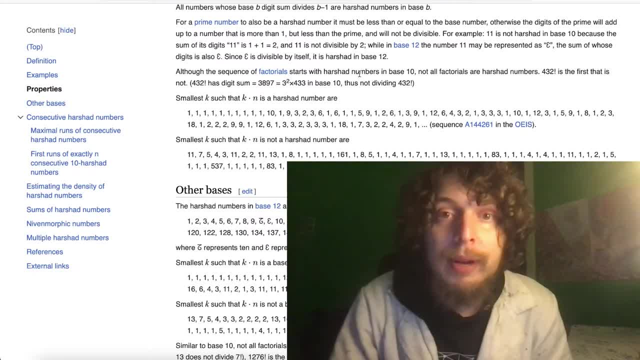 they all do this. They're not divisible by the sum of its digits. They're not divisible by the sum of its digits. They look like all factorials are divisible by the sum of their digits in our base, but not all factorials do that. 432 factorial doesn't And, as I mentioned in my 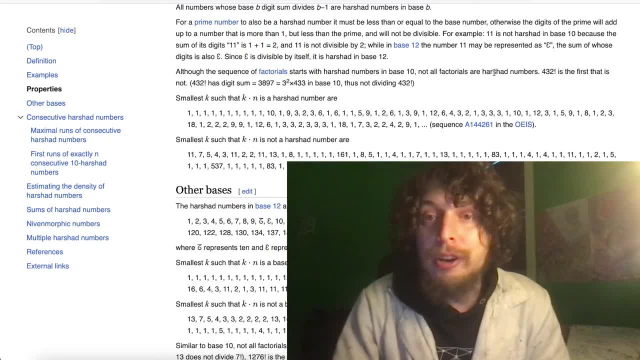 episode about factorials on my main channel that made me look up a list that I put in there of what's the first factorial that breaks the pattern in different bases, And it turns out that some bases have a lowish factorial that isn't divisible by its digit sum and other ones 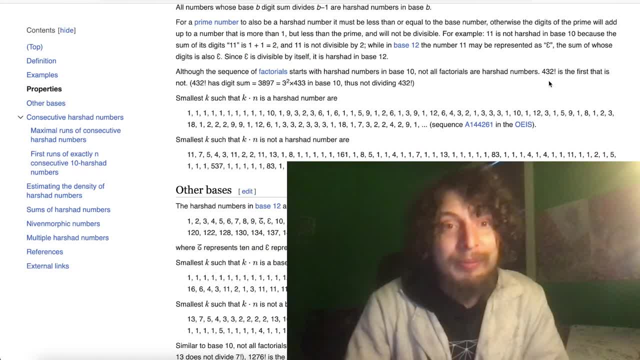 that are divisible by the sum of its digits, And so I'm going to look up a list of the numbers that are divisible by the sum of its digits. This one has a prime factorization of 3 squared times 433.. 432 could obviously divide the 3 squared part of it, but can't divide 433.. 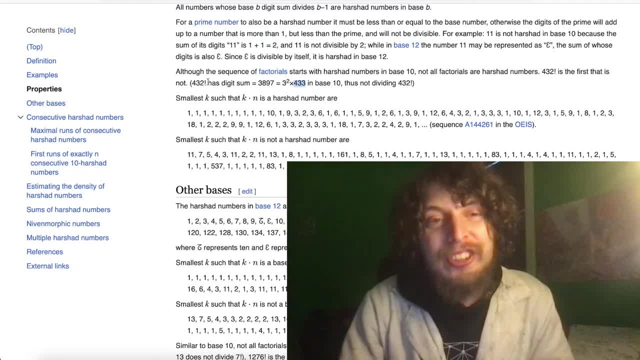 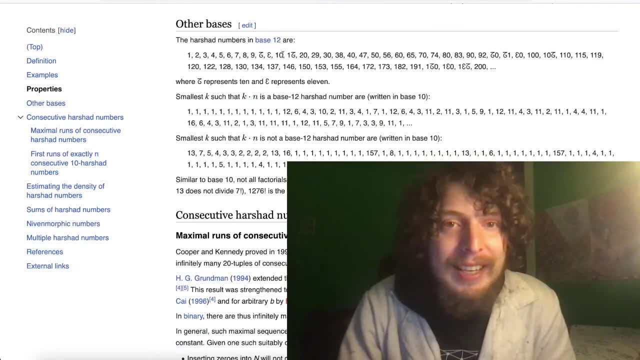 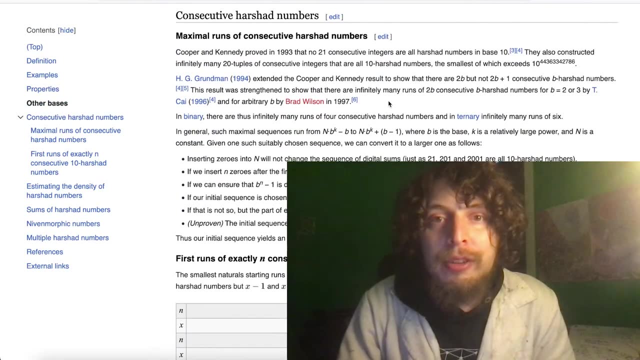 It's one number too big for the factorial, It just misses. so they also note some other things like here's some base 12 ones and stuff, and here's an interesting one that i also made a short about a while ago: you cannot have 21 consecutive integers. 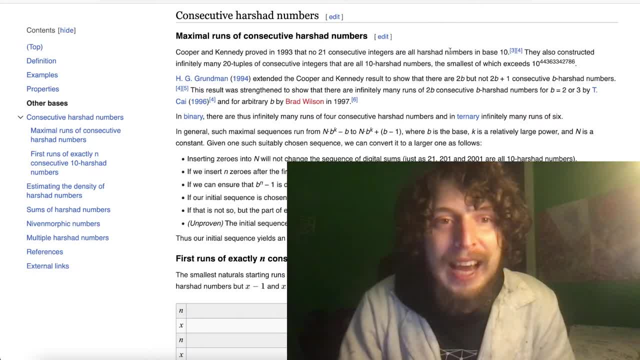 in our base that are that all do that you need in any string of numbers in the base to um, eventually you're going to hit one that's not divisible by the sum of its digits in our base and here's like the first run of a bunch of them. here's estimating something called the 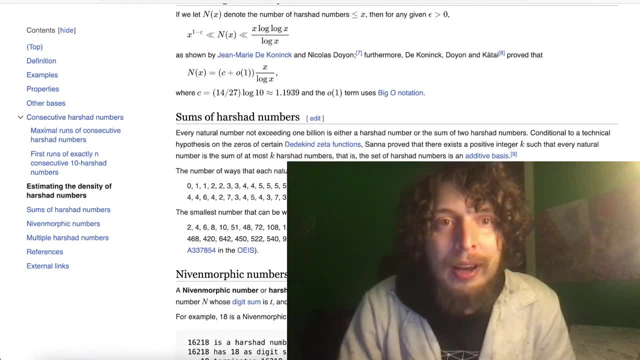 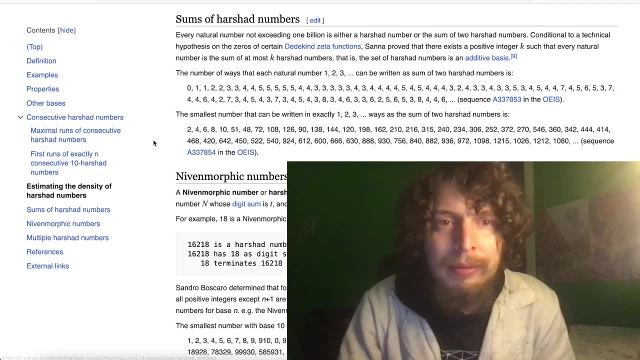 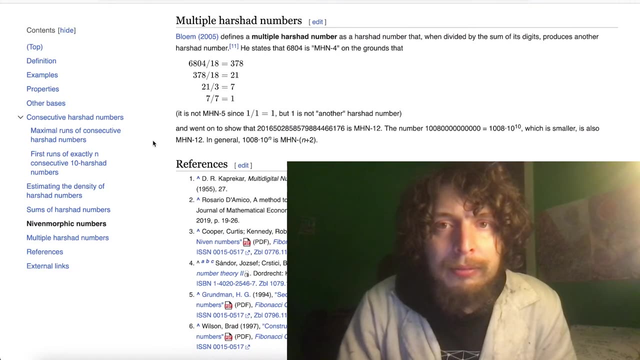 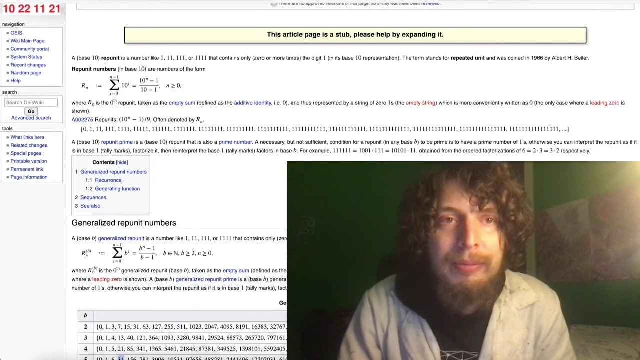 natural density. that was mentioned in my new episode. um, if they're talking about natural density, i have to read that. uh, because there's a few types of density and various fun facts. um, now an interesting one on here. that is true, don't worry about the under construction part of their 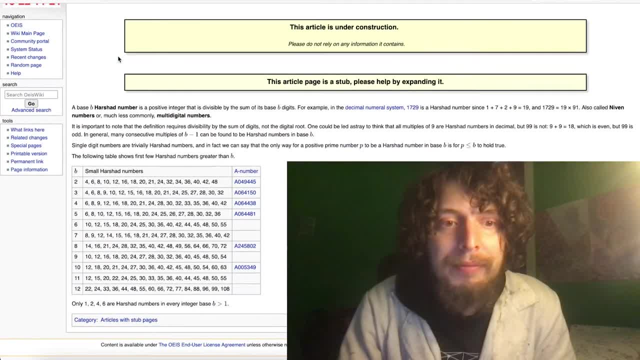 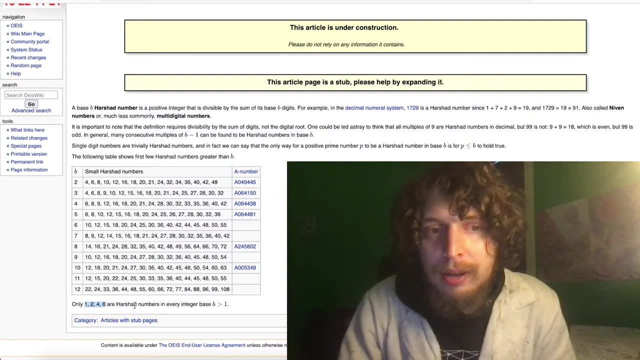 page here. an interesting fact here is something says only one, two, four and six are harshod numbers in every integer base greater than one, and i've seen these called all harshod, like all slash harshod numbers or dash or whatever something. uh, and that means that they're this harshod number divisible by 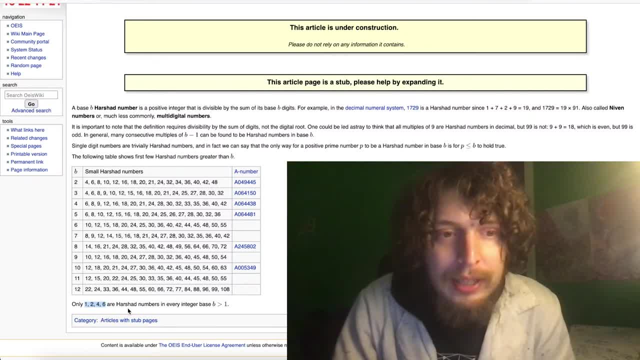 their digit sum when written in any base. now that sounds crazy to be like any base out of the infinite possible amount of these, but- and as usual they're saying integer base greater than one. like i was clarifying for my stuff when you look at a number, if i was wondering if 10 can have this, 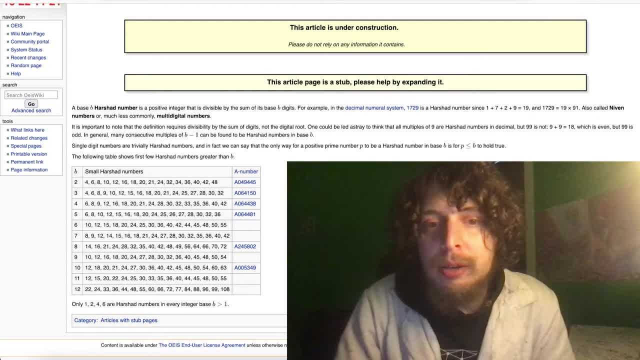 property. well, well, 10 is gonna be written with a single digit symbol, base 11 and upward, and that single digit symbol, in a trivial way, is divisible by the sum of its digits, which is itself. so, as soon as you get up to past the base number, 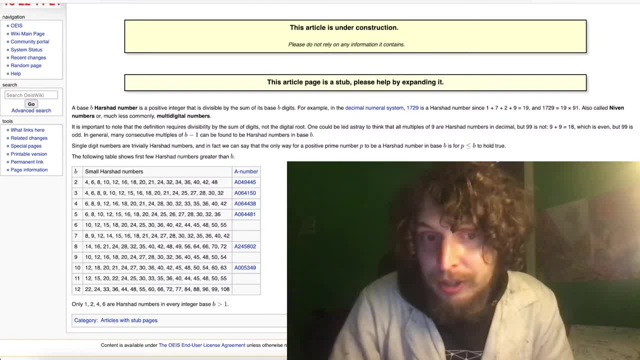 then you're good to go, even the base number. you're good to go because it, the base number, will be written one oh one zero in its own base. probably that's gonna be fine, but i'm not sure that's gonna exactly how this thing is addressed. right now. i could be drawing, i could try some golf again, i think. that would just be about ten out of ten dialed on a globe, or someone will probably pick it up about 10 size encouraged or something there. we'll cut that part out of the video and instead i'll take that separate. but but we're going to stop there and make sure that. the fact is that if we're expecting slice numbers and 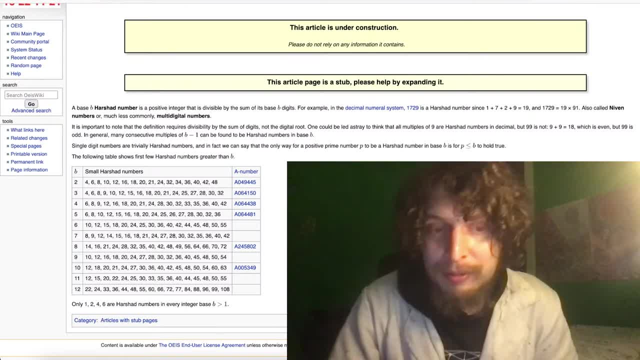 and that adds to one and it'll be divisible by one. and then in further bases it'll be a single digit symbol that will be divisible by itself. so to have this property, you'd only need to be divisible by your digit sum in all the bases smaller than you. but 10 isn't. if we look at 10, it's divisible by 1. it's. 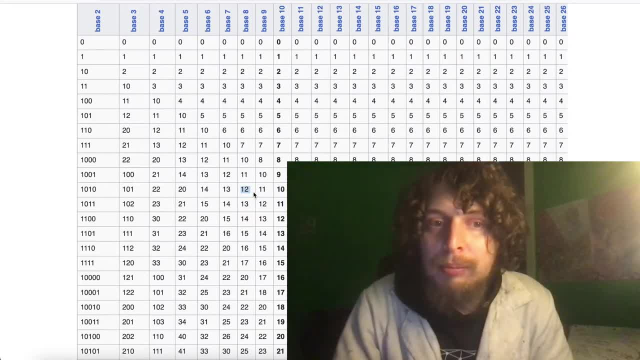 divisible by 1 plus 1, but it's not divisible by 1 plus 2, so it's not going to work and we're gonna see a lot of these are gonna have trouble doing that. however, if you look at one very trivially, has that property to in a. 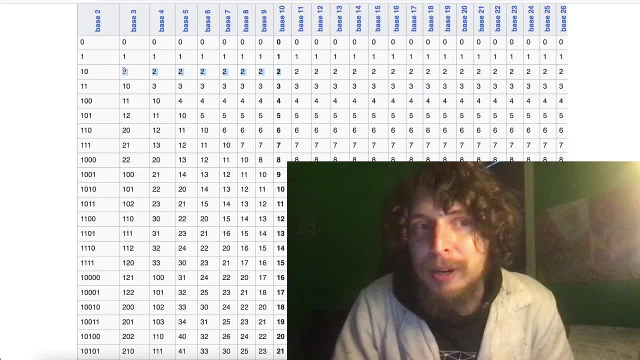 pretty trivial way as the property it's to and all of the other bases, except for here. it's one zero which adds to 1 plus 0 is 1. it's divisible by that. three in a slightly, or no three doesn't do it. one one. they're not divisible by two, but four. 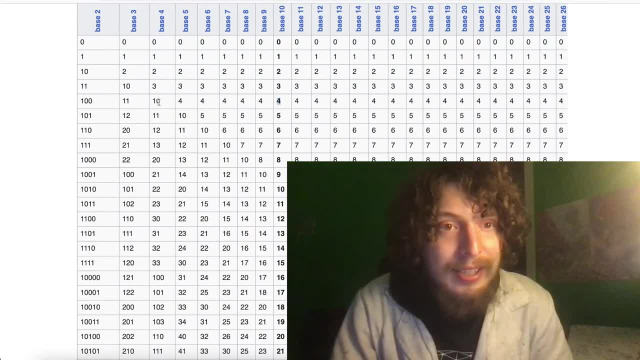 doesn't do it in a slightly less trivial way, because we have it's divisible by one plus zero plus zero, and one plus one and one plus zero, and there it is itself. so it's divisible on all the ones leading up to it, and now it turns out there's only one other number in the universe. it's been proven. 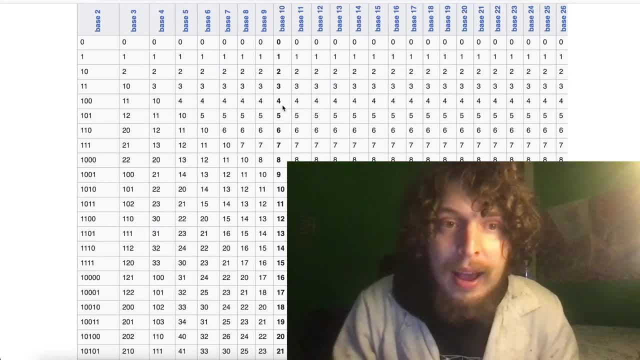 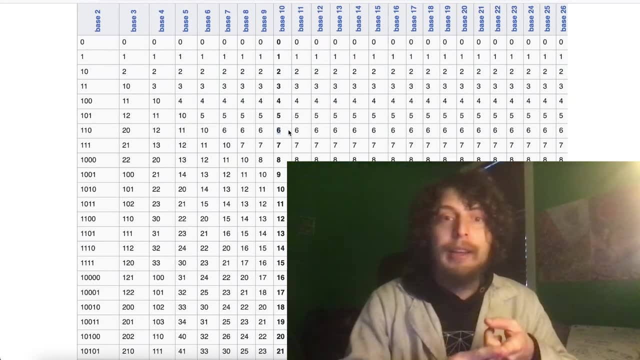 that does that, apart from one, two and four, and it is our magical number six. not only is six a triangular number, and not only is six the only triangular number, that is also a factorial, apart from one. not only is it the only triangular number. this is a fact, and you still need to look. 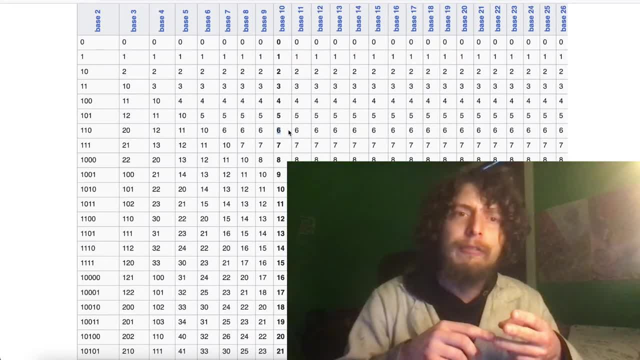 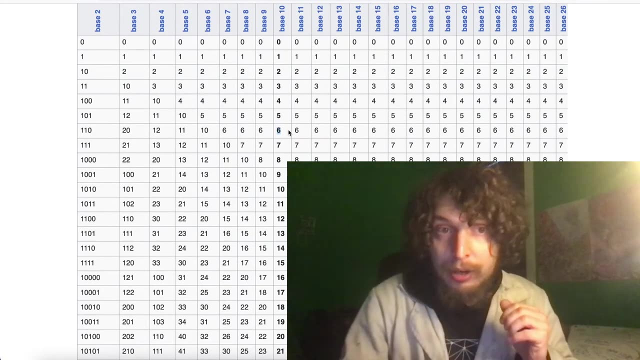 up the proof for, but i read this once, so i believe it's the only factor or the only triangular number. who square is a different triangular number. it's a perfect number. in fact, it's the smallest number known as a perfect number, because the smallest number who? 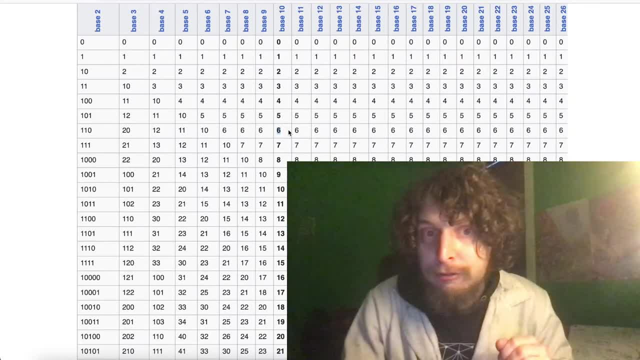 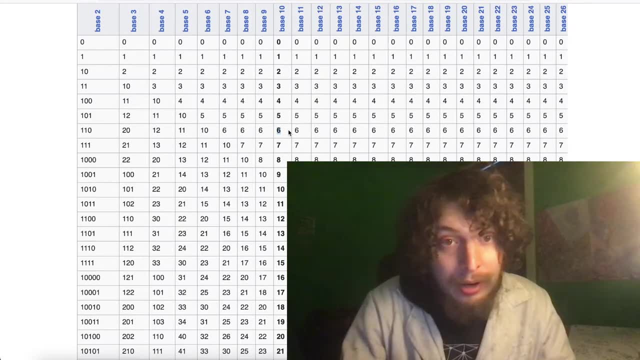 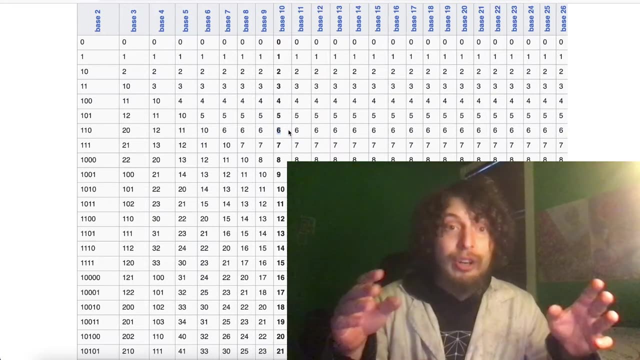 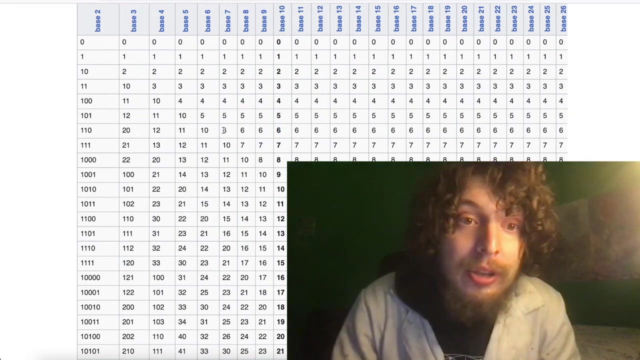 all of its divisors, apart from itself, add up to exactly itself. it is so many other names of property. it is a superior, highly composite number and many cool titles. well, it turns out it's also the largest all Harshad number, the largest number divisible by its digit sum in every integer base, 2 or greater and once. 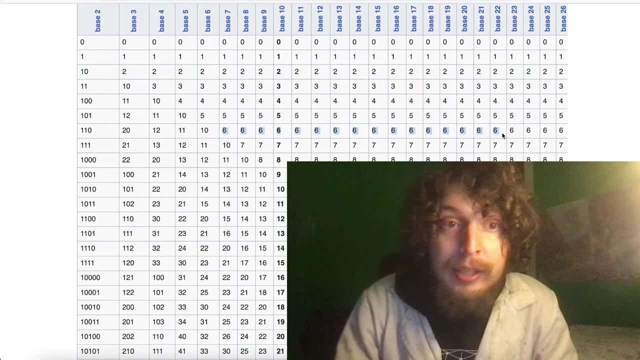 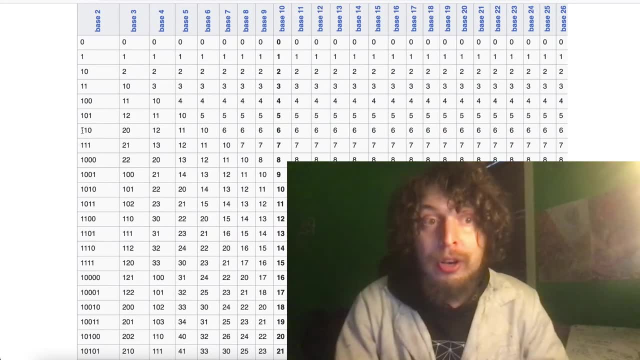 you get up to the single digits. we know it'll pass, but we and we know that 1 plus 0 will pass on the base number. but it has to get 2 through 5 correct and it does. 1 plus 1, 2. it's divisible by that: 2. it's divisible by that 1 plus 2 is 3 it's. 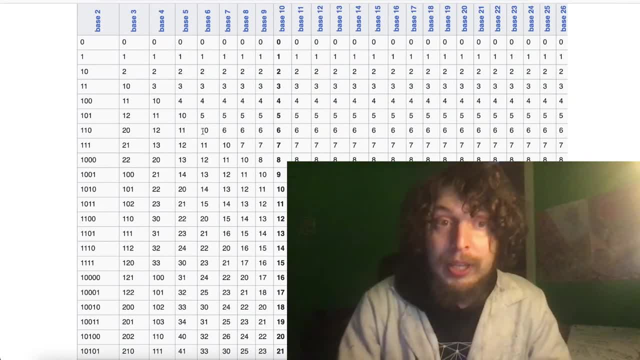 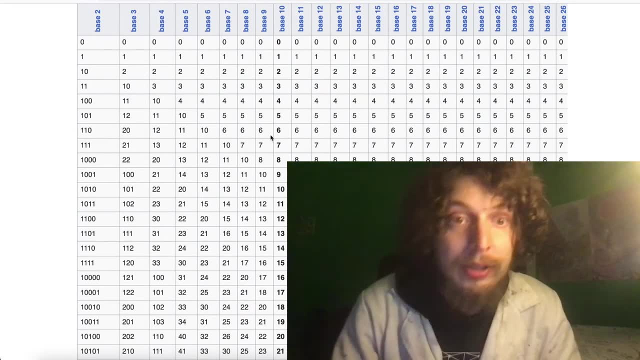 divisible by that, 1 plus 1 is 2. it's divisible by that, 1 plus 0, and we're good to go. so 6 is the largest all Harshad number, because it's actually been proven that no larger numbers are going to be able to do that. so that's. 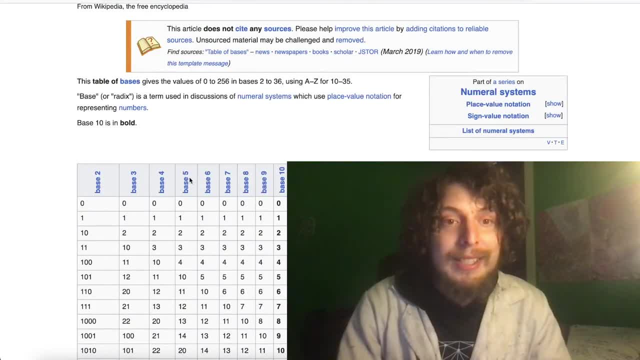 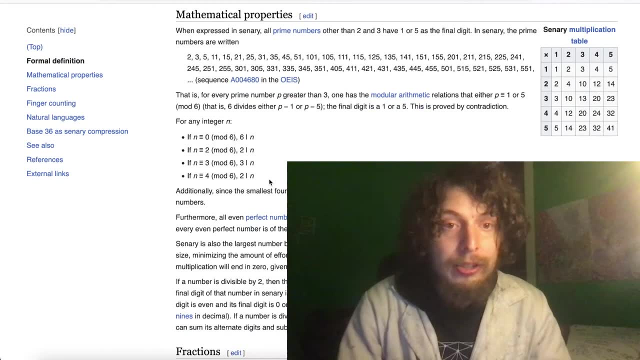 another property of our majestic, number 6. base 6 here also has a large number 6. base 6 here also has a large number 6. base 6 here also has a lot of amazing stuff. we'll cover next grade. in grade negative 1 we did a lot of. 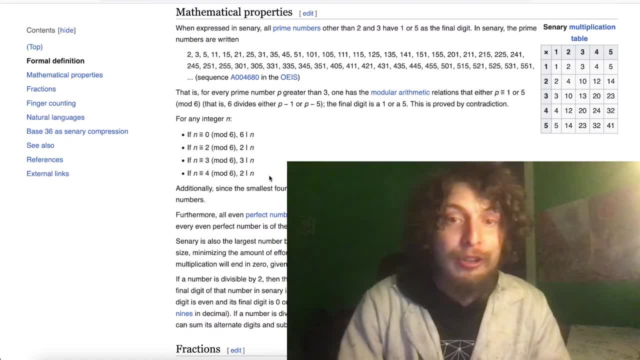 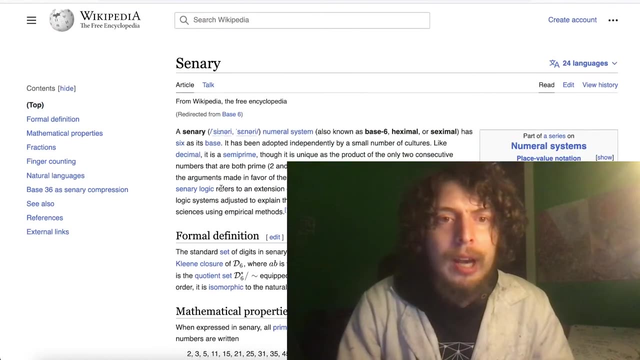 episodes about crazy bases. so in grade negative 2 we'll have at least a few bases or a few episodes about more practical bases, such as base 6, such as balanced ternary and some other ones. so I just want to get to the number 6, the 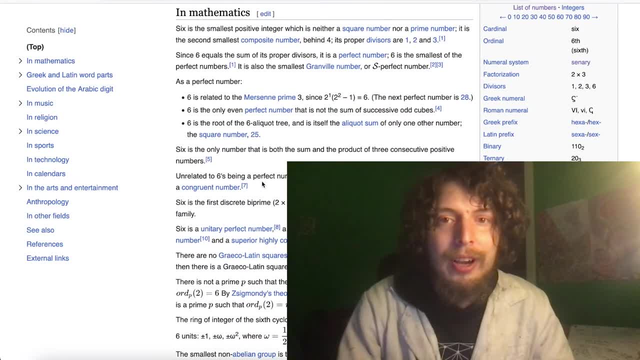 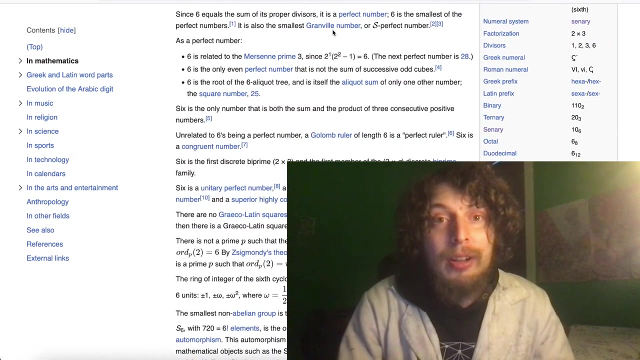 number 6, just to see a list of more of the stuff it is so it's perfect number related to the mercent. it is the only even perfect number with that property. it is the root of this. get through this step thing called malakwat tree. there it is something called a perfect ruler in. 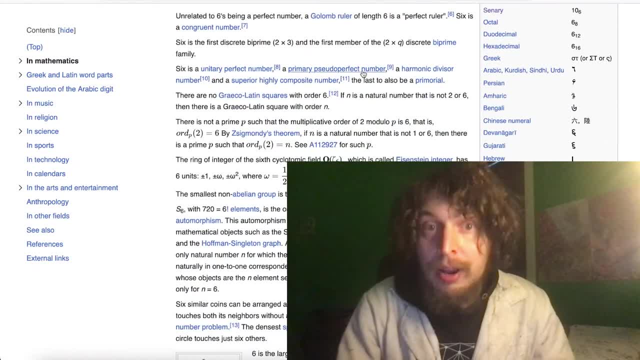 addition, separately to it being a perfect number, it is a congruent number. it is the smallest, what's called a granville number. it is a unitary perfect. it is a unitary perfect number, a primary pseudo perfect number, a harmonic divisor. it is a unitary perfect number, a primary pseudo perfect number, a harmonic divisor. 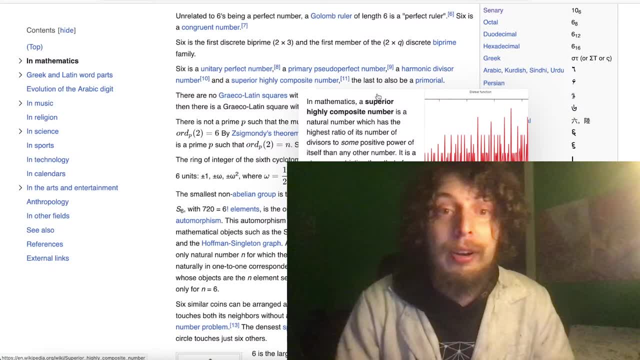 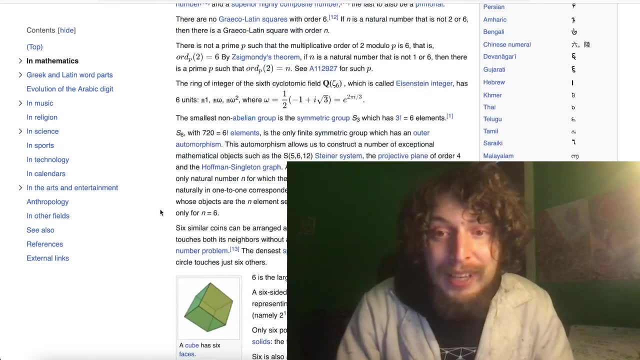 number and when you look at the roots, hold exactly what you got, showing us all and the last superior, highly composite number to be also a primordial. So and here we go: the largest of the four Al-Harshad numbers, And it's the amount of faces. 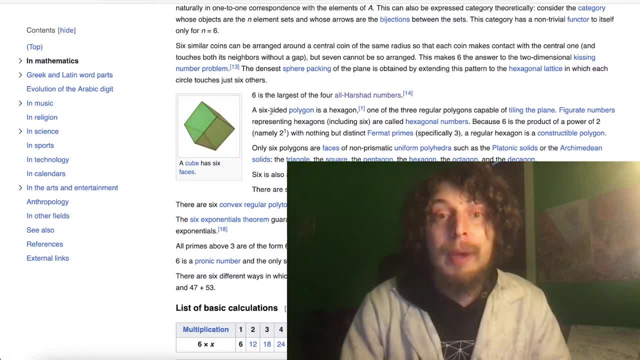 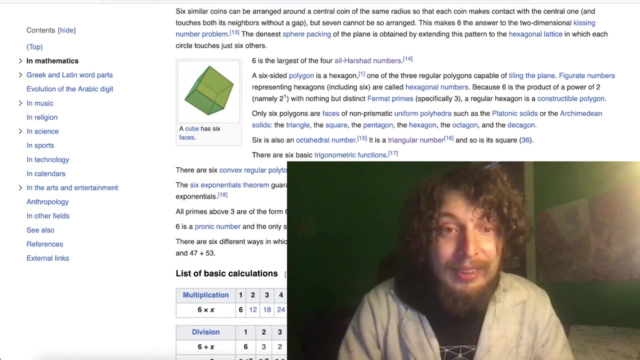 on one of the platonic solid shapes. It is the amount of edges on one of the 2D shapes, one of the only three shapes that can tile the plane. It also happens to be an octahedral number. Every prime is one, apart from the numbers two and three. 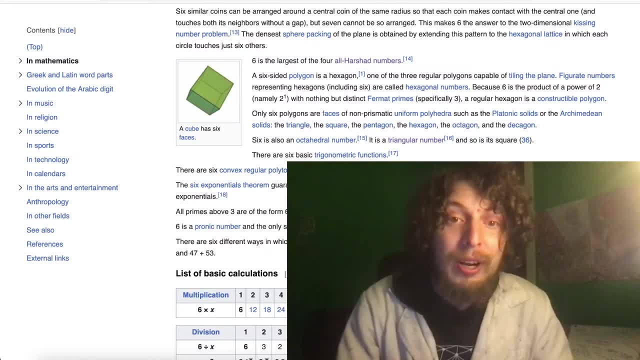 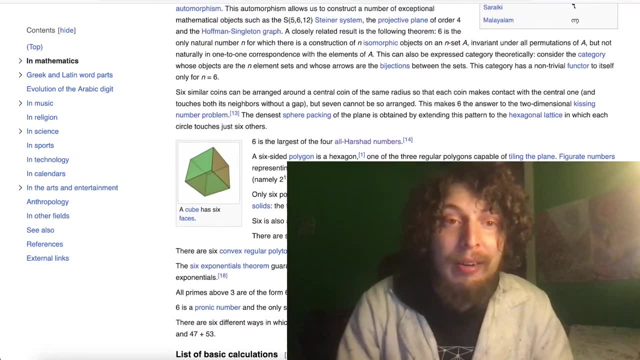 which are its factors are. one is one less or one greater than a multiple of six. It is what we call a pranic number, which is sort of like an almost square number in a way. It is so much stuff So I have learned throughout this grade. 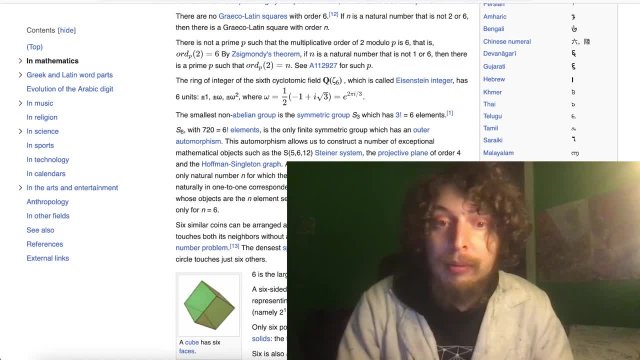 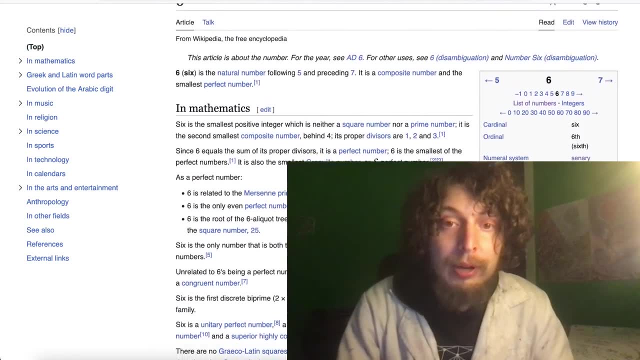 I didn't even know it as much as I know now at the beginning of the grade, but now I know six is the most underrated number and we'll probably continue to see it, as well as multiples of it. So back to our base chart. 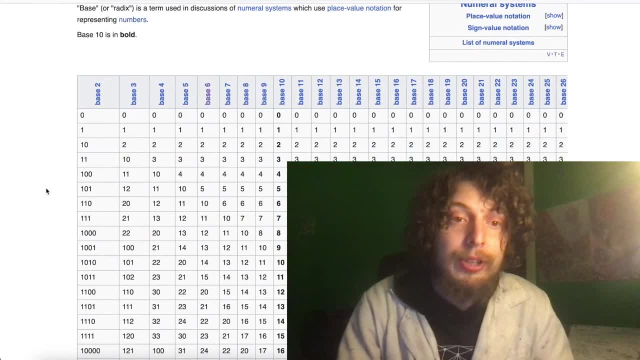 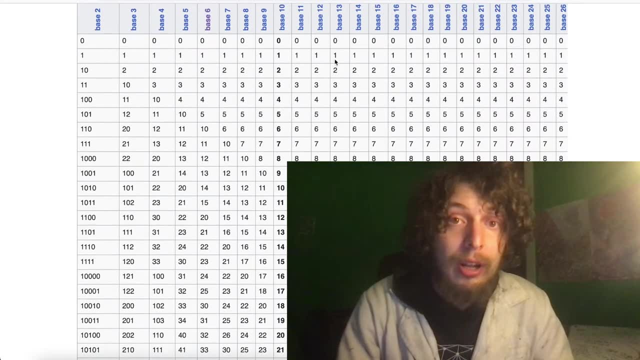 we can note if we can ever convert to base six, which is extra neat, And for all the base 10 fan, I mean for all the base 12 fans out there, base six actually does all of your good stuff in a neater way. 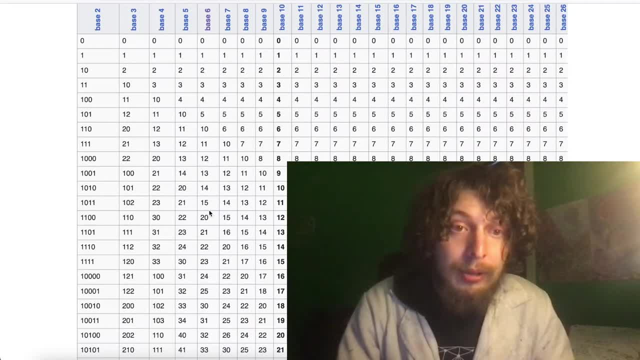 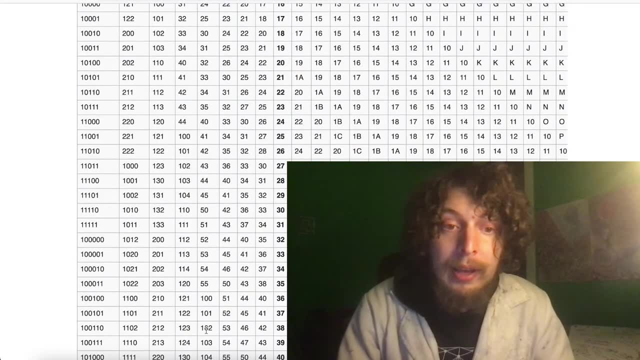 So we can see that we only get the digits one through five, and here it just looks like they're climbing up there because that's how they're going to look there. But when we see multiplication tables and fraction tables we can see how superior it is. 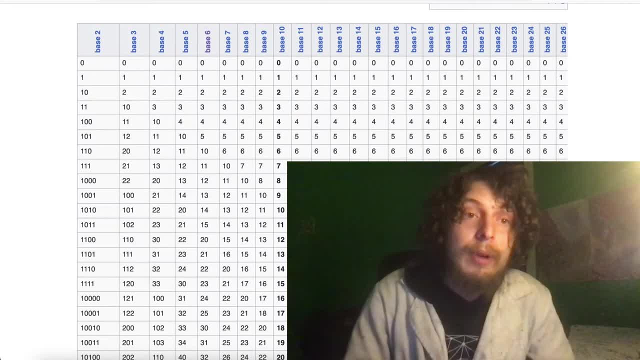 So that's a pretty fun one. which numbers are divisible by their digits? Of course, we could ask other questions. which numbers are divisible by their product of their digits? Which numbers is their product of their digits equal to the sum of their digits? 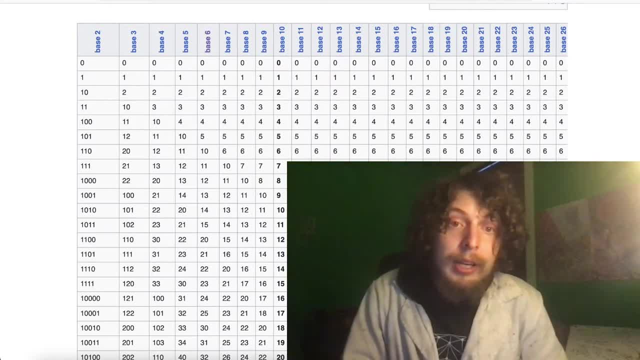 which would be verging on another interesting question we might cover later. We could ask all sorts of questions that might relate to having to be dependent on a base, And the key word there is that we are doing something with the digits. But even when we are stuck in a base, 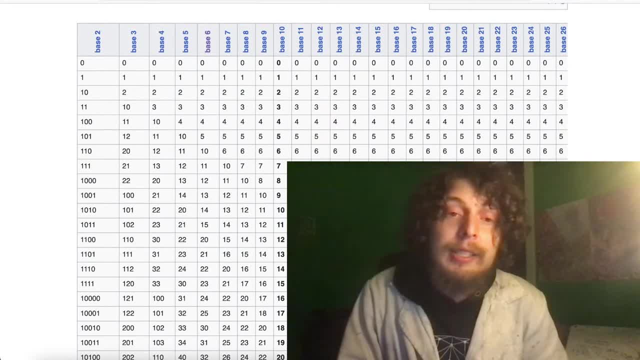 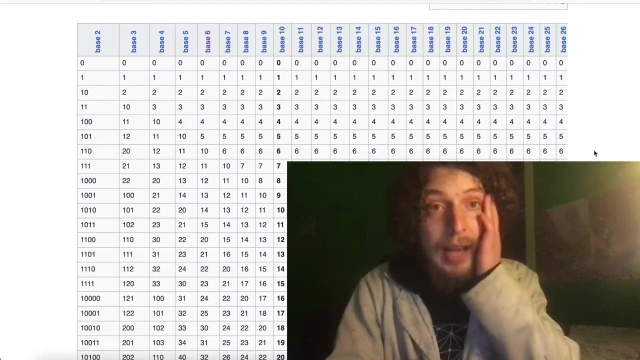 and we see a trait like that, it might be a seed of a clue, of a pattern that would exist on a whole infinite amount of possible ways of counting numbers. So, by the way, for people who enjoy this topic, I'm going to go to the combo class YouTube channel. 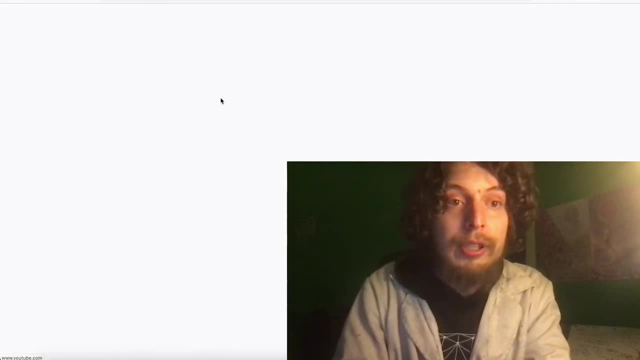 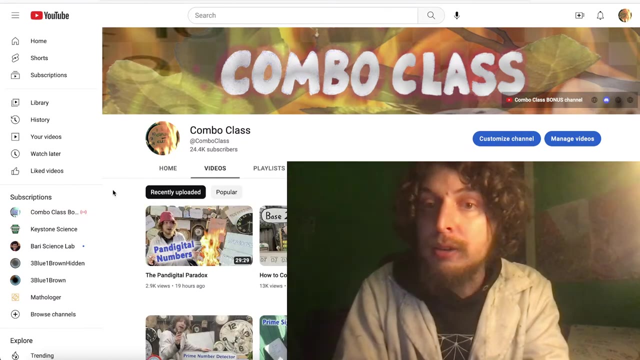 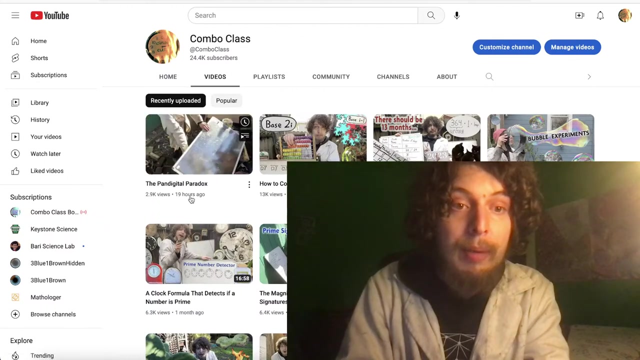 real quick just to show. even though everyone loves this bonus channel because of the shorts and the live streams and stuff, remember that my most thorough dives into topics that I'm most proud of are on this main combo class channel. And here's the new episode I put out 19 hours ago. 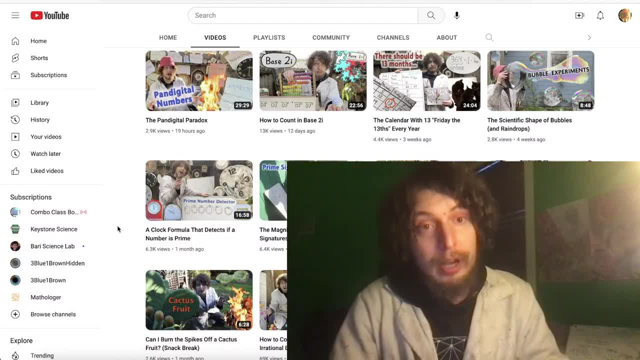 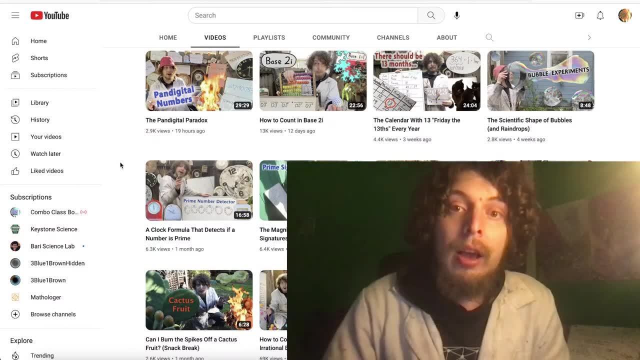 that make sure you watch that after the stream. Super crazy stuff about pan digital numbers that this stream only scratches the surface of in comparison to the episode. But some other episodes apart from that that are related to these strange base topics are obviously. there's three that are about: 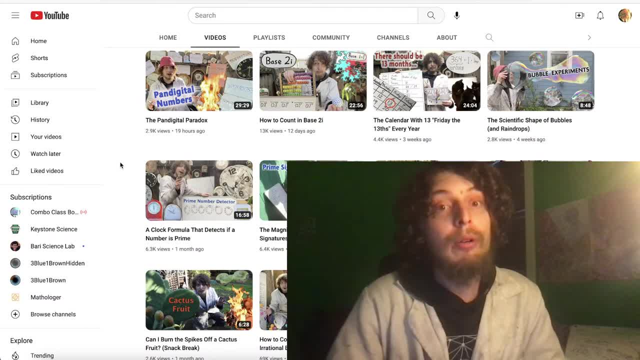 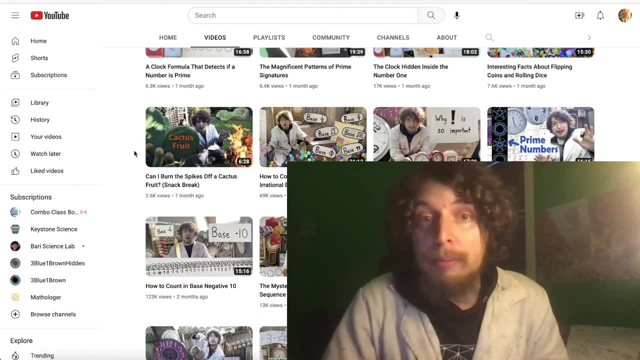 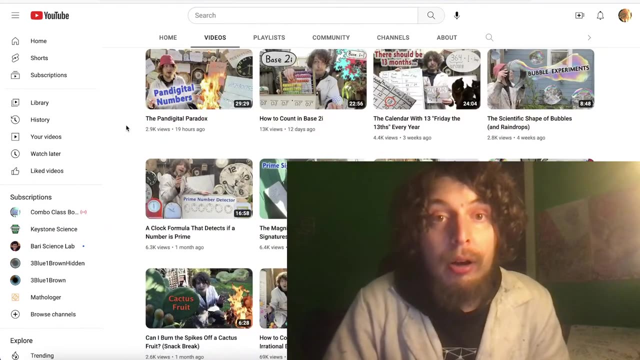 how to count in weird bases. that's in their name And those are about what happens when you go to a really weird base. So like base 2i and other complex or imaginary, all these weird fractional and irrational bases or negative bases. So that's sort of a little trio. 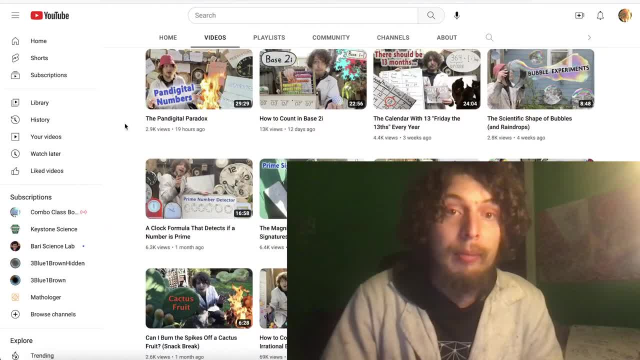 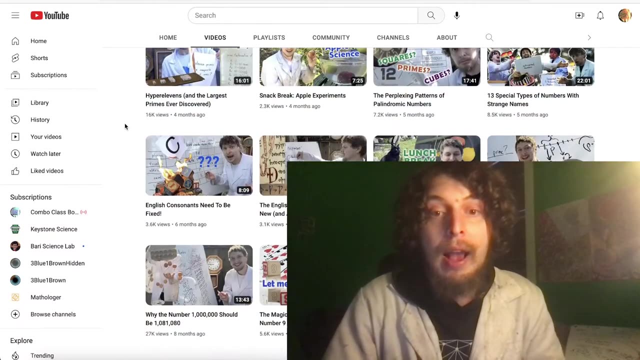 that are about more obscure types of positional base: what number you're taking the powers of being a weirder thing. But there's also some episodes I've made that are just about a single topic and end up going down a rabbit hole of what happens with that topic in other bases. 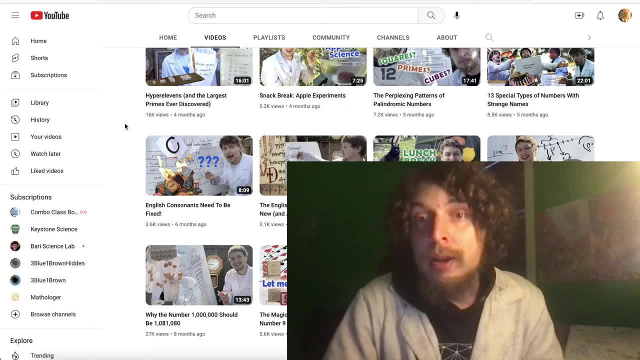 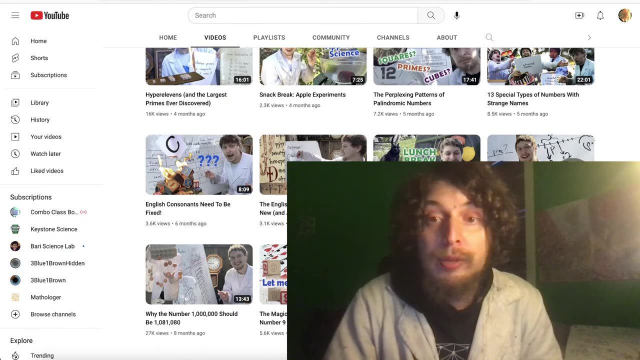 And that happens to a degree. whenever the topic starts out being a base dependent topic, For example, we're not gonna need to talk about other bases much in an episode. about prime numbers necessarily, I mean it could come up, but maybe less often, because prime numbers 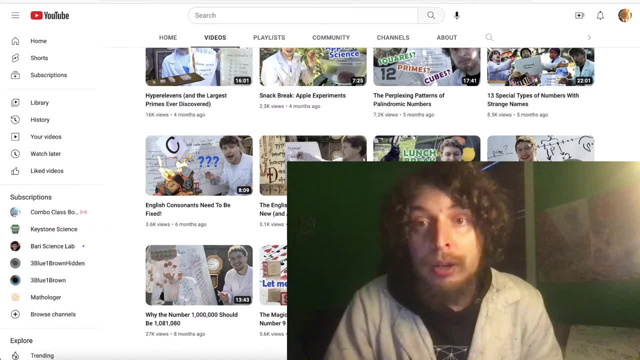 are based independent. the patterns mention with them would probably be the same, just with a quick translation. if we were in a different base, not different answers like some patterns would have, And one of the first episodes I made is Magical Properties of the Number Nine. That's when I spray painted nine on the side of the house. 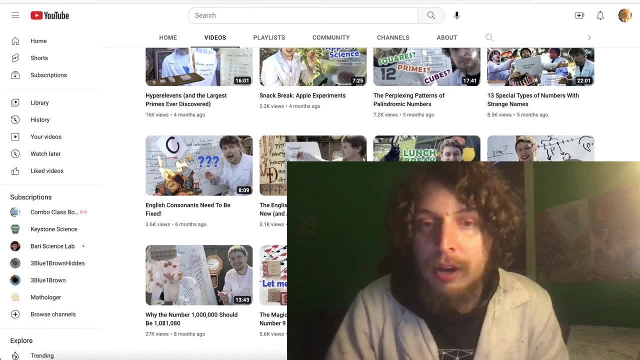 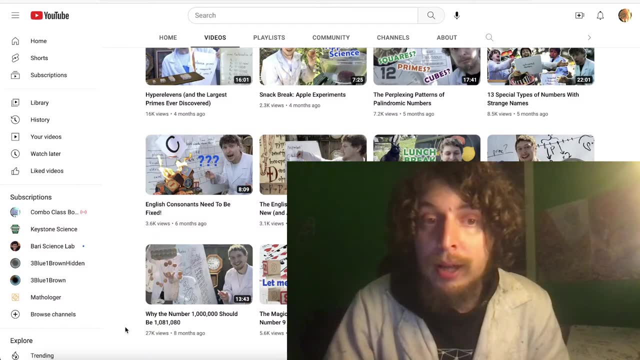 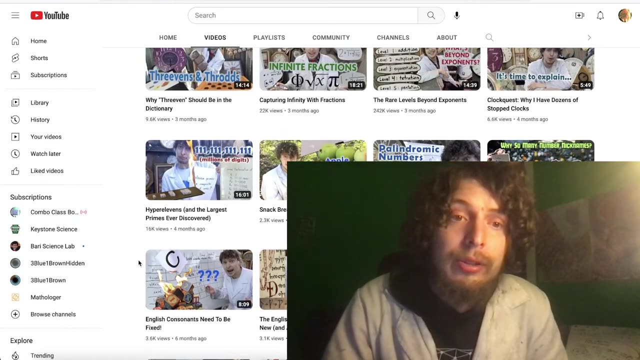 and ranted about nines and started off the first non-intro episode of the show, And in that one I do turn into an equation about what these traits about nines divisibility means in other bases. And then a little bit later here there's one about Hyper 11s. of course That one is. 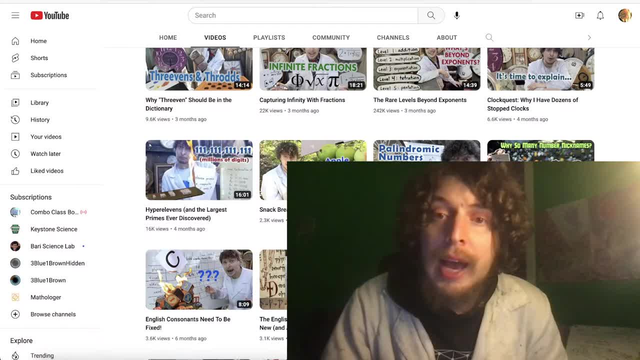 I would definitely watch that And to a degree the prequel to that is this: 13 Special Types of Numbers with Strange Names, Because those ones, to a degree this is also a prequel to that. These are sort of like a little trio. 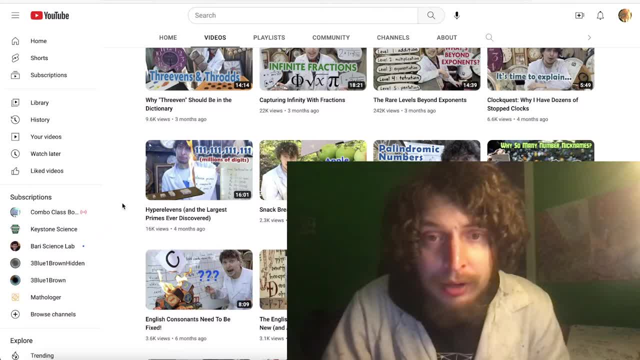 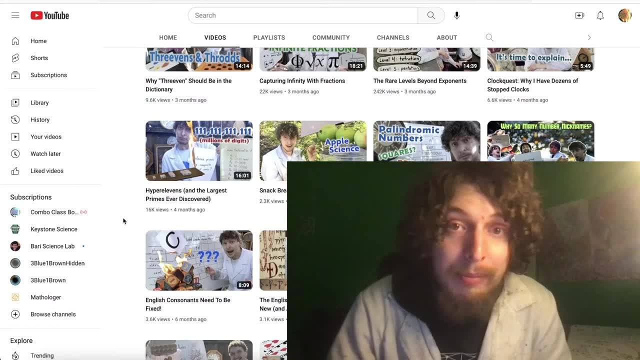 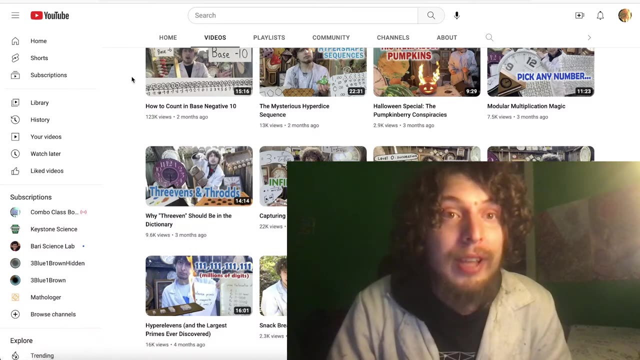 Hyper 11s is about those numbers that are all ones in different bases, but also these palindromic numbers went down the rabbit hole of different bases. So I also recommend the palindromic numbers for different base heads And yes, we can, if we need to name these type of numbers that have. 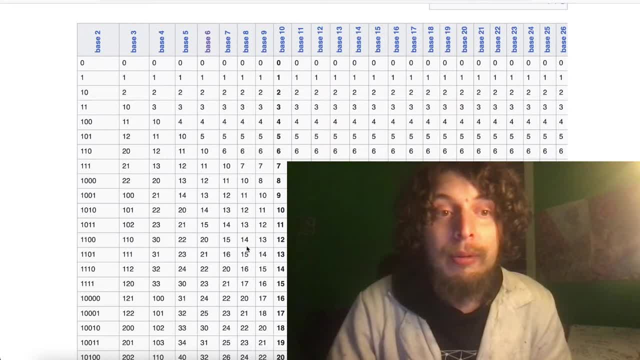 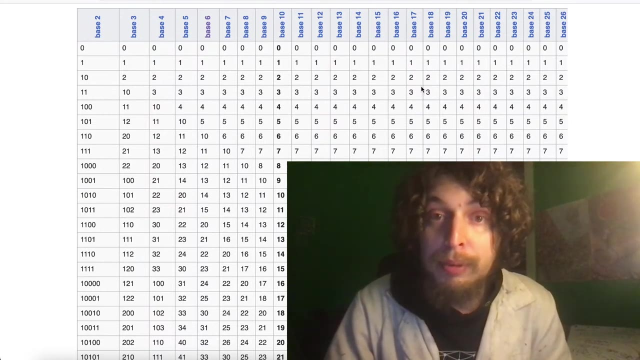 properties in different bases. if we find something cool, we can call them something like hyper-based numbers. So, and for people who use the term based as slang, just remember where it originated from: Lil B, the bass god, A very strange, innovative rapper and creative soul. 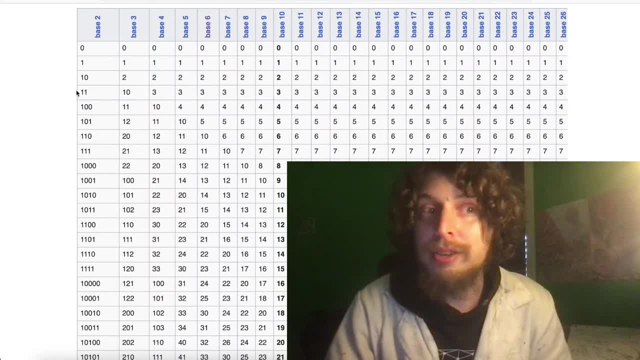 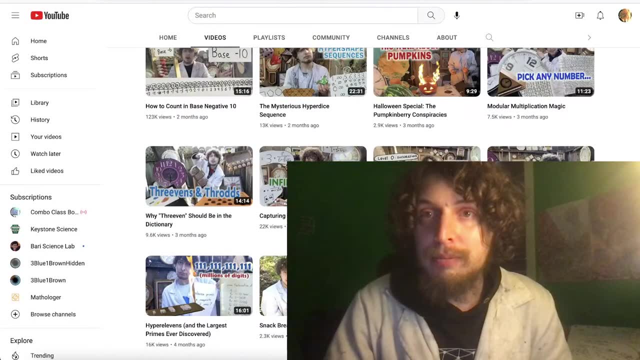 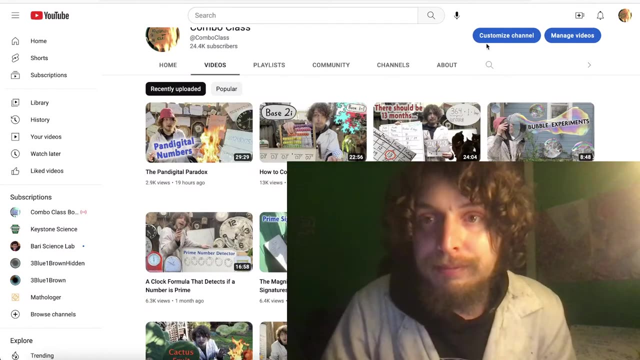 So, as long as you remember the origins, it's a good word to use. Now, that's most of the crazy base ones, apart from the ones that are titled about different bases, And then the new one, of course. Now, in the new one, it's not just about fun facts about pan-digital numbers, but it's also about 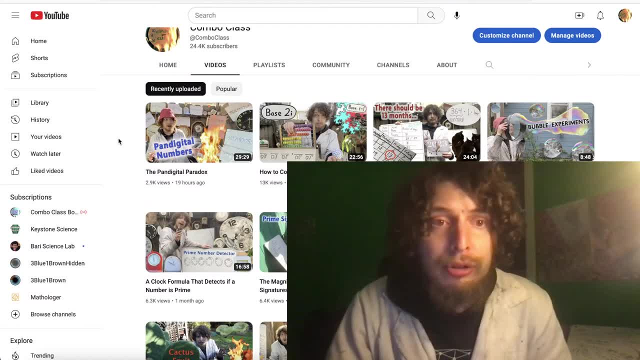 crazy paradoxical things you encounter when you try and compare or analyze larger stretches of number line approaching indom comments. And thank you for joining me. Let's see how long we've been going, for It has been Uh-oh, what happened. 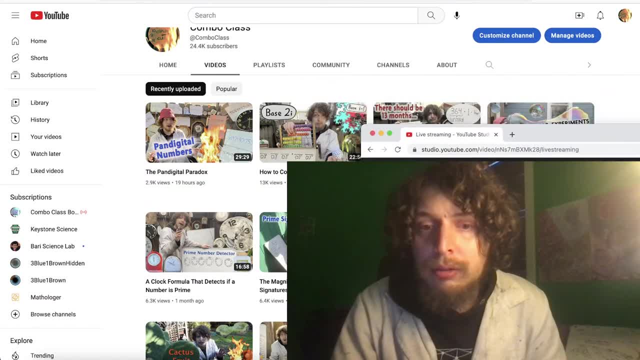 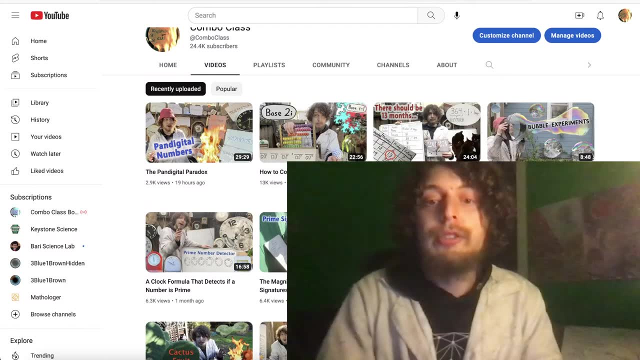 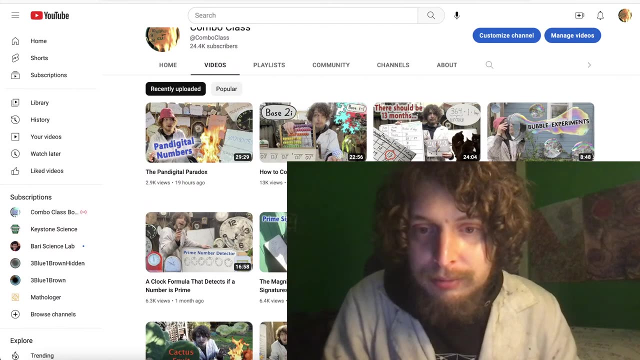 Oh no, What's going on? Sorry, my internet's being super weird. Hopefully it'll work. I need to sometime figure out why my internet gets weird sometimes, So hopefully I'm coming through at all. Thank you all to everyone who stays around, even when glitchiness occurs. 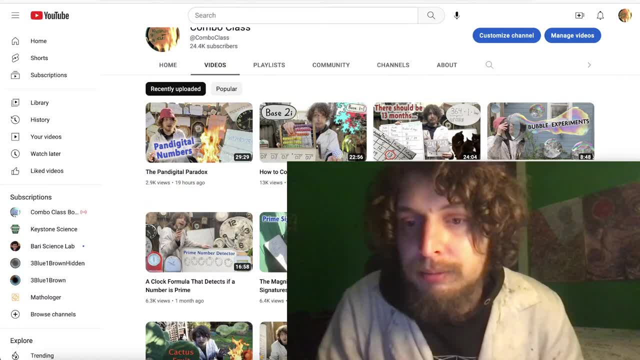 I think we are good to go now, though. Now on this stream, since we've been going for a while, I'm not going to go a crazy amount more of time, So people can feel free now if they want to leave any other questions they have. 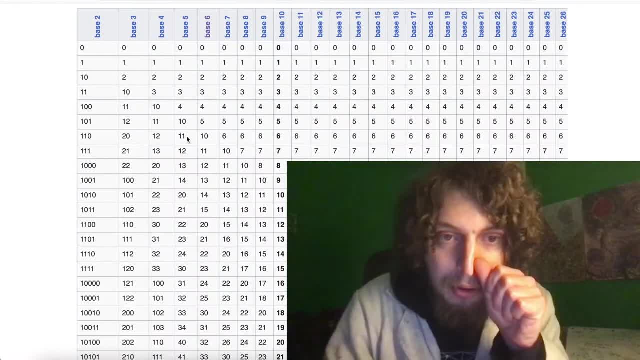 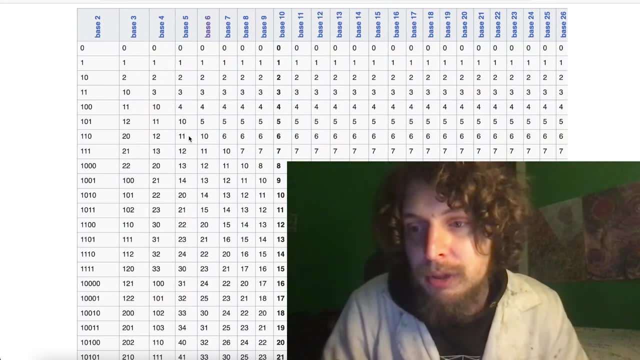 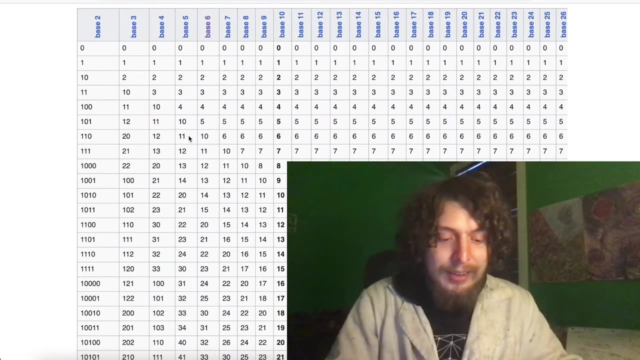 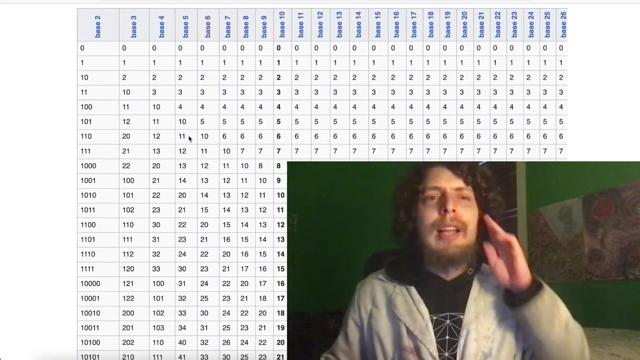 either about these strange bases or in general. I will be investigating more of these as time goes on, So strange bases will be a recurring concept, although, of course, in between that, I'm going to need to use Base 10 to communicate it all in an understandable way. And let's see what else we have coming soon. 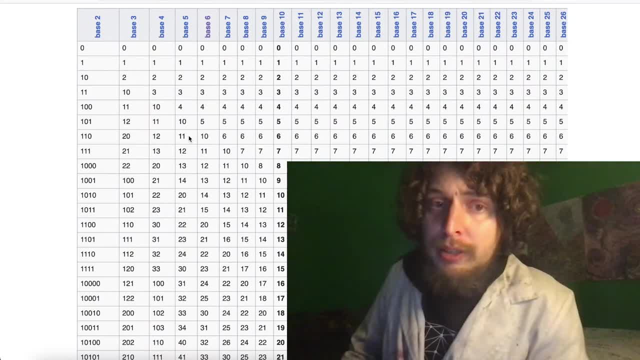 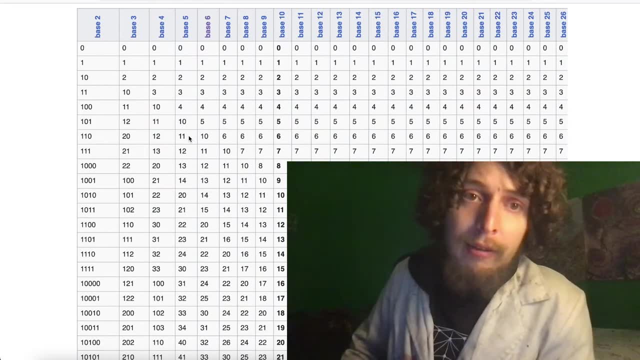 So I'm still pretty busy this month with private teaching and stuff, but I think that starting next month, I'm going to cut back on a lot of my private students and have more time to focus on them. So I'm going to be focusing on my private teaching and stuff. So I'm going to 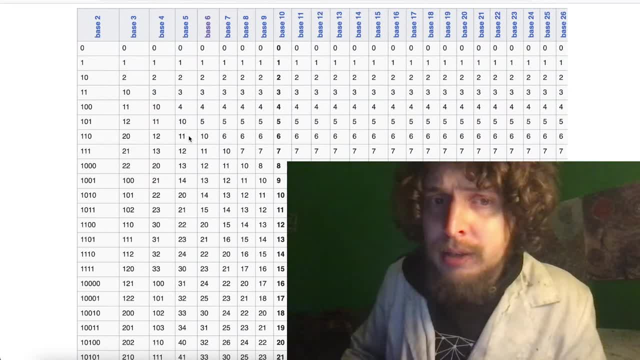 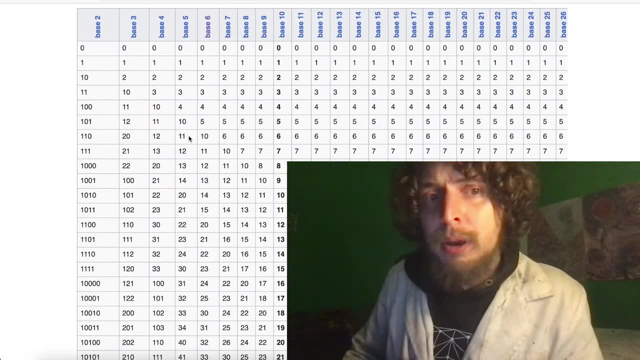 be focusing on my private teaching and stuff. So I'm going to be focusing on my private students on combo class, as well as some writing projects and physical therapy and stuff i have to do because i got a bunch of surgeries last year so hopefully that'll give me time to for next month in march. 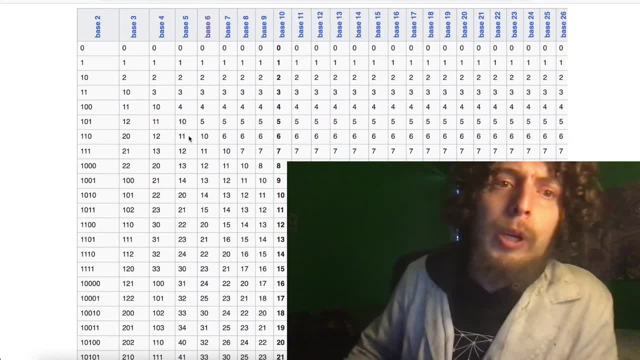 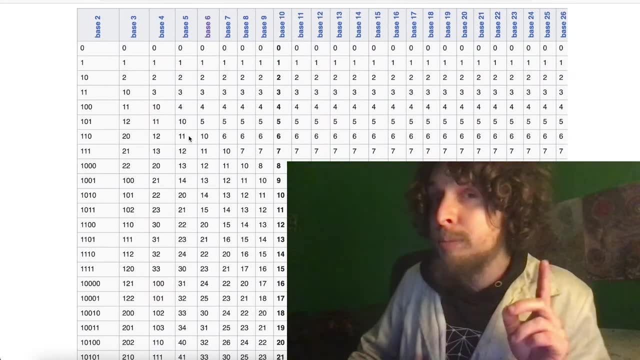 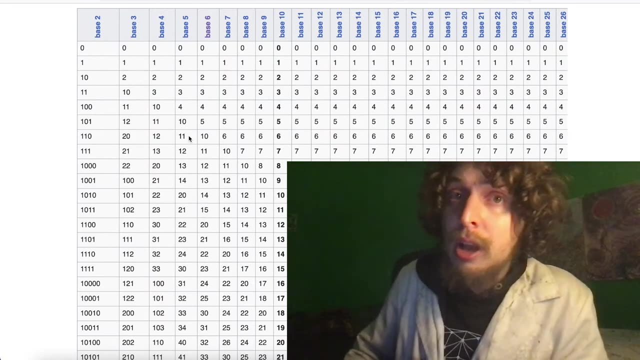 have a clearer streaming schedule of which days i will be streaming. i also will be, like i mentioned last, stream sometime before march opening a po box here in california for people to send their old, broken clocks as well, as if you have any dice, and they will be things that may get. 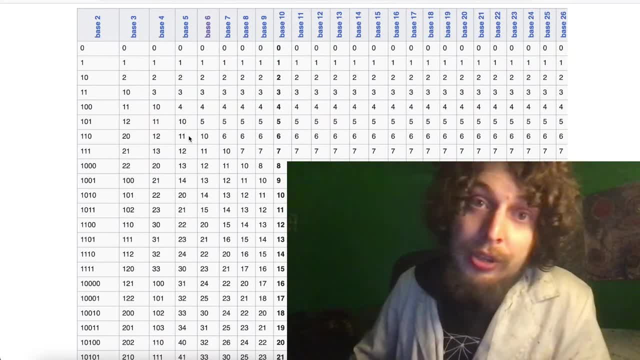 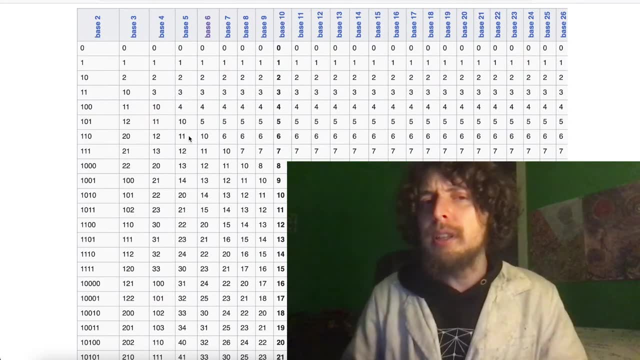 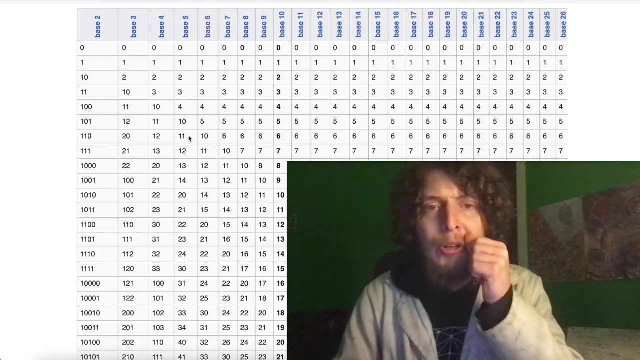 destroyed but will probably end up in the background of an episode and gain a historic role instead of getting dust on a shelf somewhere. so i'll definitely let you guys know in a stream and or short or something when i have the address for that sometime before march. so take a peek out around your house, around. 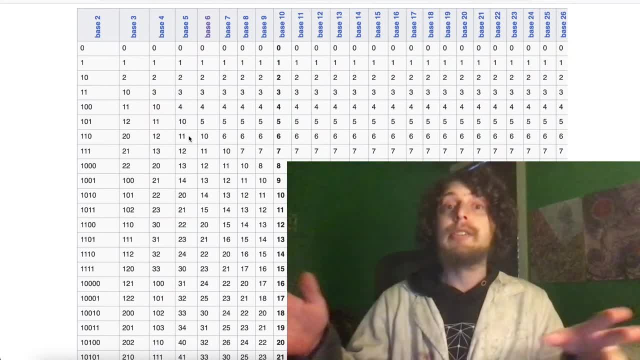 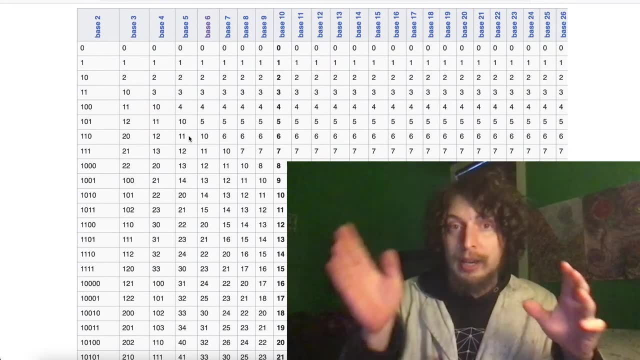 your storage, your attic and basement and whatever got any clocks that are just collecting dust, that aren't helping you out. they do have to be analog looking clocks. they can't be digital clocks. they have to look like a clock. but if you got any laying around collecting dust, you know who to 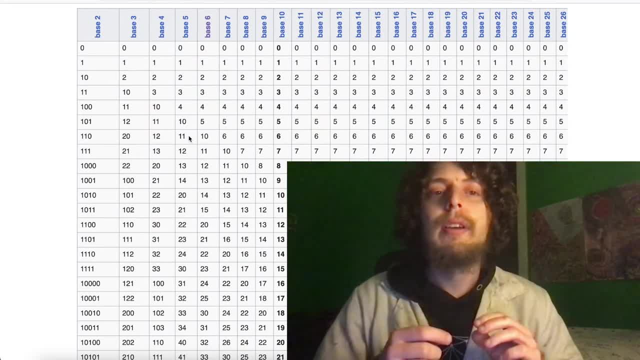 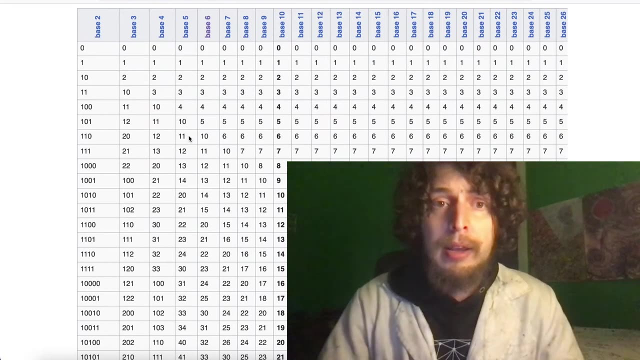 send them to in a month. so in addition to that um in march i i i will be also working more um schedule wise, with a few of my camera people. one of the main camera guys, carlo, as well as a guy, johnny, who i've filmed some of the episodes with. 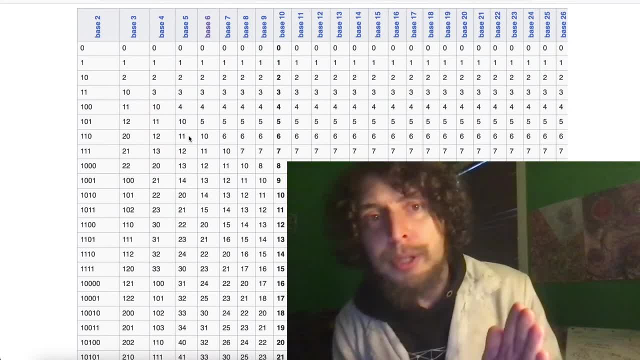 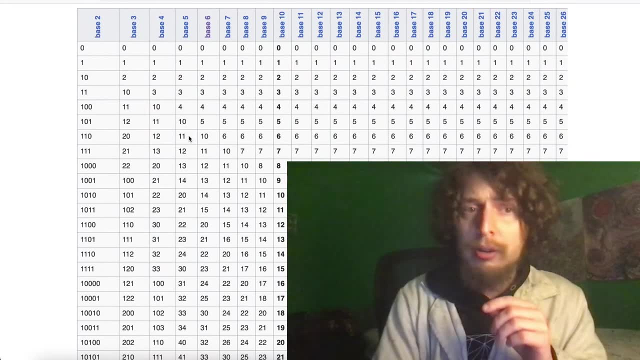 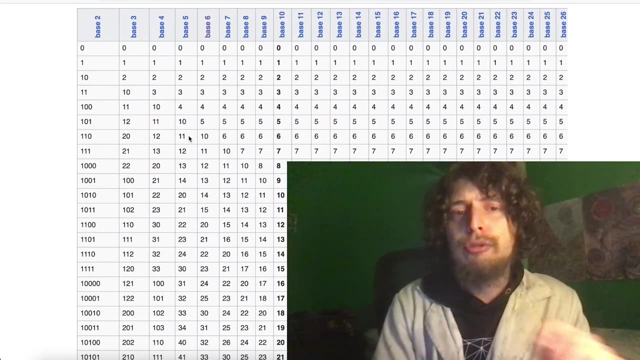 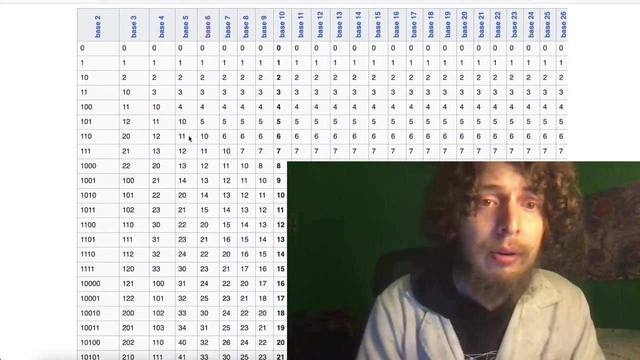 to work on the remaining five episodes of grade negative one to finish, most of those in february and early march, although they will be released throughout february and march, so that in march i can transition toward grade negative two, which will require me getting a haircut, getting a new desk, throwing away or destroying somehow a bunch of things. 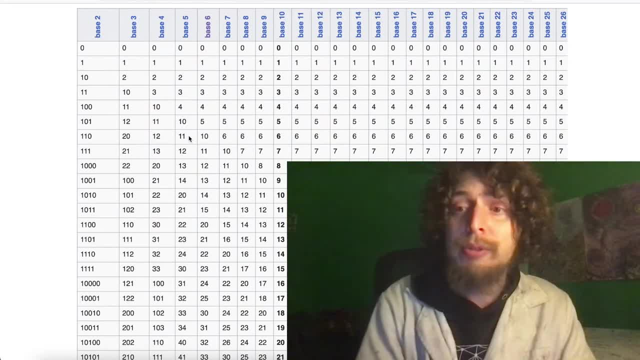 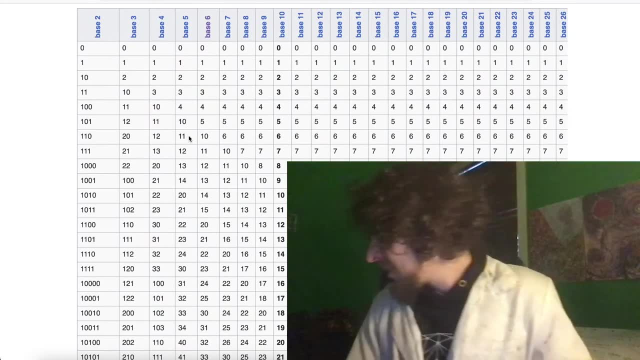 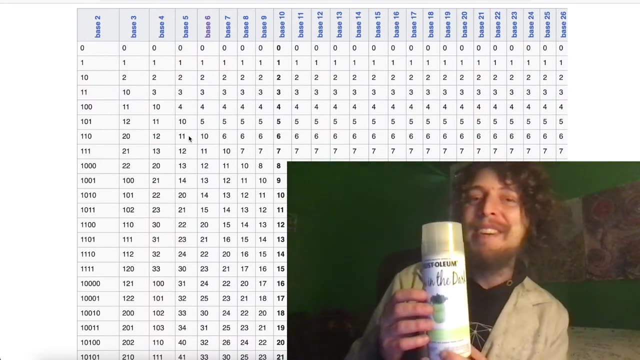 getting a bunch of new classroom supplies restocked and other things that may be a surprise. until then, maybe i'll have to use this new thing i got, which is glow-in-the-dark spray paint, so that'll be pretty fun. maybe we'll have to put some of that up in the classroom for grade. 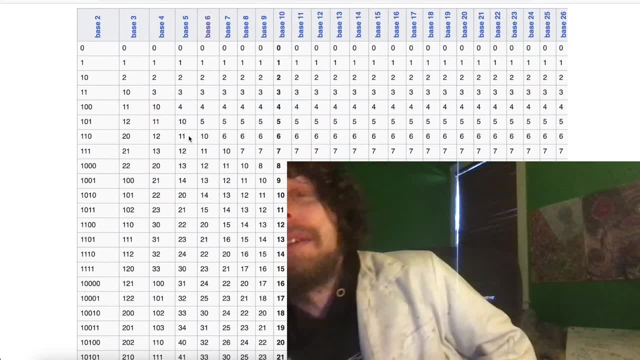 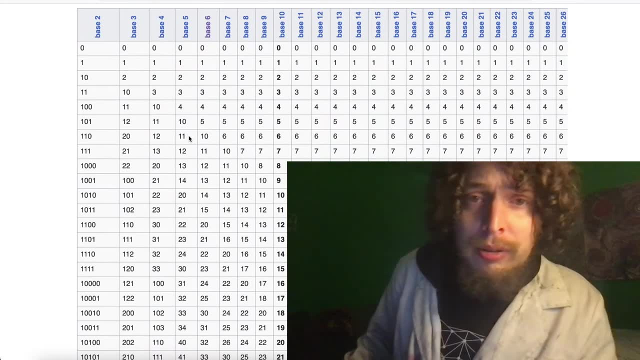 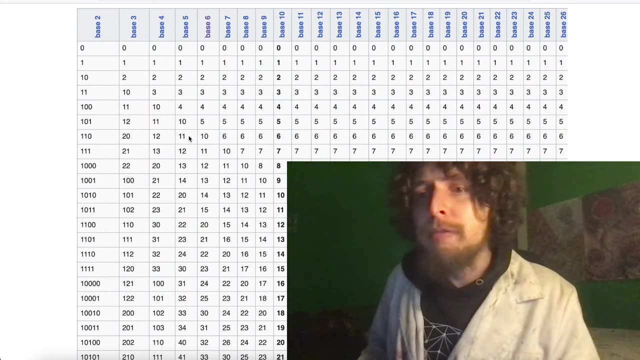 negative two, and maybe you won't even know right away when it's up until it starts getting dark, and the remaining episodes on the channel will be about a week to a week and a half apart from each other. a few of them will be just around 10 or 15 minutes, but a few of them will also be really long. 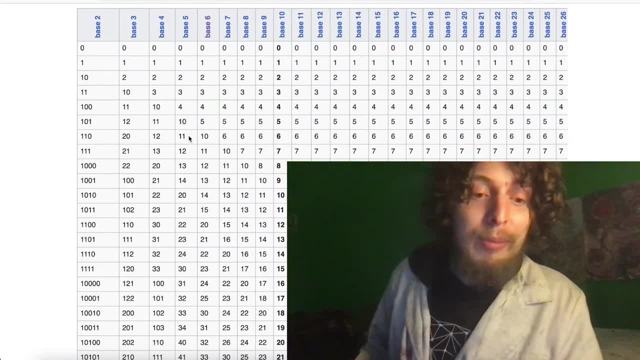 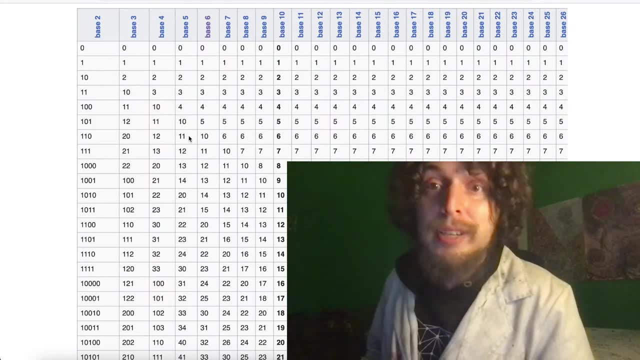 ones like the pan digital one was because some of them are topics that i've been planning all grade uh, hesitated to make because i wanted to make sure i got them correct and as good as i could get them, and now that we're near the end of the grade, it's time to turn them into something. 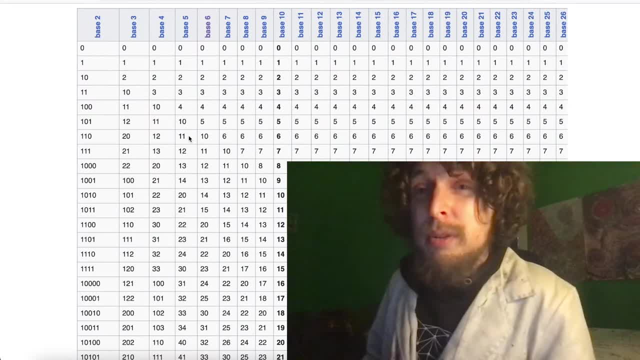 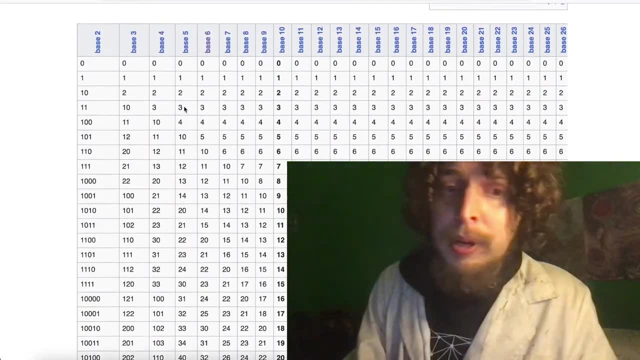 and i'm not even sure exactly, for one or two of the episode slots that i have remaining, because we're going for 36 episodes, which is in base 10.. i mean it's in base 10, it's 30, it looks like 3-6, but 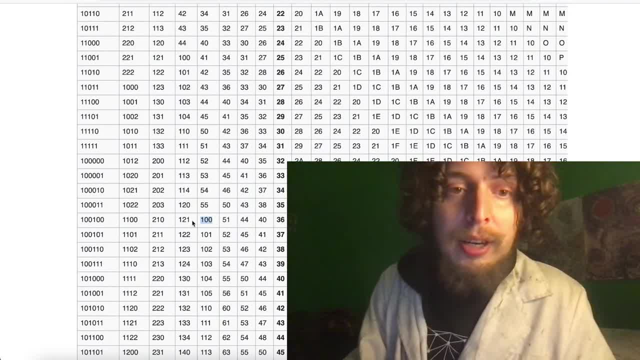 base six it looks like one, oh, oh. and hey look, it's palindromic in base five. hey look, it's also uh, a rep digit, not a rep unit, a rep digit in that base. so we're going for uh. and it has zeros in a bunch of bases because it's a divisible number. 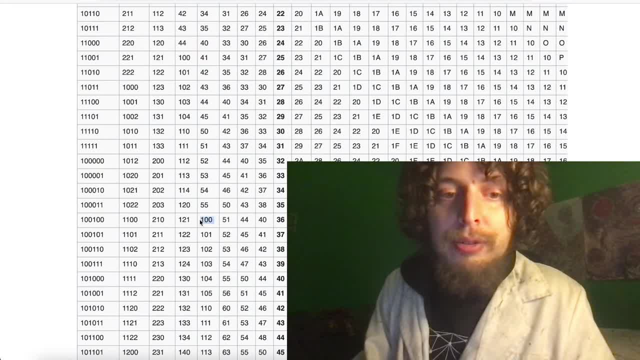 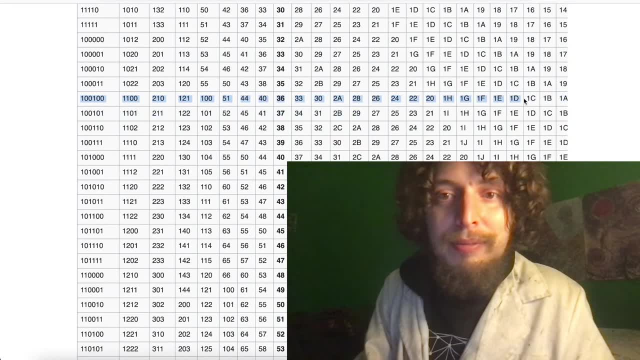 we're going for that many episodes: one zero, zero and base six. the number we know is 36, or how all of these bases might write it in different ways- and that leaves five more episodes on the channel, and that includes a finale that will be more behind the scenesy and, uh, include some rare footage throughout the grade that was never released. 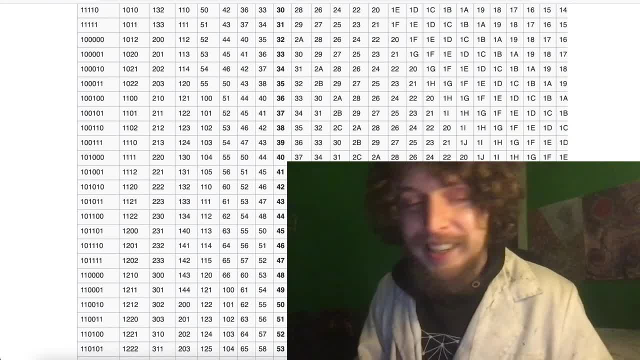 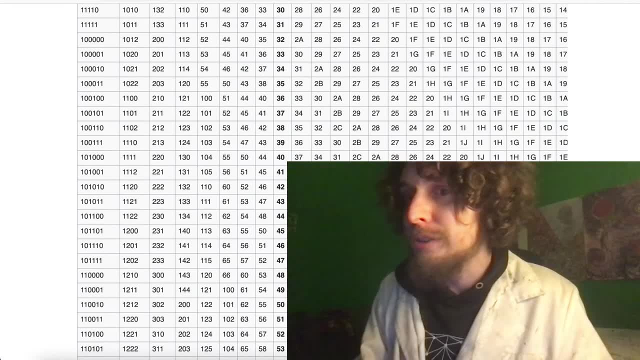 and will all be really long, probably. so part of what i will be doing in march is putting together a crazy finale in addition to resetting for next grade. as far as february, the episodes will be normal, maybe some of them more like a week and a half. 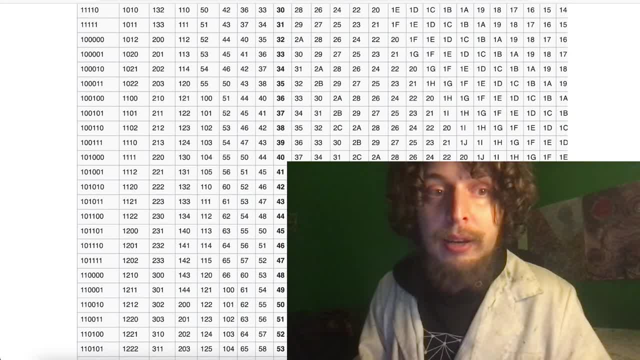 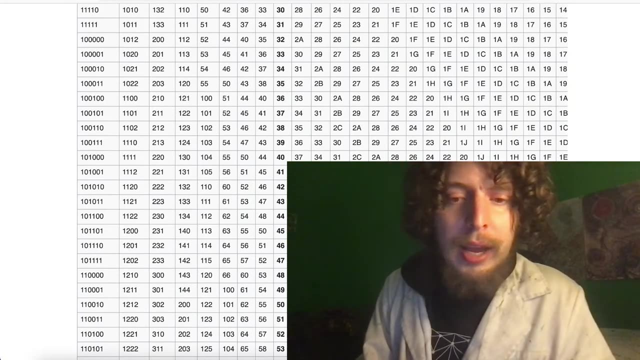 apart from each other. instead of a lot of the time it's been like a week or less. uh, some of these are now going to be, maybe, you know, like eight or ten days apart, so i can get them extra cool and extra good, and a few of them are just more silly, playful topics, like one of them that i need to fit in the. 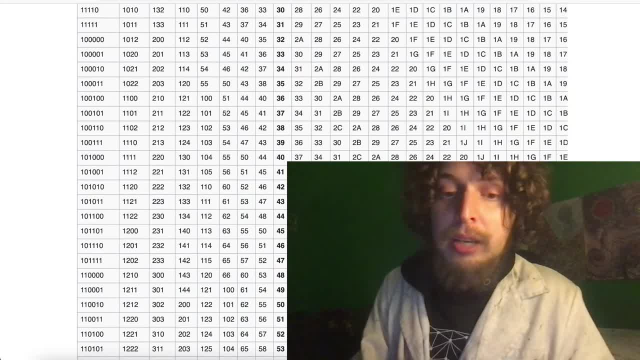 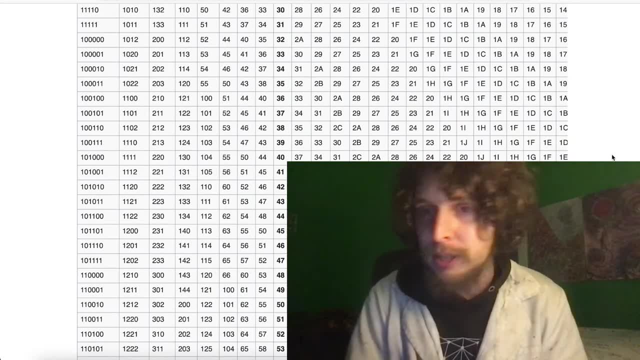 grade, just because it's time to fit in, is one that's a mix of language and writing. it's sort of another language episode, which i did a few before, which usually end up being roasts of language, but this one's about spelling numbers, and so it ends up almost like when we look for 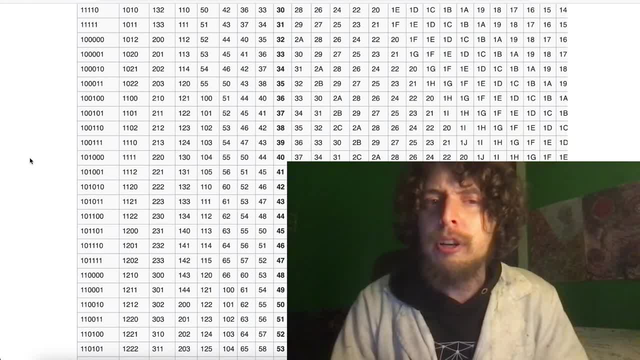 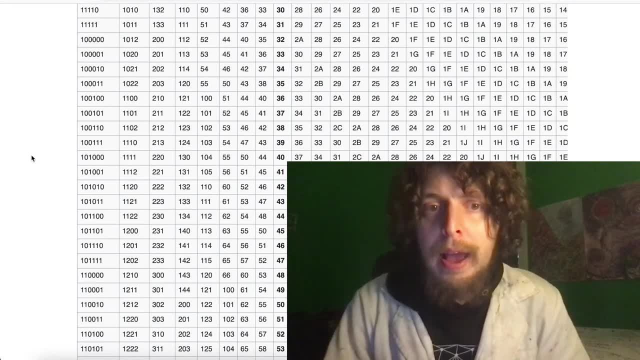 traits in different bases, uh, being similar of. we're going to look at english and see some crazy, surprising traits about how numbers are spelled and written and using letters, and we could, you know, guess about or figure out traits that might be necessary for any way of a language writing. 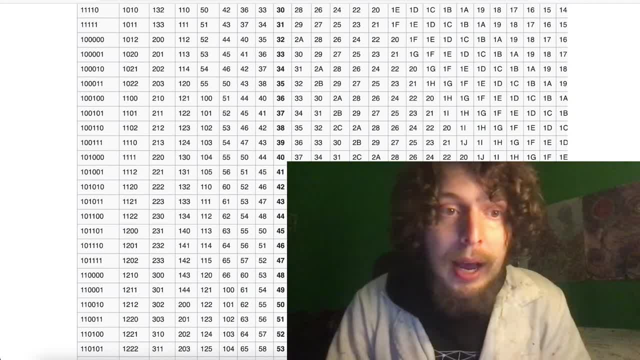 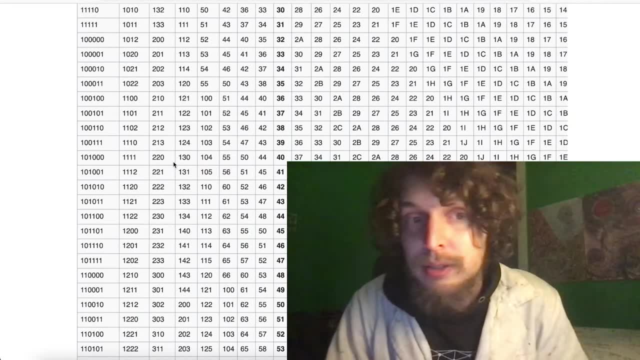 numbers, sort of like we could use base 10 to get clues about what traits other bases might have. if we wrote numbers using digits, it'll be like that, but using letters instead almost also reminds me like using alliteration in some titles like pen digital paradox and like ones with the same uh. 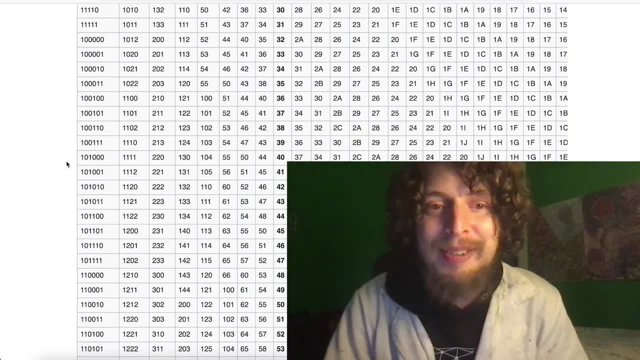 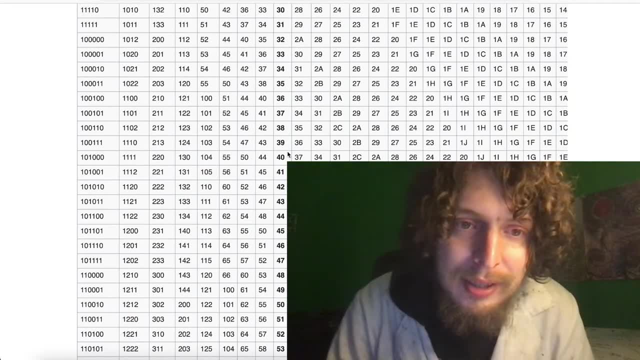 beginning letter. that's something that you know. only happens to be like a language dependent trait for it to work. but you know, if you're stuck in a base, might as well enjoy your base dependent patterns. if you're stuck in a language, might as well enjoy some alliteration. 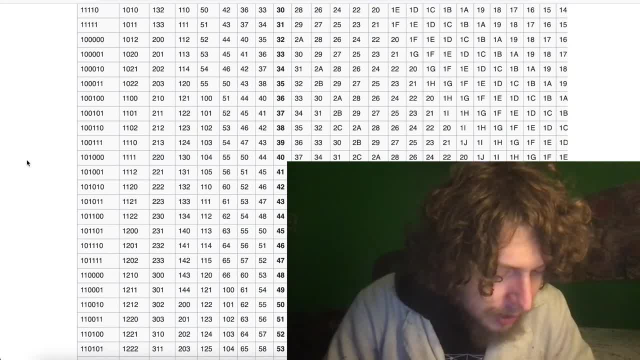 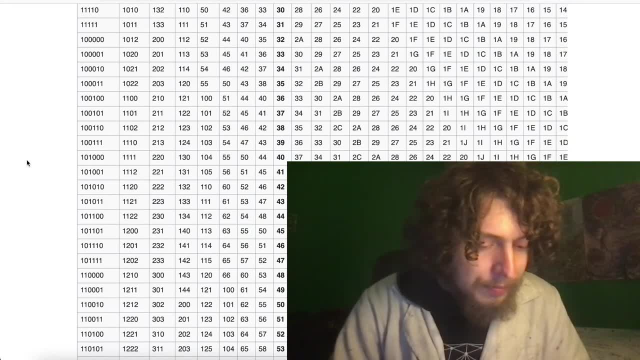 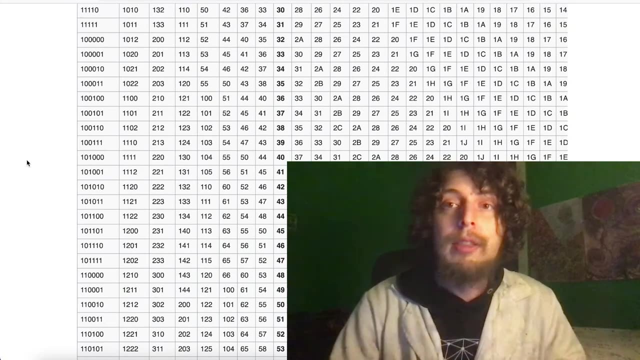 so hello to everyone here saying hi, and someone's wondering if there's anything cool about the number 2008, and i believe there probably is. i don't know anything off the top of my head, but one thing that we can do if we're ever curious about a number is to either see if they happen to have 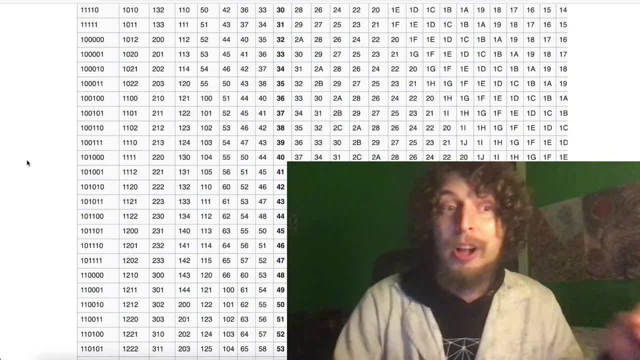 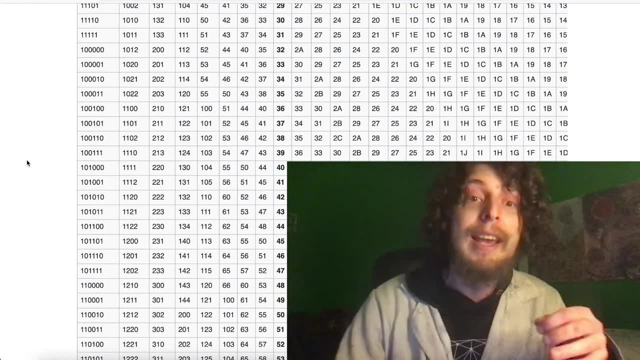 a section for it on the wikipedia article for the smallest round number under it. so they'll have a wikipedia article for 2000, for example, and we could see if 2008 shows up on their wikipedia article and we can actually look at it and see if that's. 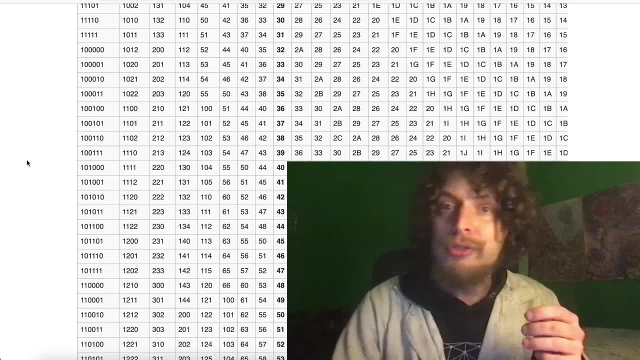 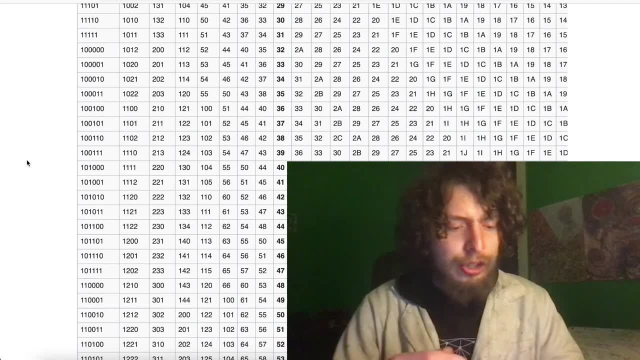 interesting enough and we could also look at it and see if there's anything interesting that they're going to mention there when they list some bonus numbers. and we also could look on the oeis, the online encyclopedia of integer sequences, and there analyze. does this show up in any interesting? 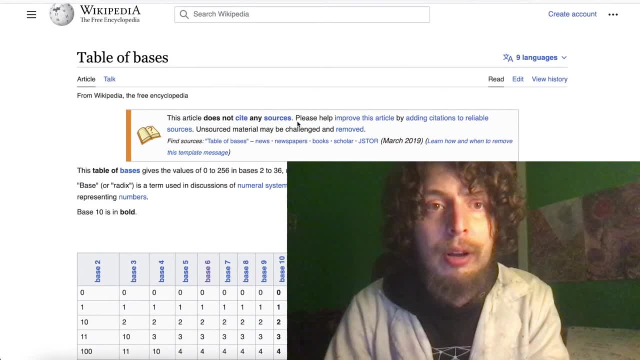 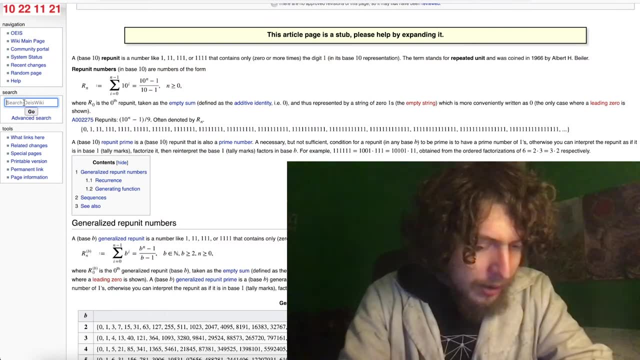 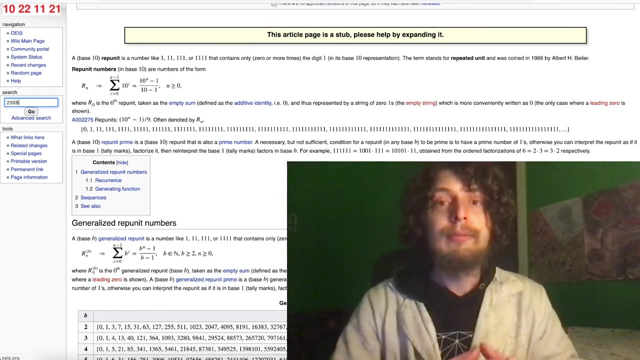 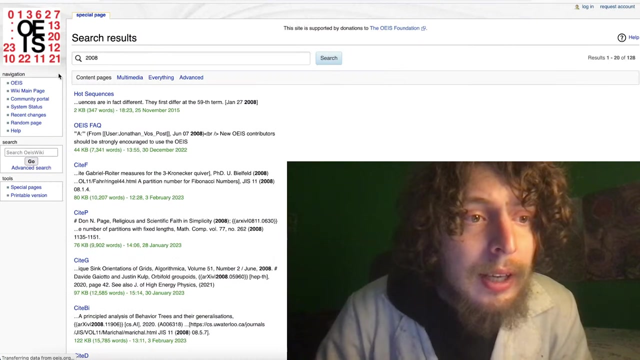 sequences. so let's take a peek on that oeis um and see if 2008 shows up, and we'll also search it here. on wikipedia is- And hello to Brian McLogan there, Good to have you- And we got 2008.. And that was. 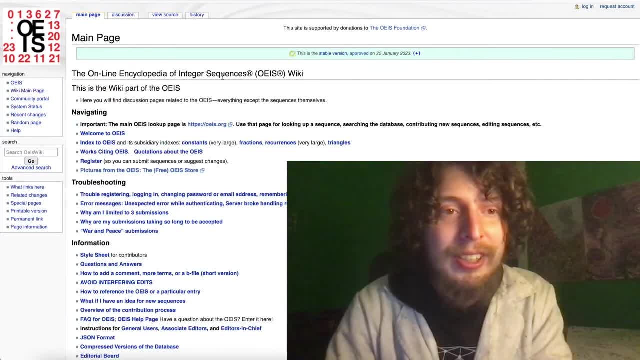 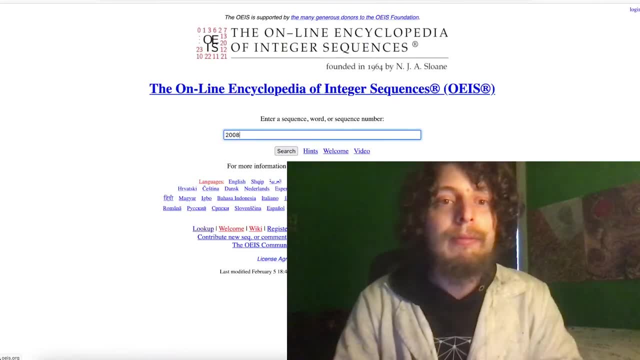 searching in the Wikipedia sector of it. So we got to go to the homepage actually, So just to the OEIS, And we're going to see what 2008 shows up in, And some of these may be the facts that Wikipedia gives us in a minute as well, if they have any, But it's. 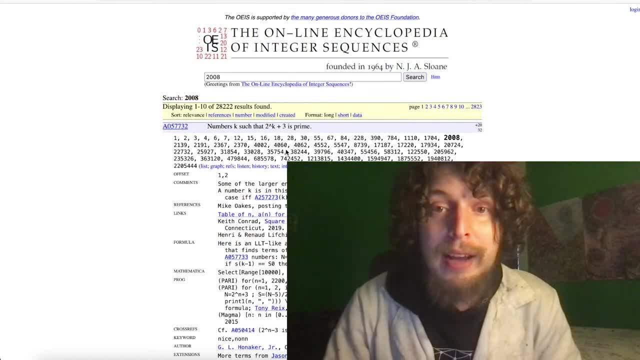 kind of fun to see it in context. So this is kind of a random one that must have been important for some particular problem. It is a number such that twice it or two to the power of it plus three is prime A little random. 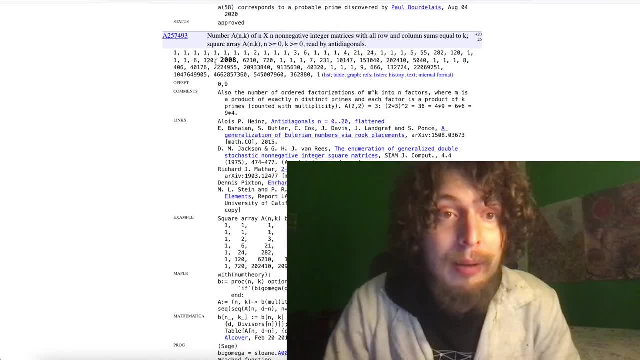 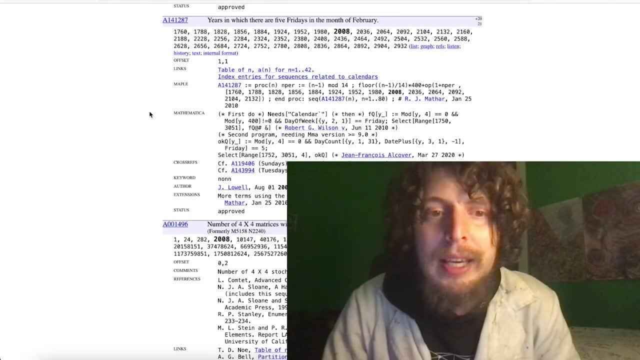 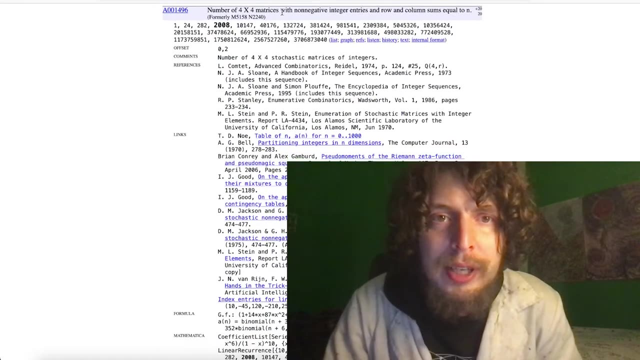 Here we got one that it is the only number in quite a big range of this trait And this is a very arbitrary one. It's about years. I'm almost surprised they put that on here. This is interesting. Number of 4x4 matrices with non-negative integer entries and row. and column sums equal to four, I guess, Unless what's the offset here? Let's see Equal to three. So there are exactly, apparently 2008 4x4 matrices with non-negative integer entries and row and column sums equal to three. Someone's noting number of 4x4 stochastic matrices of? 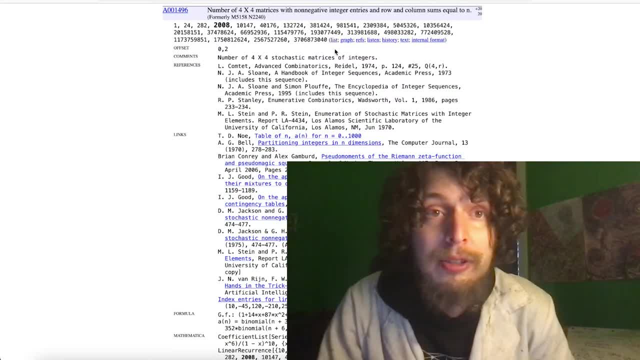 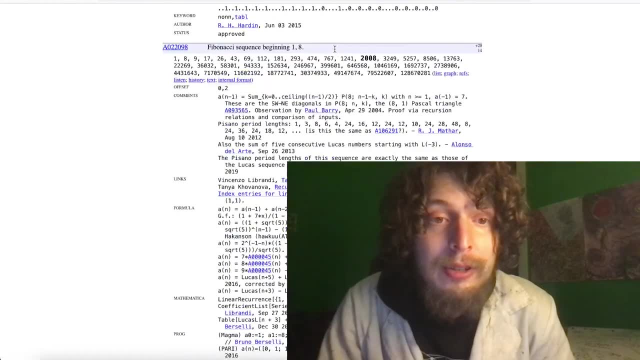 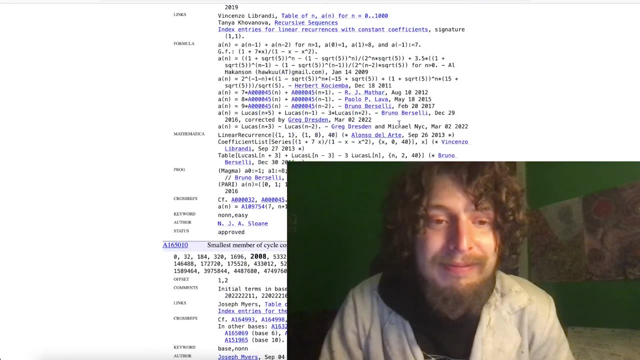 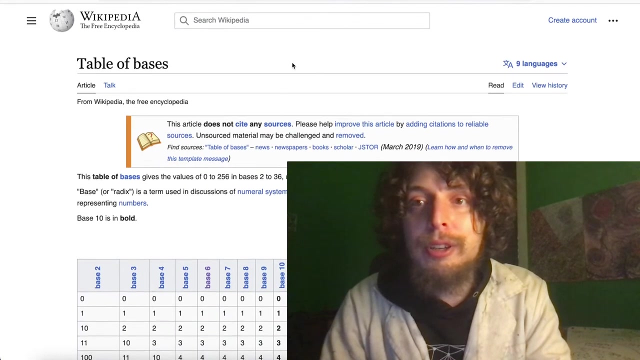 integers And we can also now look on if Wikipedia has any other ones. These are some other fun ones, And if you started your Fibonacci sequence with one, then eight, then played with similar rules, you'd get it Okay. so now seeing if Wikipedia has anything fun, we are going to look at. if they just 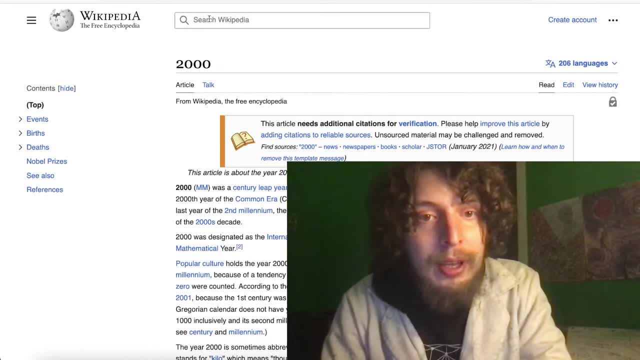 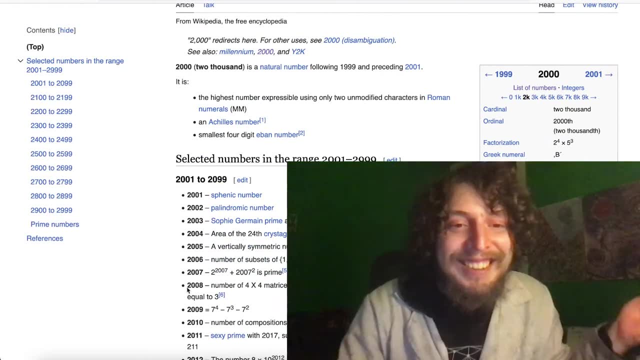 have the calendar year, then we've got to go for 2000.. And no, I don't mean the year, I mean the number, And here 2008.. Oh, that's the one they mentioned. They mentioned the one that I mentioned. 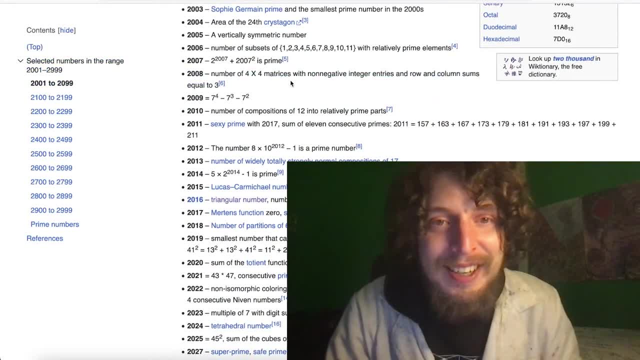 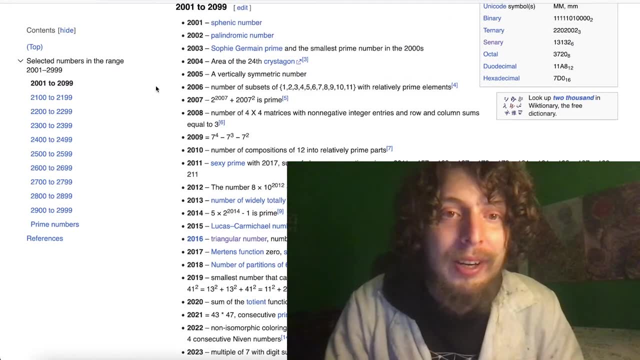 That I thought was coolest. They also thought was coolest It's the number of that that. I just said So to people who have other. I'm guessing that's like a birthday or an important year to you, To other folks who have birthdays in this range, which my birthday is a little. 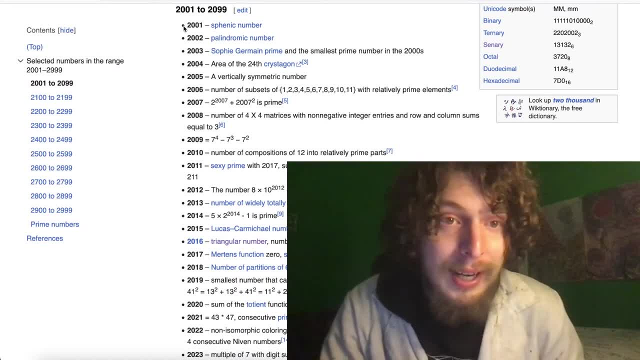 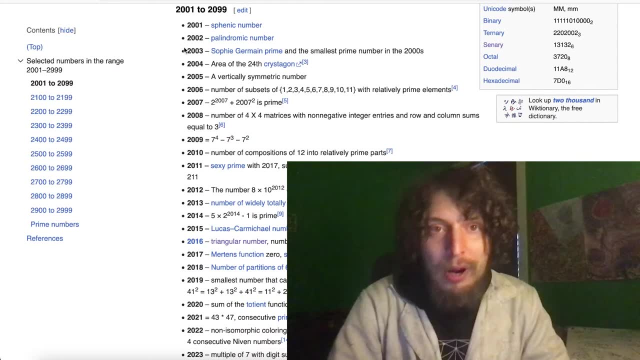 before that it's in the 90s, But here you got traits for most of them. You know you get your Stenic number year. That's a number whose prime signature is one comma one comma one, Or in other words a number that's made up of three distinct primes. 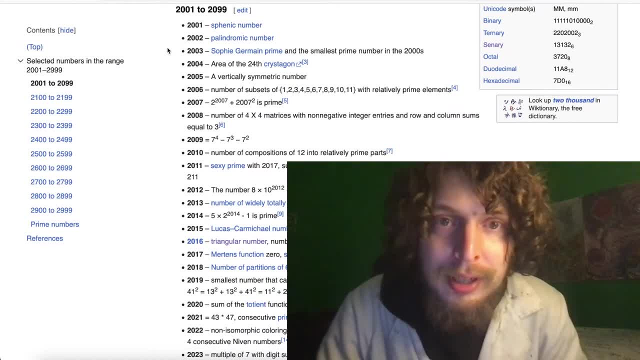 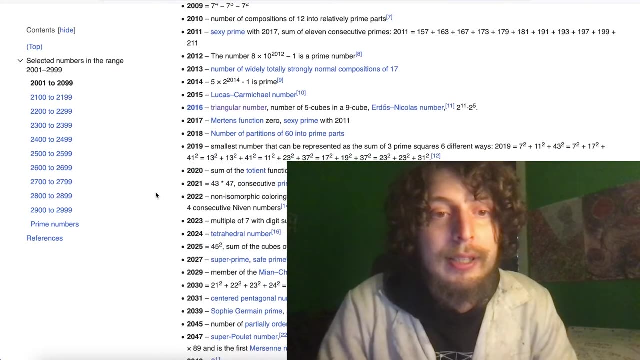 It's multiplied together, 2002 is palindromic in our base And then you get some other ones. Now maybe we'll look at that more in the future for some of the past years. Looking at some of the years that are coming up, I am pretty excited about the fact that next, 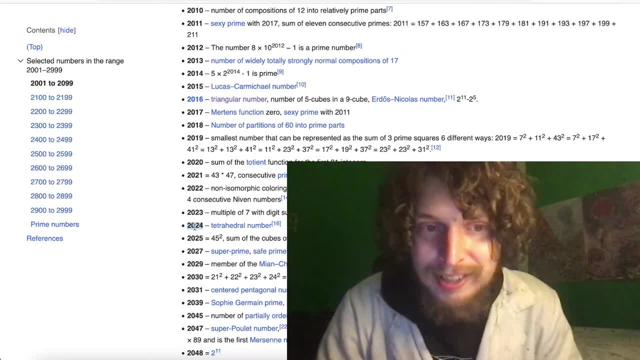 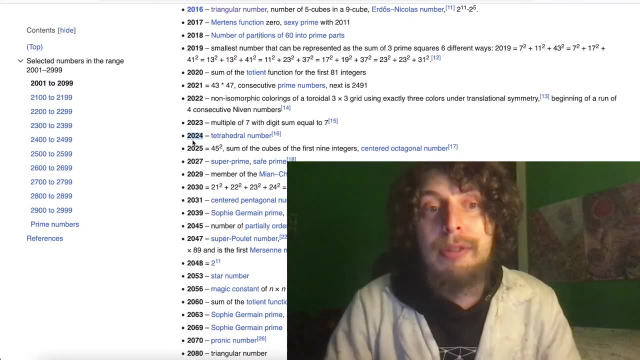 year. although it is arbitrary now that our calendar calls it that year, you know other calendars don't call it that year. stuck within this Gregorian calendar system, 2024 will be a tetrahedral number. That's when you add up all the triangular numbers. 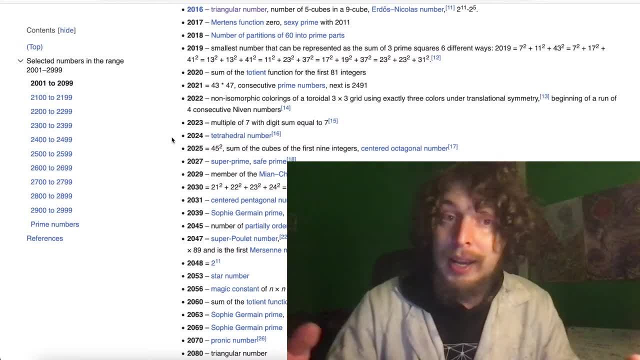 like, the triangular numbers are the sum of the natural numbers And, like you could say, the natural numbers are a sum of a row of ones. So we can find cool things about all sorts of numbers here, And that is even a fun game that we've played before that we'll play in the future is picking a number range and trying. 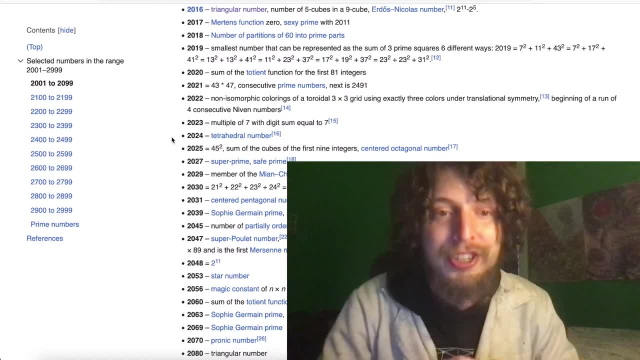 to find the least interesting number in that range. and least interesting is highly subjective, but we would, you know, learn some fun things while playing that sillier game. sometimes, if your silly game is using important tools or concepts, you end up stumbling into some important truths or questions anyway. so when that tetrahedral year comes, 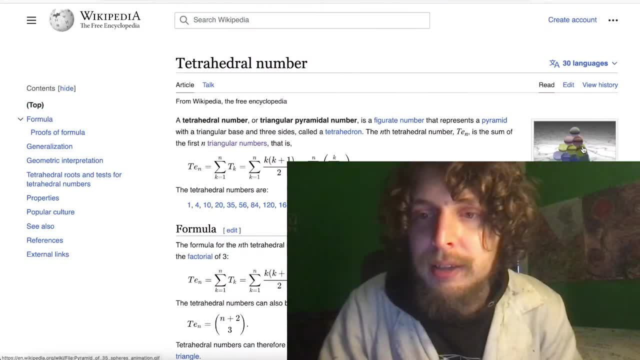 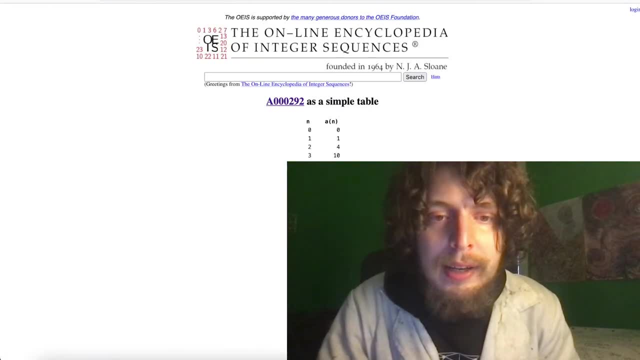 we are going to make a giant tetrahedron like. you see this rotating tetrahedron there. well, the tetrahedron we're going to need is going to need to have a height or amount of layers of 22, so that's pretty big. i'm going to need to buy sometime. this will be in late grade- negative. 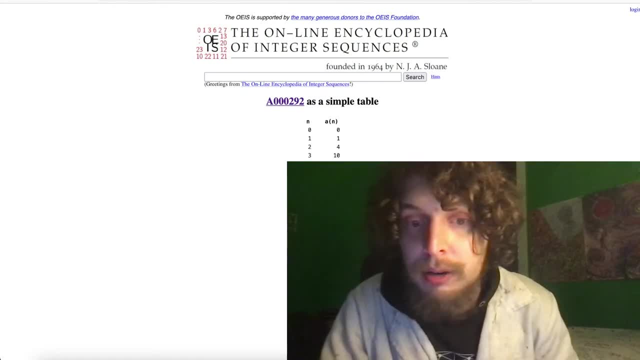 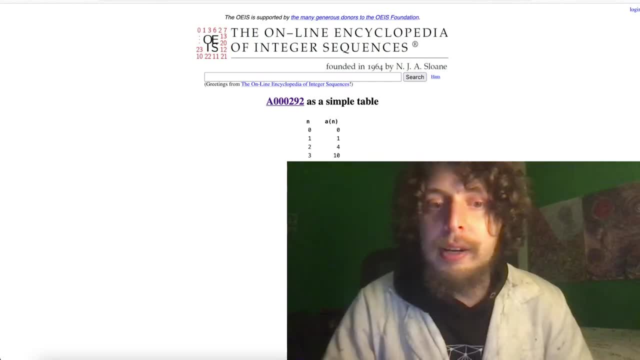 three. that'll still probably be some point in this year. i'm gonna need to get 2024 marbles and a ton of glue or something, because i want to make a tetrahedron for the year. so, uh, thank you all for joining me again. i am going to log off pretty soon because this stream. 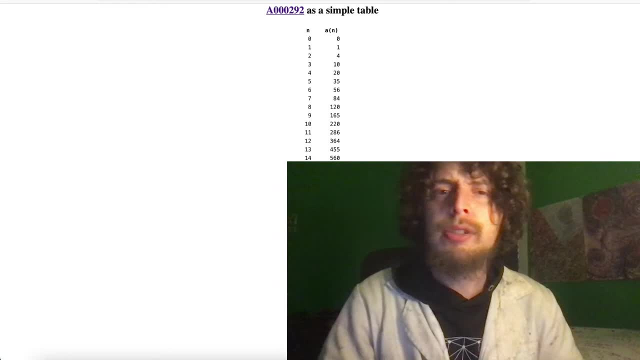 is just going to be about an hour. i may post a short or a bonus video later today as well, but remember that on the main channel. uh, for those who haven't seen, that new episode about pan digital numbers is one of my favorite ones i've put out. it is the longest one on the main. 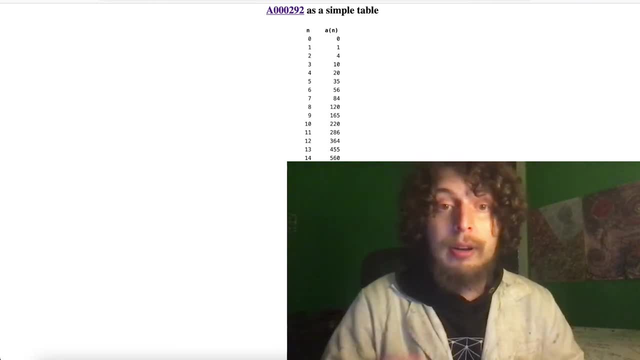 channel and i'm pretty, you know, trying to be pretty concise with my editing and phrasing on those episodes, compared to in these streams where i'm a little more free form and so the length of the episode isn't usually on the main channel. just that i was ranting a bunch. 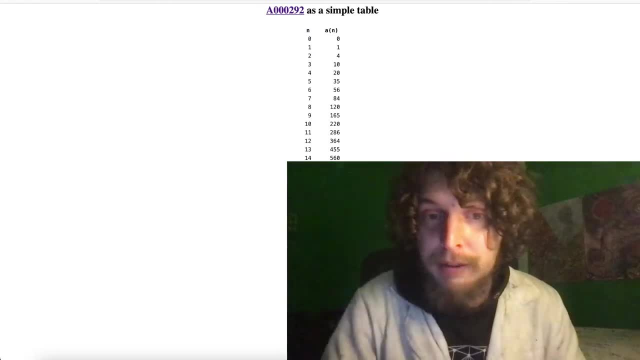 it's a longer episode. it means there was like more subtopics i felt obligated to put in and of course i'm going to give my obligatory of the stream. extra thanks to my patreon supporters and a recommendation that other people check that out if they want to see various bonus content. 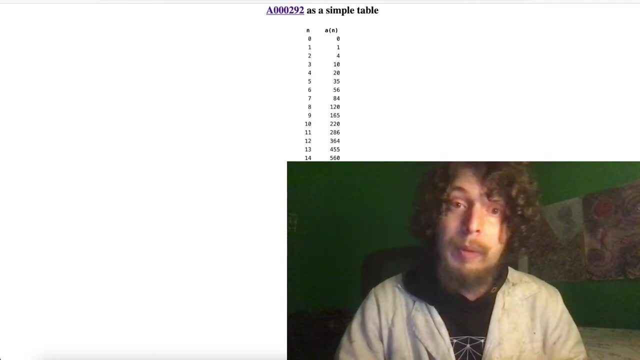 including a pretty long scene that got cut from the pan digital episode that i'll be editing just to put on the patreon in a day or two, which will be the core or seed of a future episode topic. but that's some of the stuff i put on. there is like bonus, extra stuff that gives. 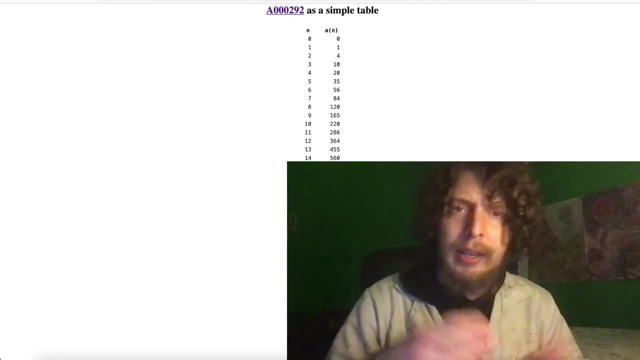 hints of the future or past, as well as thanking people in descriptions and as well as i'll put the soundtracks of a bunch of the episodes on there soon. so thank you to all my supporters there and thank you just to all of my viewers who comment on stuff and watch stuff. 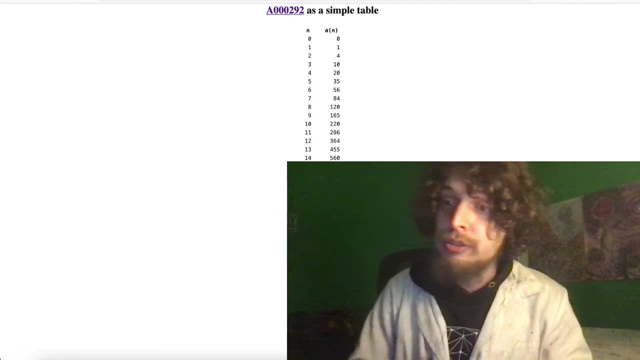 in the latest pan digital episode. one extra fun thing to look out for is there are three squirrel cameos got very lucky when filming that. normally in an episode you're lucky if you get one squirrel cameo back there. they run by a bunch but they do it so quick all the time we're there and a squirrel 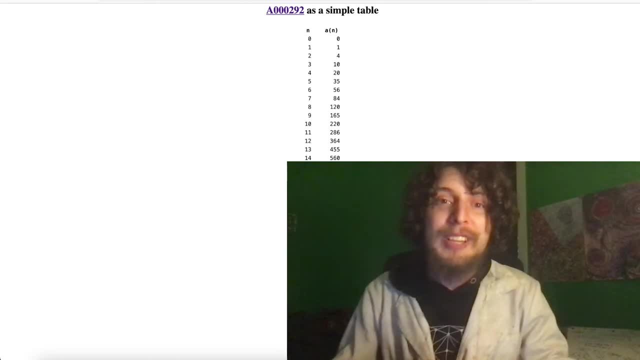 runs away on the fence and i'm like, start filming, start filming, and it's too late. but this time we were already rolling and i was already talking about stuff for three minutes and i'm like, oh, three different squirrel cameos. so that's fun. part of why i like having an outdoor classroom. 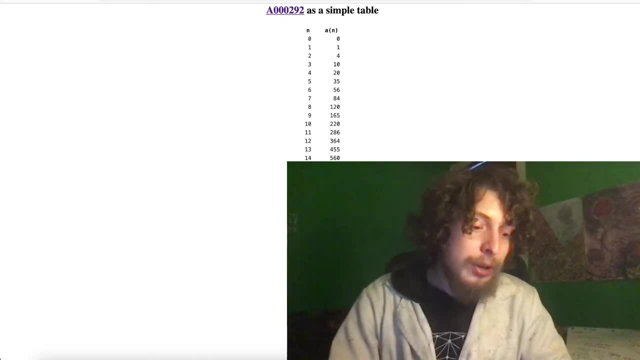 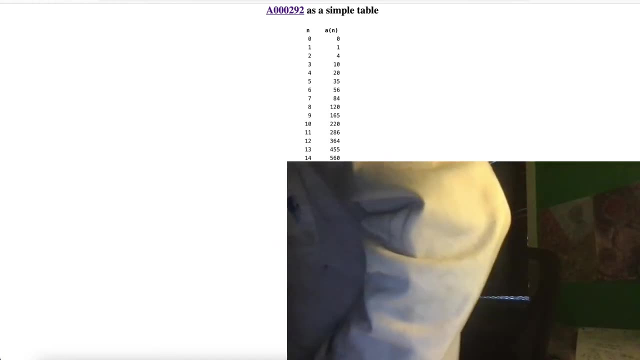 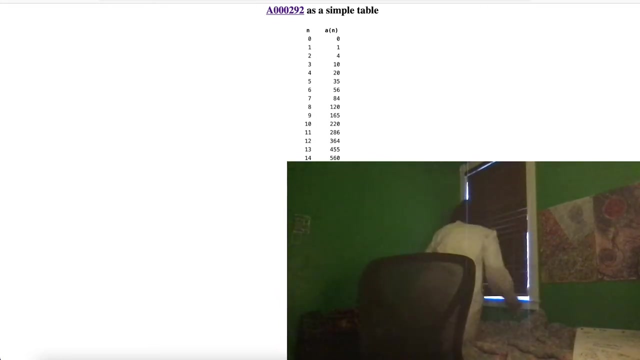 is those squirrel cameos as well as the bird song, and despite the fact that the rain right now- which let me check how it's looking out here, the rain's probably, uh, taking some of the clocks to their final stage. all right, not too much rain, but we are sprinkling, so we cannot take any sort of field trip out there. 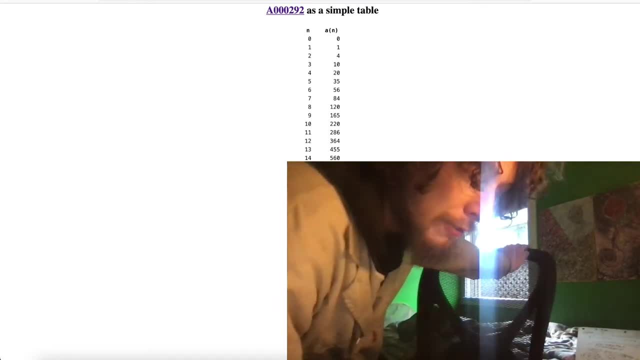 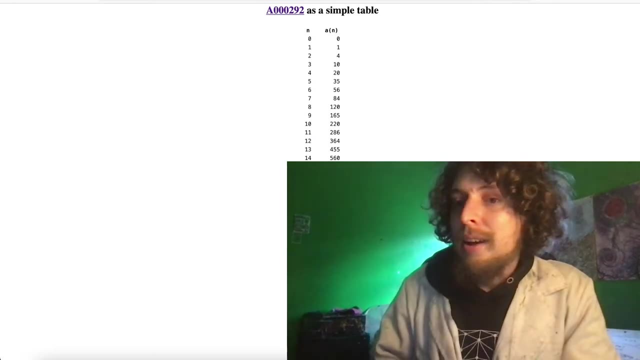 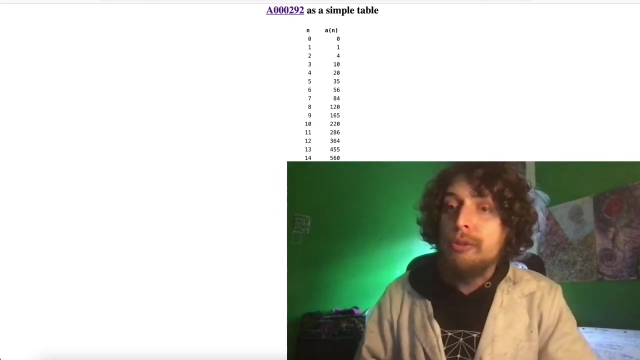 you know, small chance- we'll do a bonus video or something out there when there's a little break from the rain. um, in any case, i'm going to work on some writing in a little bit. like i've mentioned in the last stream and some other streams, i'm trying to do a little bit of writing. 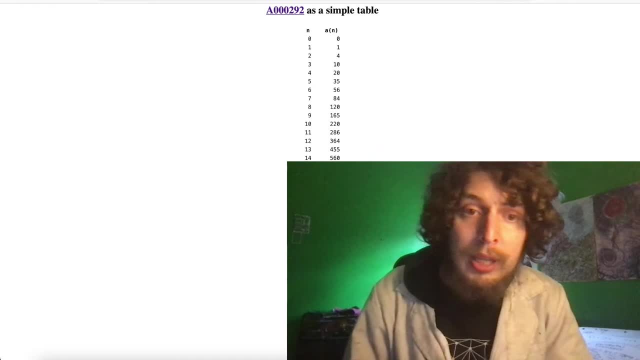 to as i transition to spending more time as combo class, hopefully being my job, and so on. part of that, uh, although it won't detract from the videos, because i will still have more time to make the videos than ever- part of it is also writing things that i want to publish and eventually, a lot of 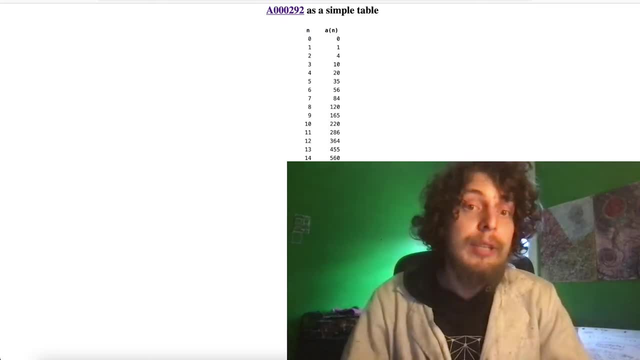 them may be free online, or i might sell paper copies of them, uh, or things like that, but i just want them to be read, and some of the ones i'm working on right now are a very surreal fiction story and a book about threvens and throds, as well as a number of other. 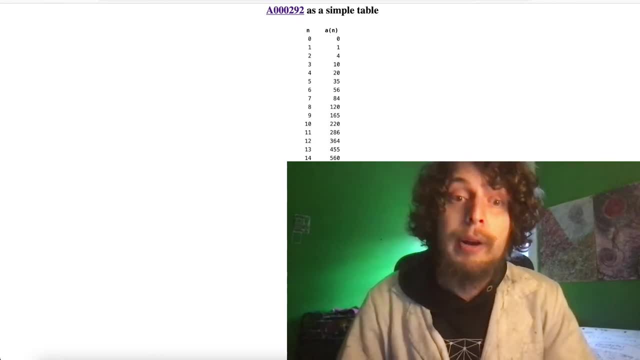 projects that i get usually more carried away in my brainstorms and i'm better at coming up with ideas than finishing the projects. i'm a little perfectionist about my books for some reason, compared to my videos, but that's something i'm going to work on a bit today. 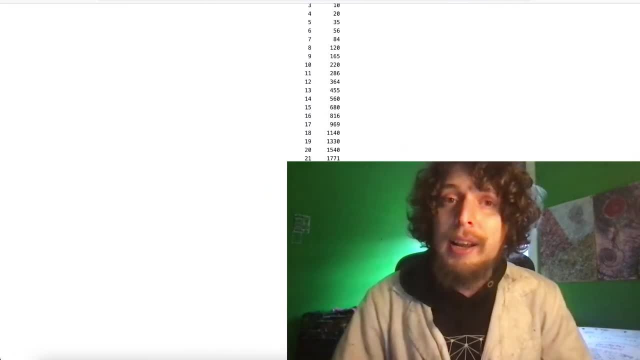 so i will be, during part of that time, culminating some more fun facts about threvens and throds and some of the things that i'm going to be working on today, and since one of the facts i'm going to take notes about, i remember seeing a good chart of 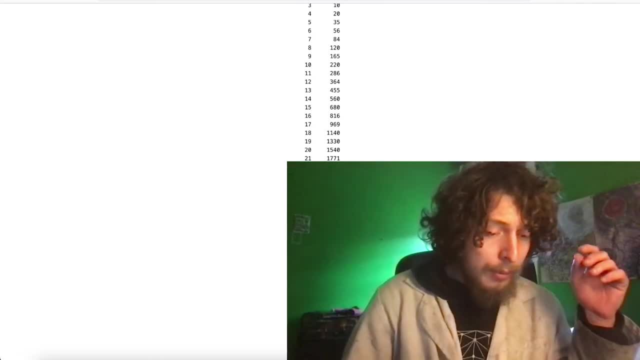 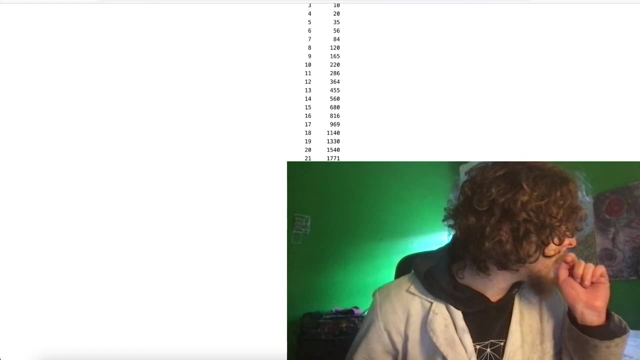 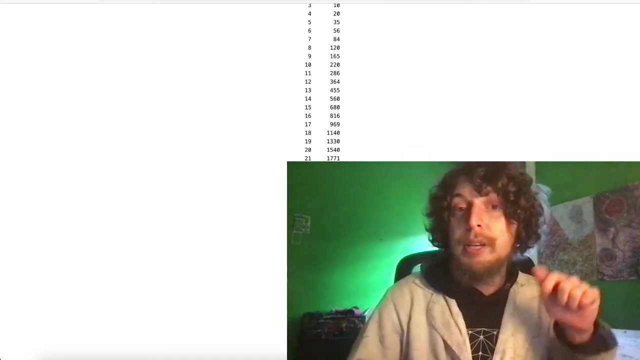 in one of the books i have here about number theory. i might grab my number theory books for a moment to show you one of the um things from there. and thank you so much to quinn for taking down some notes about when stuff happened in a time stamp. if you can copy that to. 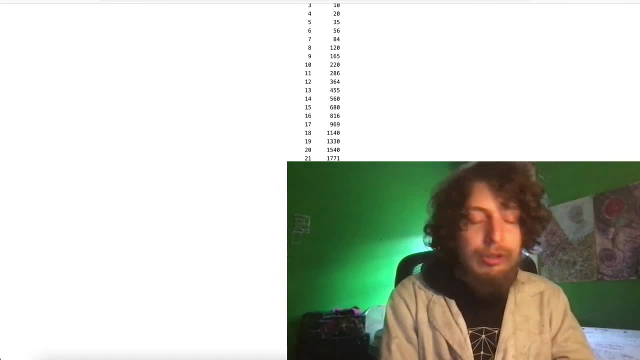 post like on the stream later, or i'll also screenshot it here now too, uh, but if you can post it in a comment after the stream posts, that'll be extra helpful, even if it's not fully complete. uh, and like i've mentioned before, if people ever want to help out, like with that like, 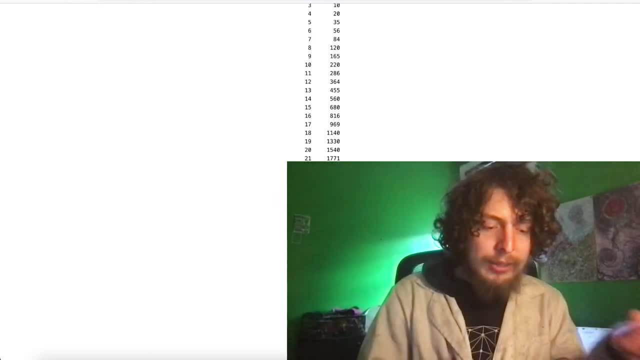 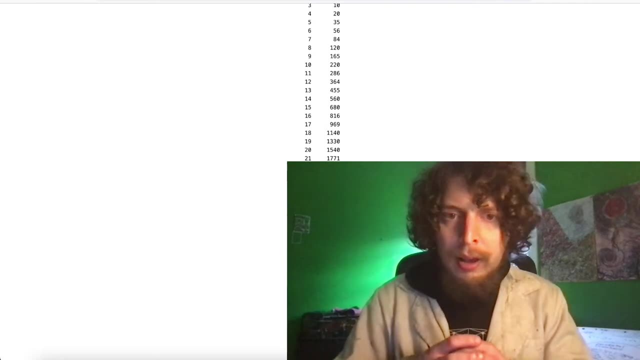 quinn's doing of um taking notes of when stuff happened. that's very helpful for future viewers and i will like pin your comments or whatever to make it a little bit easier for you to read. and i'll see you in the next video. and i'll see you in the next video. 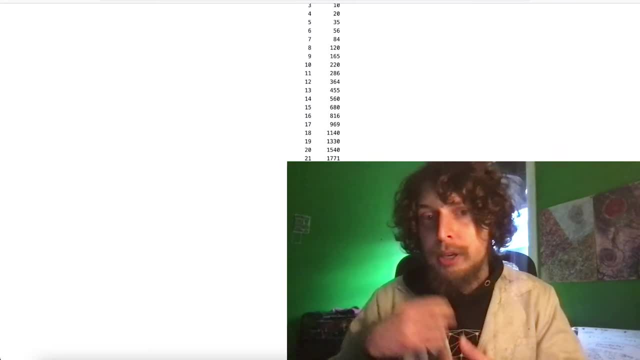 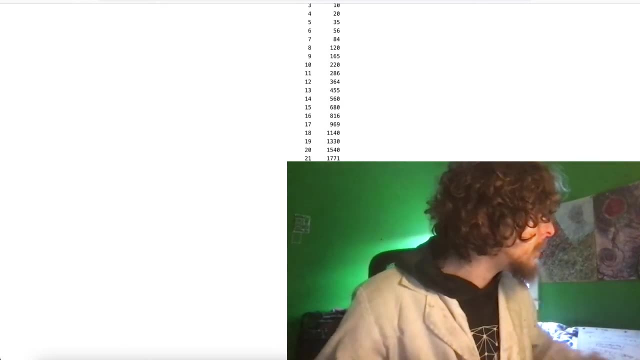 extra helpful for future viewers, or viewers who missed part of the stream, to click around to whatever topic they liked. and um, taking a look at one little number theory book right here briefly before i close off the stream, because i want to revisit this chart to take some notes on. 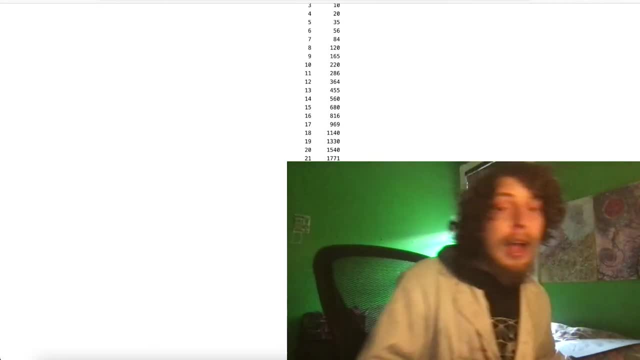 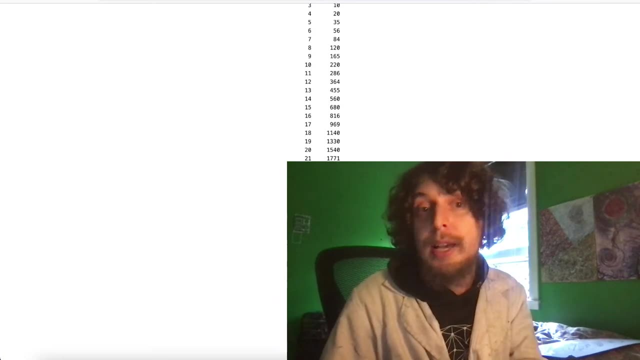 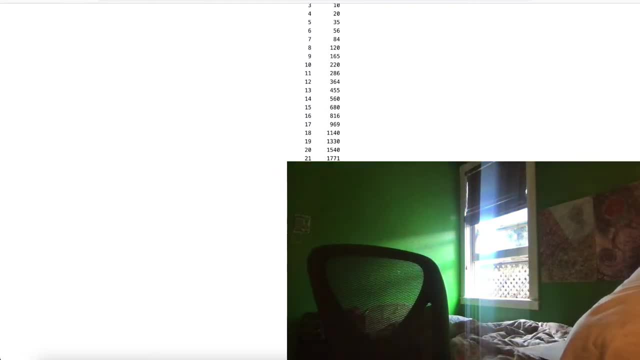 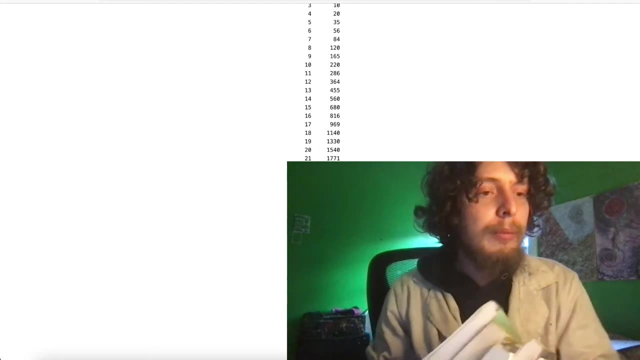 i've already promised a type of stream of me showing how to make digital beats that i never ended up being able to get around to that. i will do that one before long. that'll be fun, showing you guys how to make a beat from scratch now out of all these awesome number theory books. 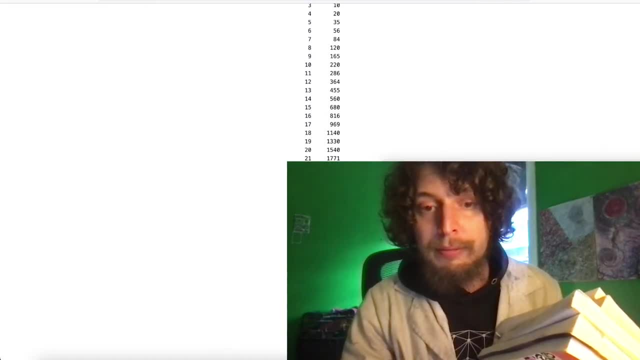 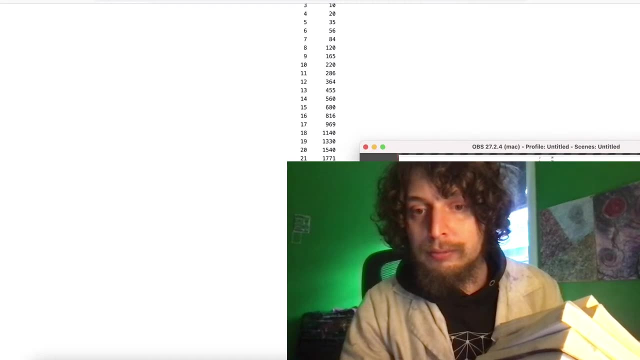 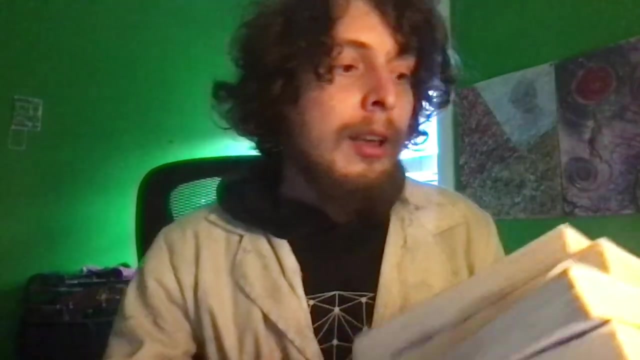 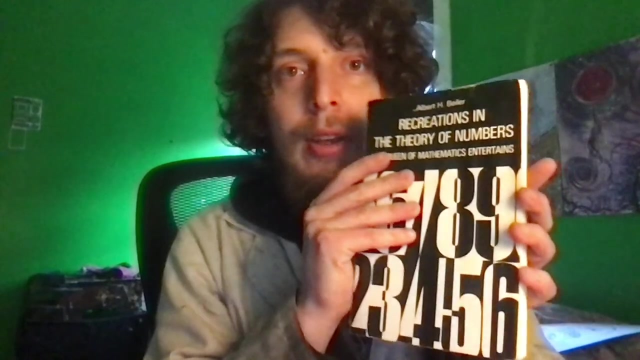 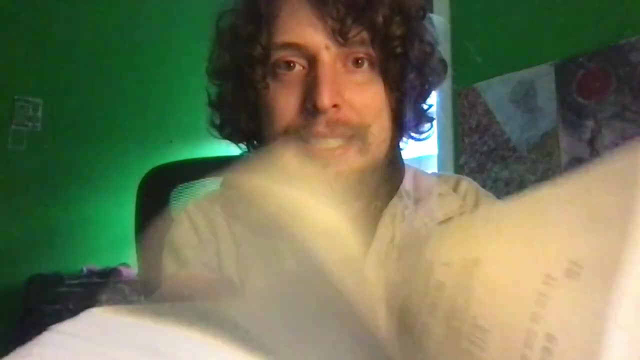 which i'm now going to make full screen. um moment, with all these awesome books, uh, one of them that i've been especially liking is this one: recreations in the theory of numbers, packed with interesting facts and stuff, and this book got mildly rained on. oh, that's bad. you hear this. okay, no, it's now. it's good, but the pages were. 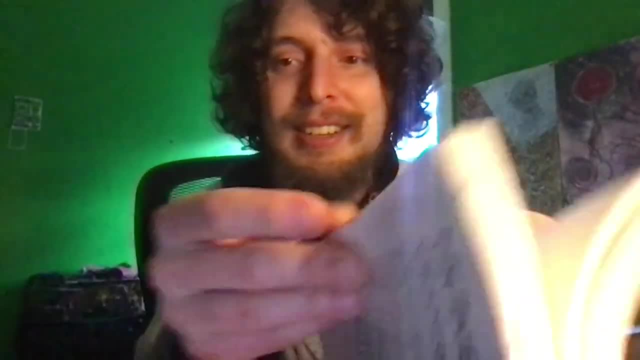 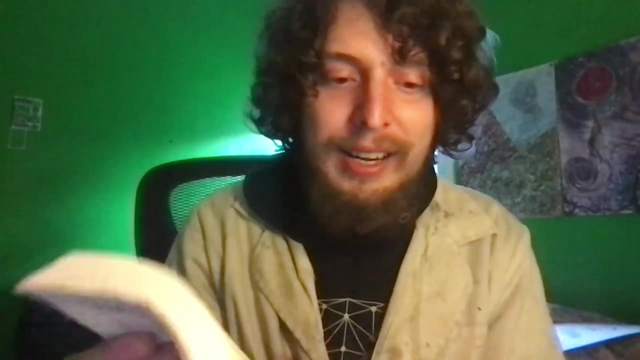 actually good, so i'm going to show you guys how to make a beat from scratch now out of all these. and kind of weird, you hear these. that's not a good sound for a book. yeah, these all got mildly rained on, but i think they uh got dry enough that they won't grow mold or anything. so who cares if they're a little warped, they get the job done. now, where is this thing i'm going to look for? now, if we're looking at things like triangular numbers or the family that triangular numbers and square numbers are in, called polygonal numbers, which are the numbers that there are multiple ways of. 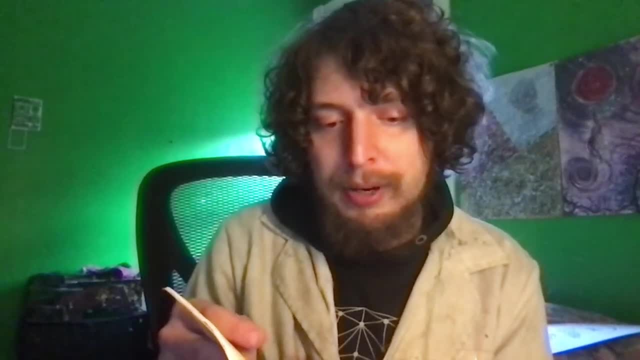 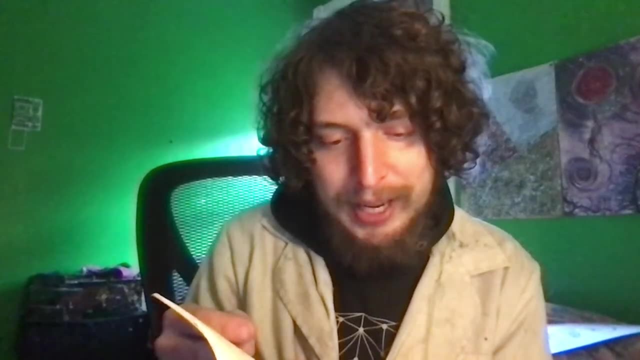 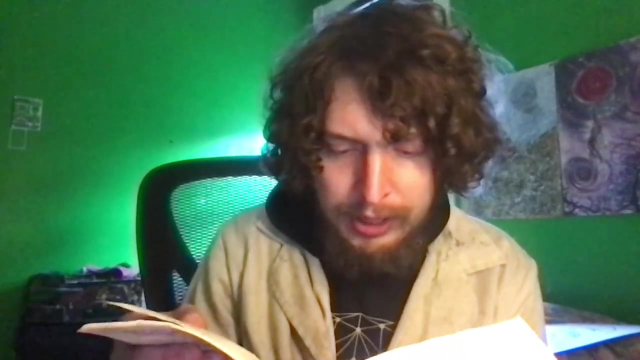 defining them algebraically, but in a sense they're the numbers that if you made that amount of dots it can be arranged in that shape, following you know certain rules for how the dots have to be placed and jumping to some of the things they have here about our polygonal numbers, 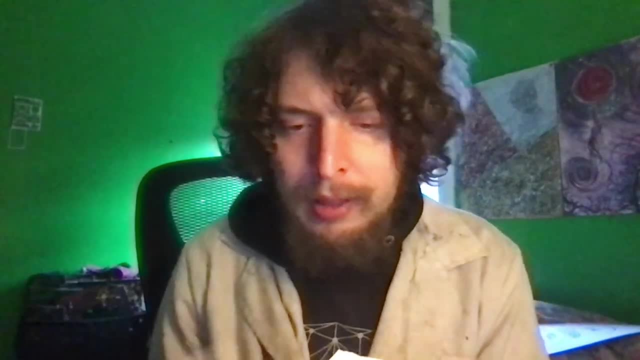 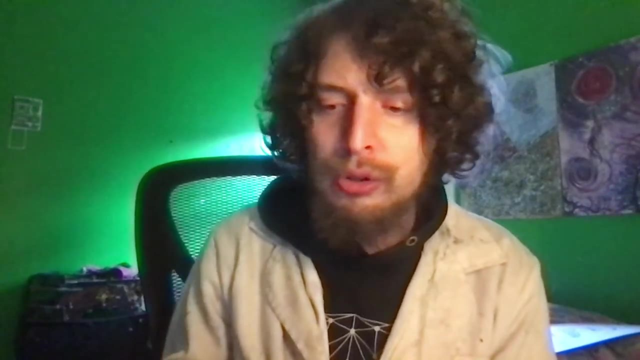 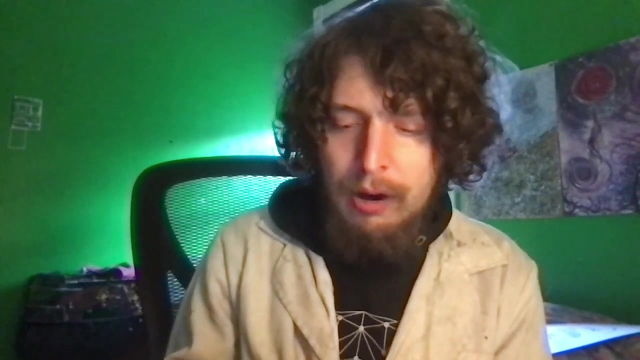 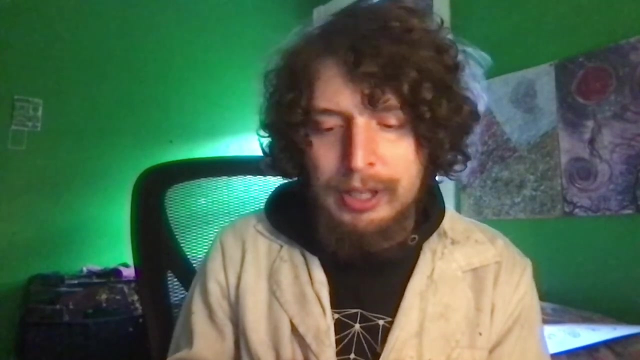 they had some very interesting charts in here that reminded me of some cool traits about three of the numbers, as well as some cool traits about square numbers, and we often think about square numbers as being: oh, you get them by taking x times x, that's x squared. but square numbers can also be seen as: 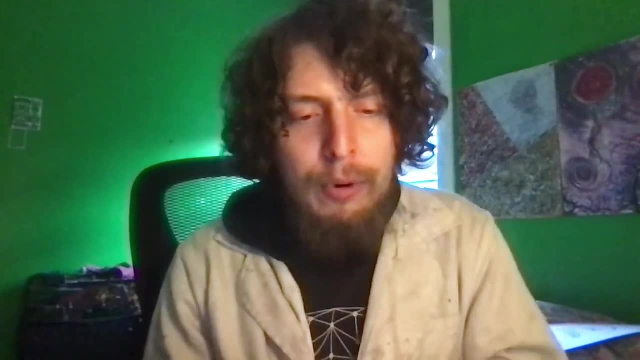 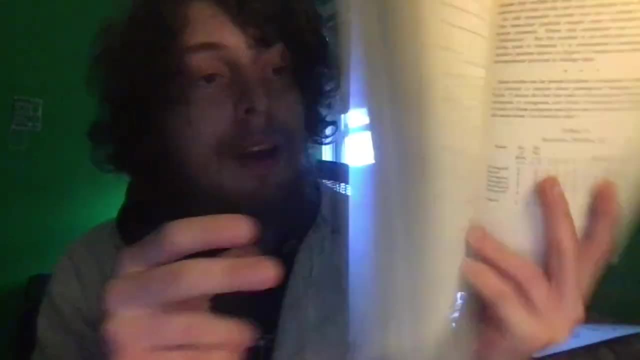 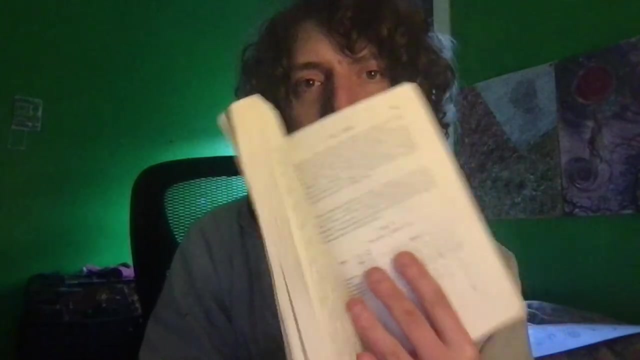 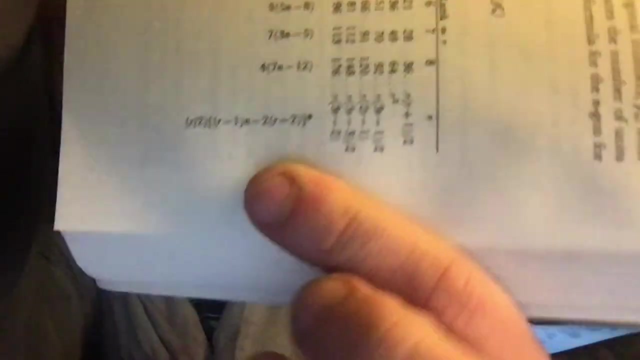 just the four-sided variety of what are called polygonal numbers. such as these polygonal numbers and if we look at the equation for polygonal numbers and how many dots would be in one, the generalized equation here is pretty complicated. there's one way of writing the 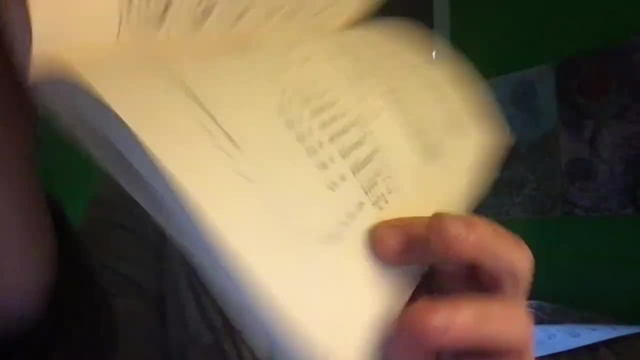 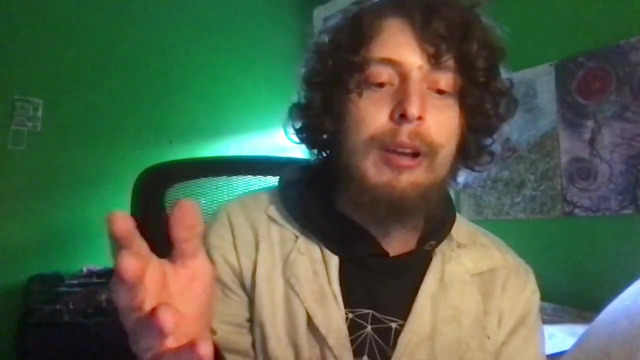 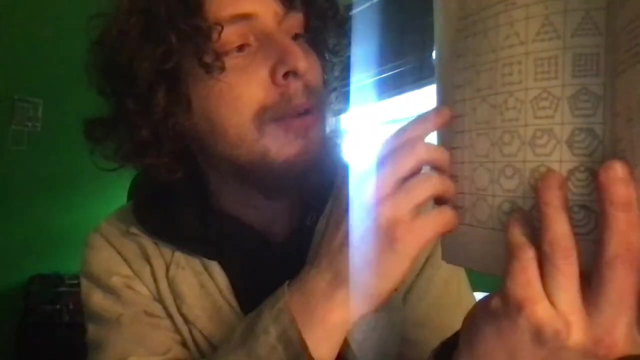 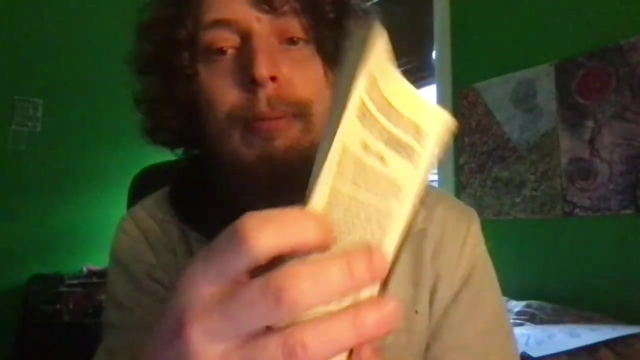 generalized equation. but what happens when i plug into that generalized equation which has one variable for how many sides we want, like the n gone, numbered on a pentagonal would be five, hexagonal would be six and the other for which level i want? how many stages into it i want? 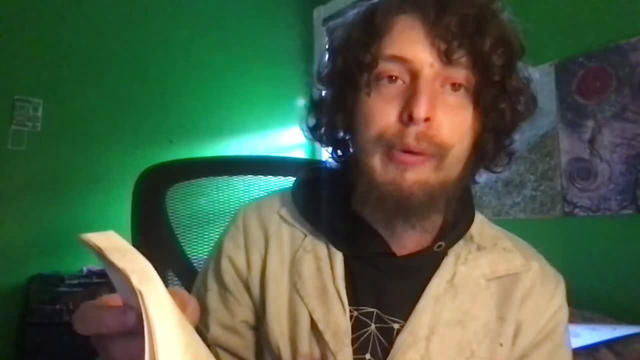 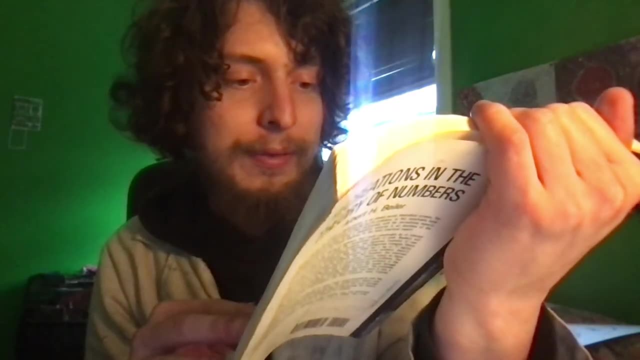 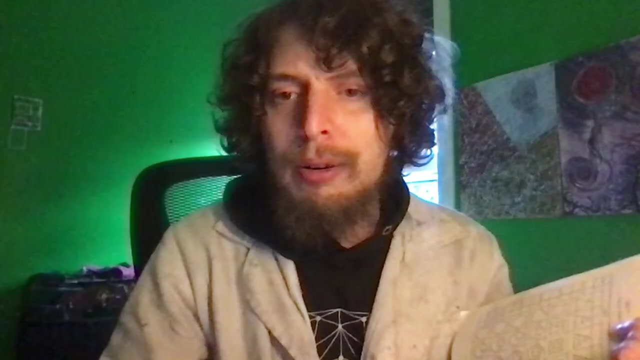 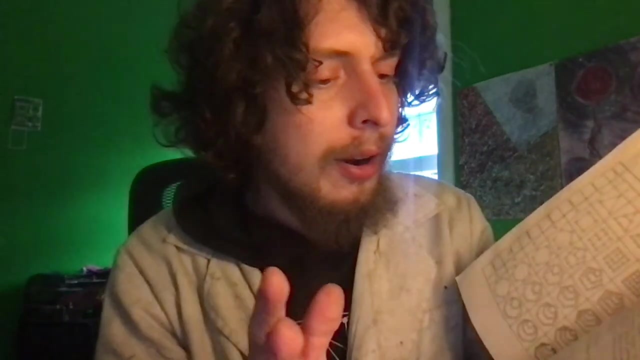 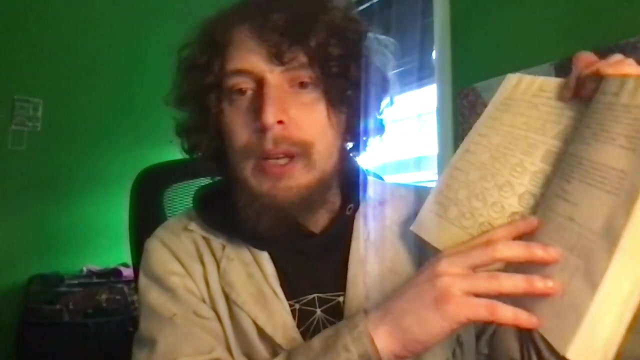 well, when i plug in four sided for the level i want, which is square numbers- that crazy wacky formula right here, let me see where we're freezing. oh, no, sorry. yeah, n squared can be seen just as the square being lucky. oh shoot, we're freezing again. okay, the stream will be ending soon. sorry for the. 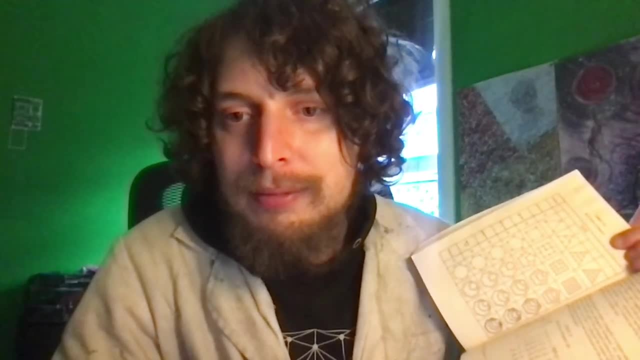 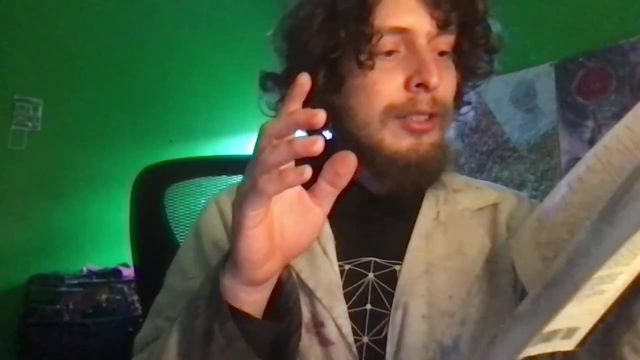 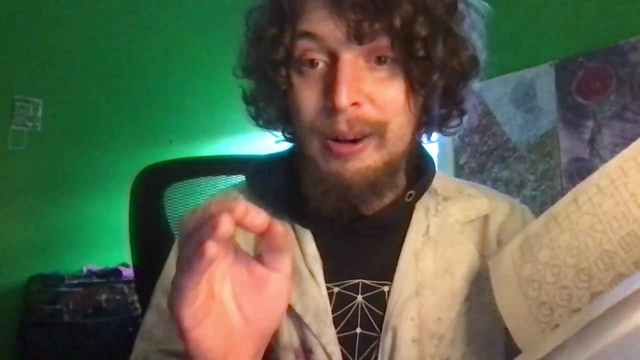 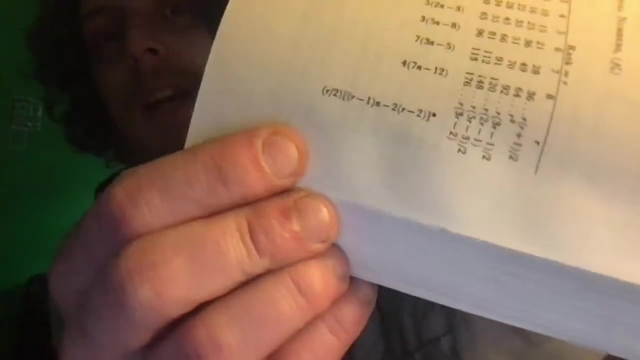 freezing, but um uh sorry about the glitchiness in the last couple minutes here, so assuming this is still hopefully going the square, sort of just got lucky that this crazy formula that i'll show in a clearer form in a full episode before long simplifies when you plug in four to it. it. 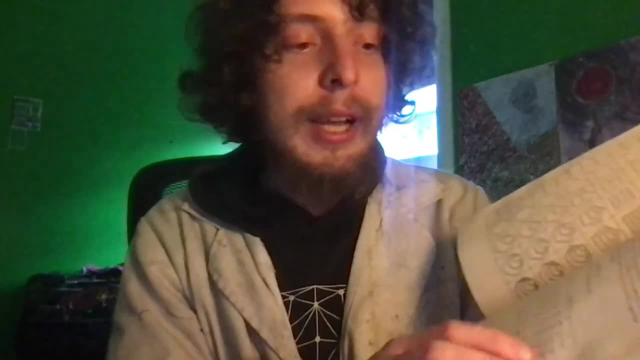 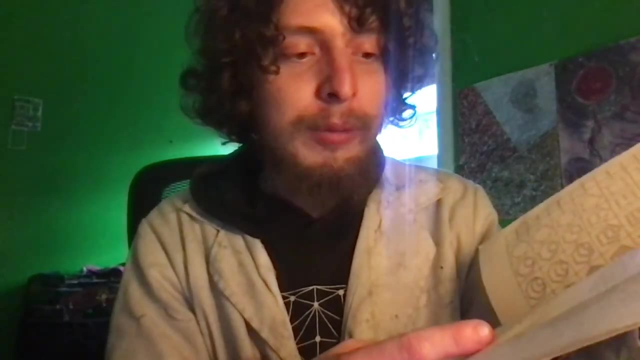 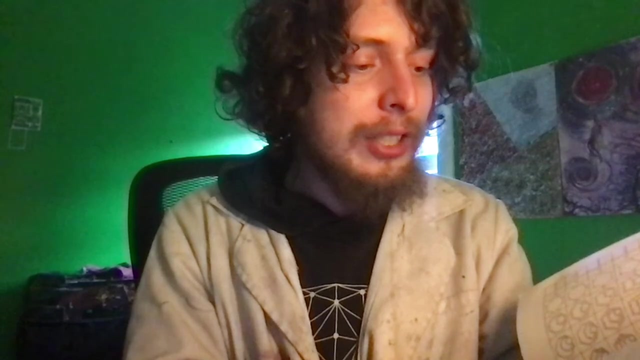 goes down to r squared here. the triangular numbers got a little less lucky. their formula simplifies to r times r plus one. so if i plug in four to it, i get a four squared here. if i plug in two, three, all over two. So we'll go into this in a future episode, that there's a weird way that the squares 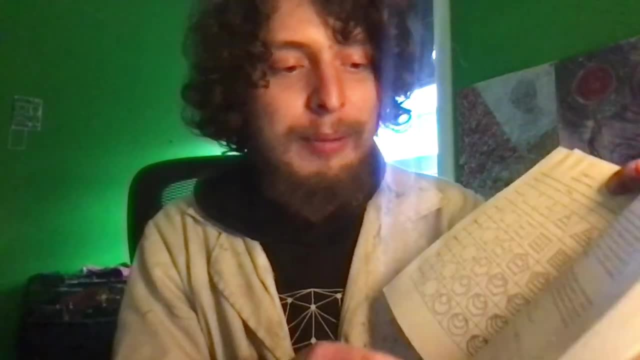 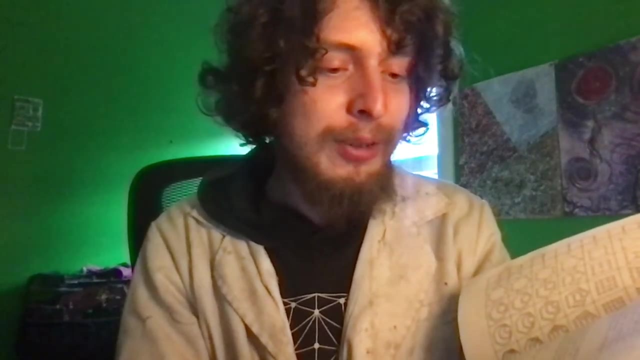 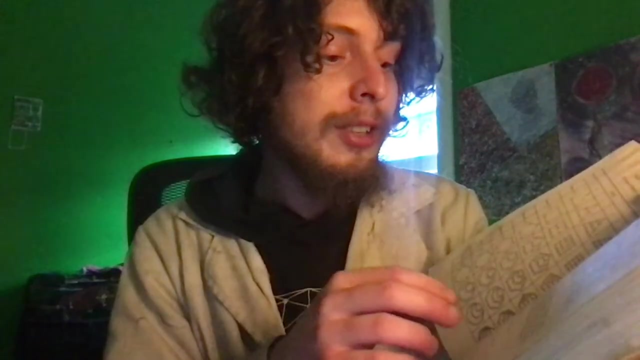 just got lucky with their equation simplifying to something times itself, So you can sort of approach from a backwards way why squares are that? And there's many ways of defining what a square number is that we will go into later. And the thing about the Riemann's I wanted to note. 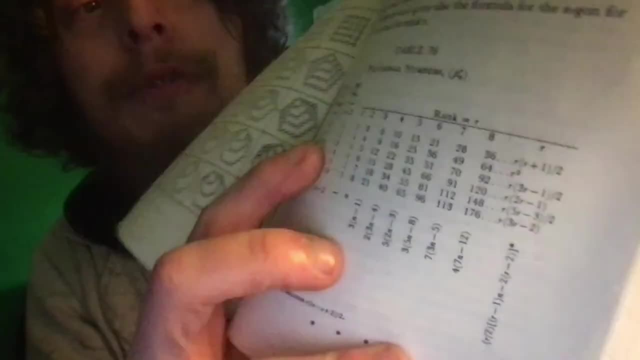 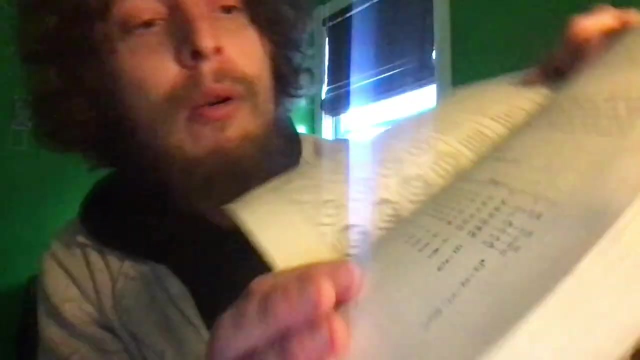 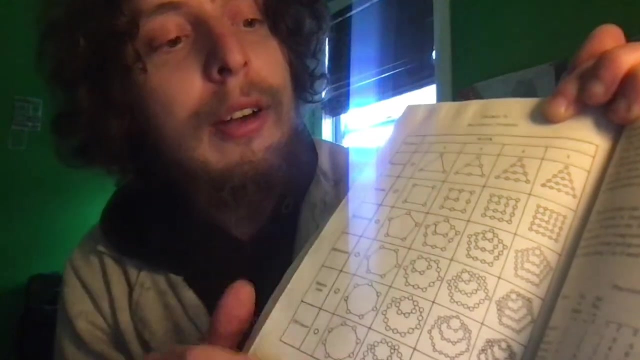 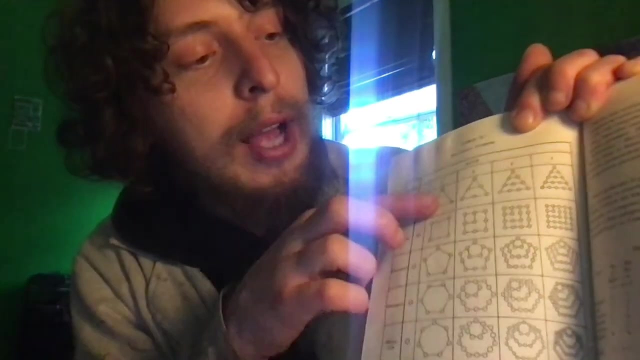 here is that. here's the chart that's shown for these different types of number, four different levels of them. how many dots are in a certain thing? Well, we'll notice that on the first level they all just have one dot. On the next level, they have the amount of dots as what. 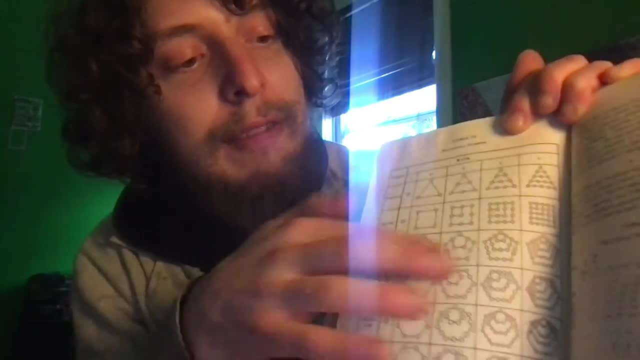 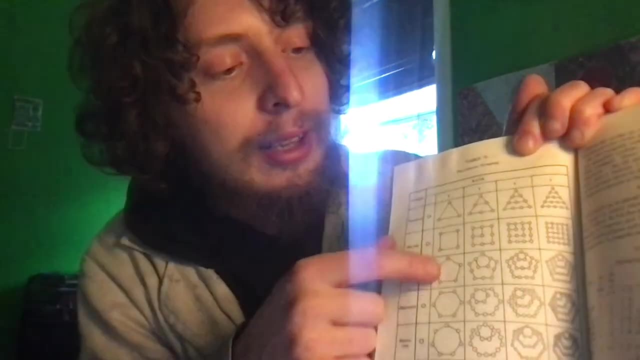 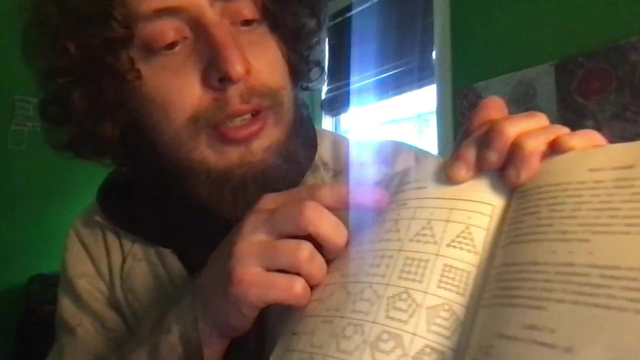 like not level into it, but what level? Which? if we're like a five gone which is a Pentagon, then it'll have five for that second level. And then in the third one, let's see what happens: Three there, six there, nine there. 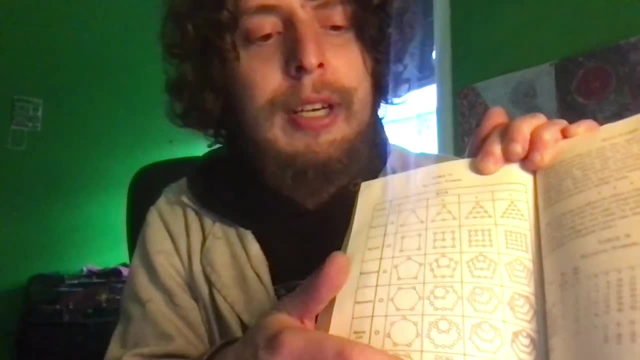 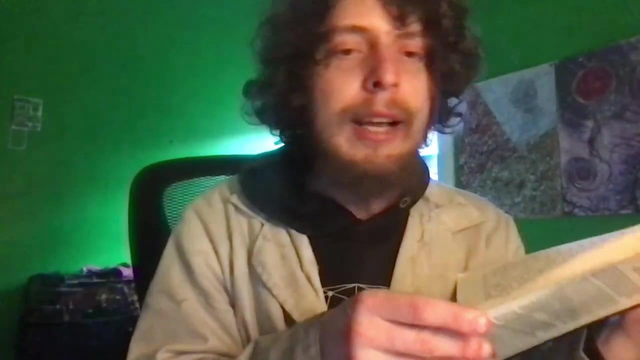 12 there, 15,, 18,, 21.. It's the Threven numbers, amount of dots on the third cell, And at first you might be like, well, that doesn't sound that interesting. You got the Threven numbers because 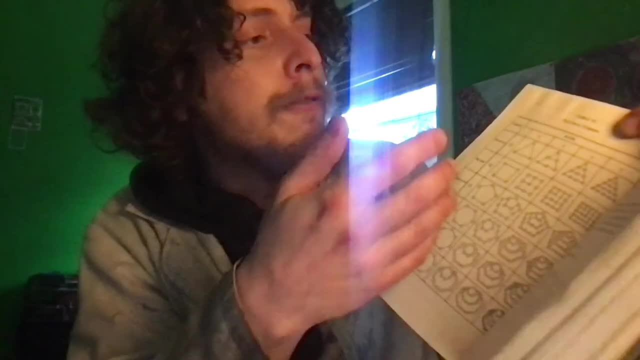 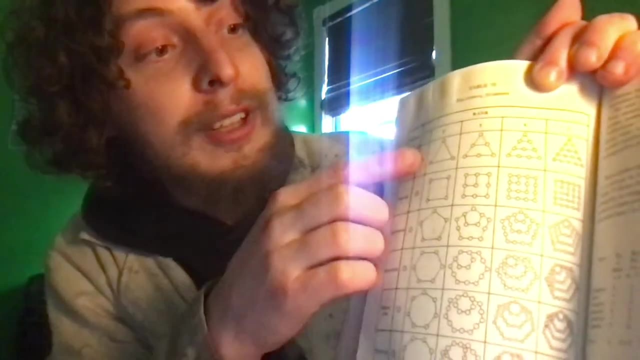 it was the third cell And at first you might be like, well, that doesn't sound that interesting, But that's not true for any of the others. Even numbers are not the second rank. Natural numbers, all of the natural numbers three and above, or two and above, if you counted these. 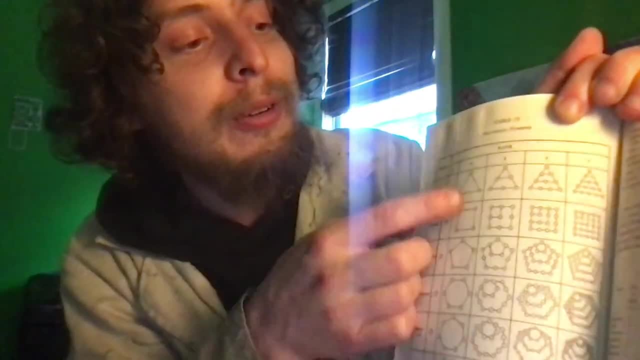 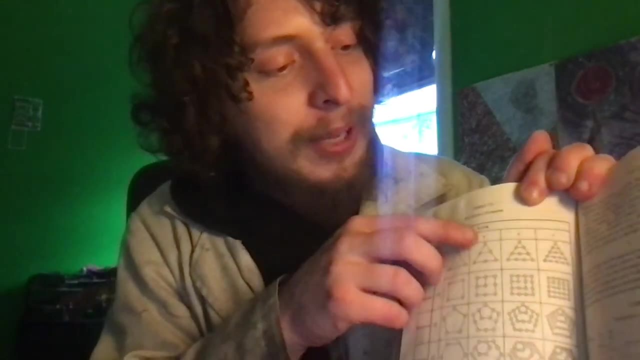 linear numbers or point numbers or one. you could try and start it there too. All these natural numbers are the second level. A series of ones is the first level And from here, Threven numbers being the third level are the only, like some, 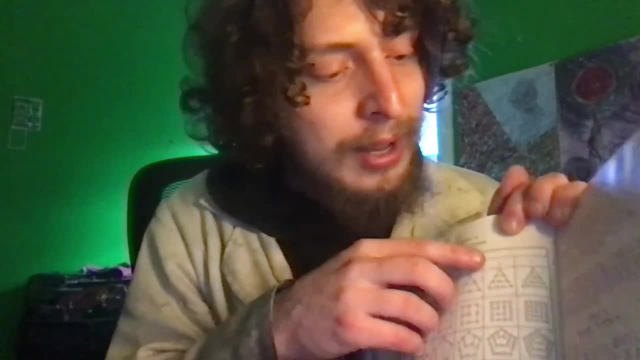 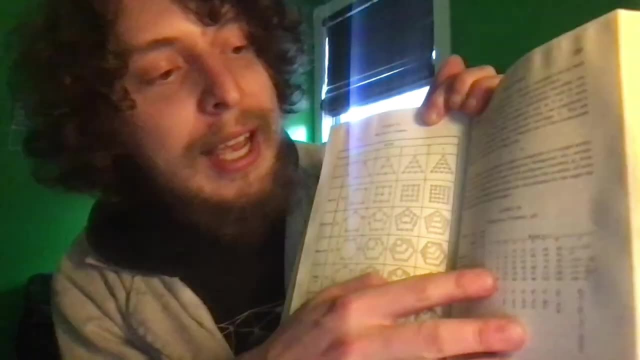 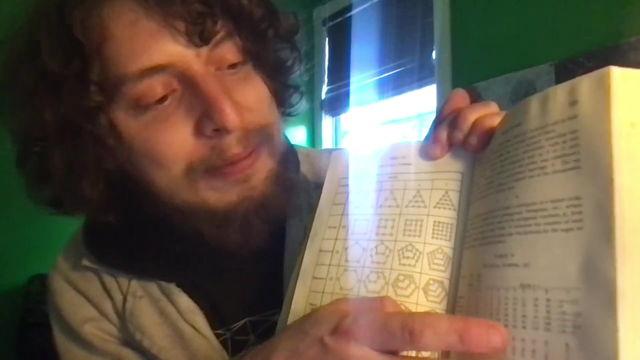 multiple of something, one that happens in such a clear way. Level four is not just the multiples of four. It goes four, then 10,, then 16,, then 22,, then 28.. They're six apart from each other, but starting with four or 10, starting with 10,, depending how you look at it. 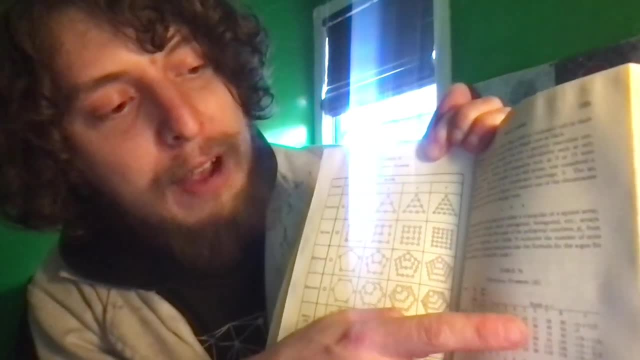 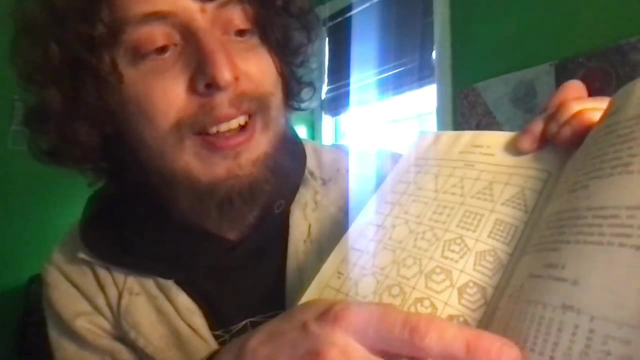 And so all the others. here it looks like we go five, 15,, 25,, 35.. For the fifth level, they're going up by 10 in each time, but they don't start on 10.. So it's not. 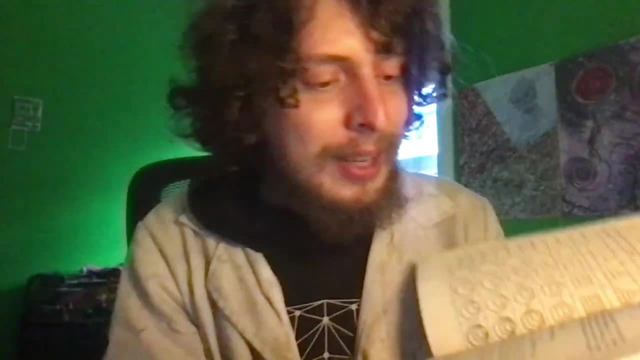 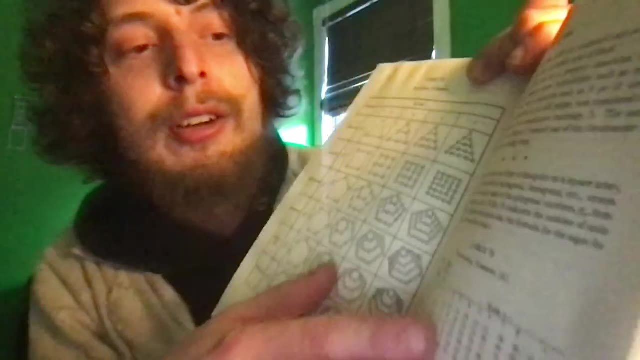 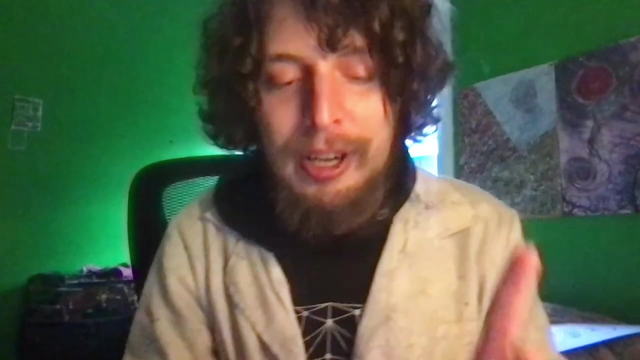 they're not the pure multiples of it And so you have weird jumpiness on the other ones if you had to figure them out. But on the third level of each, it's just the pure Threvens, not what I actually know. It's just the Threvens. I'm not going to say pure because I actually 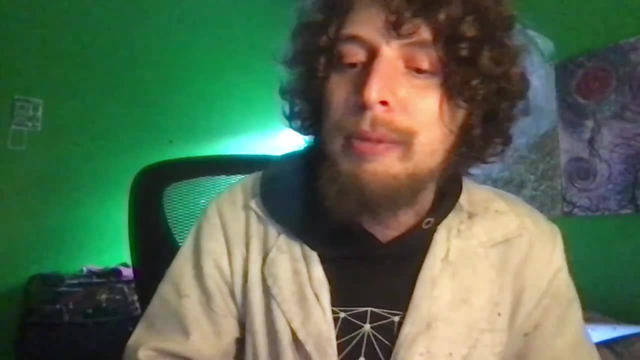 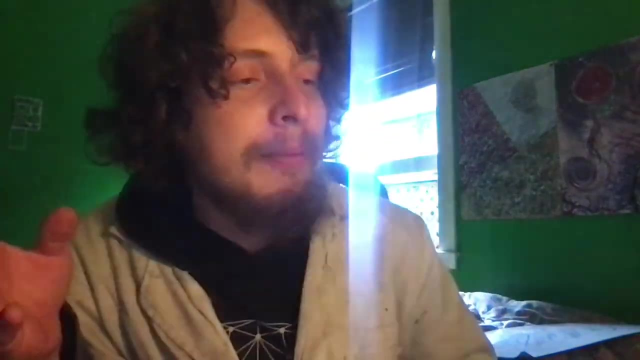 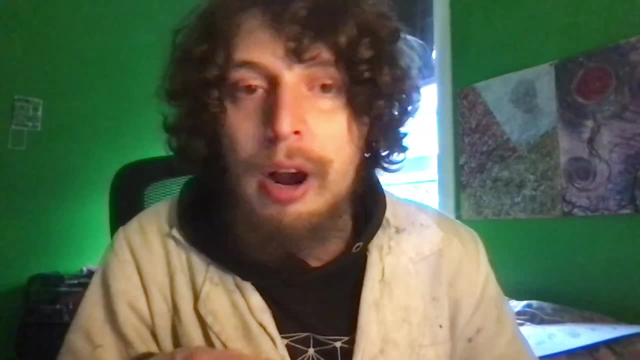 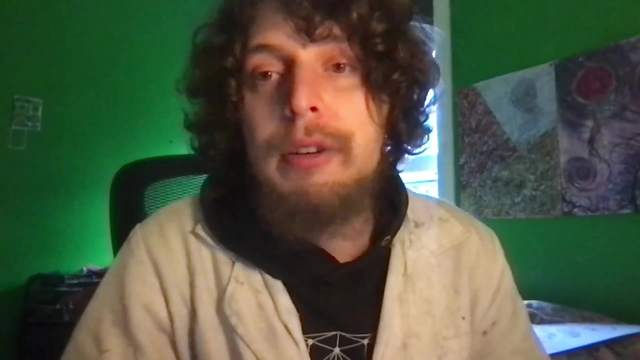 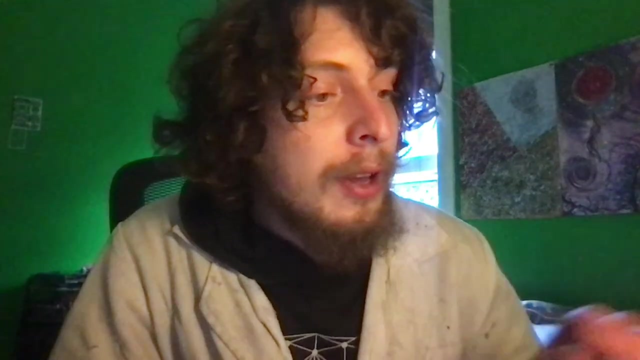 and so that's a place where Threven numbers show up that evens don't, So Threvens don't always just show up after you've already analyzed evens having a cool trait: Sometimes the Threven numbers show up on their own regard, and they should have shown up in many episode topics similar to how. 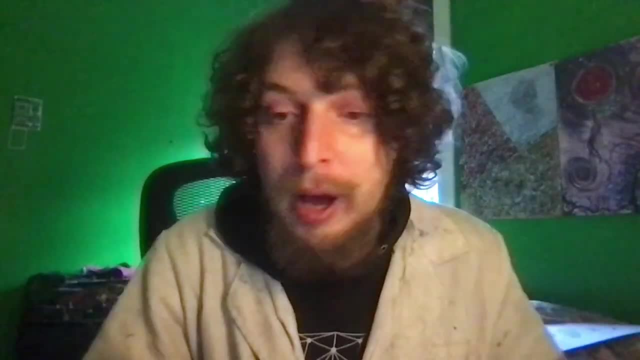 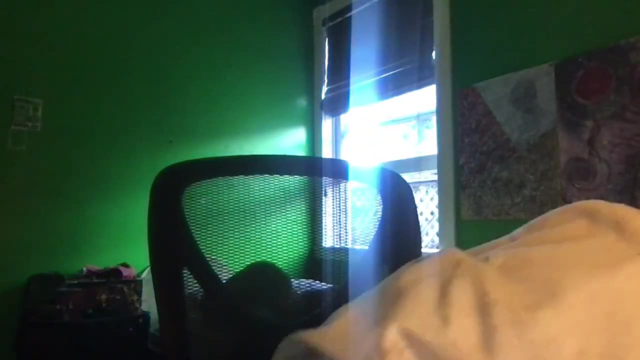 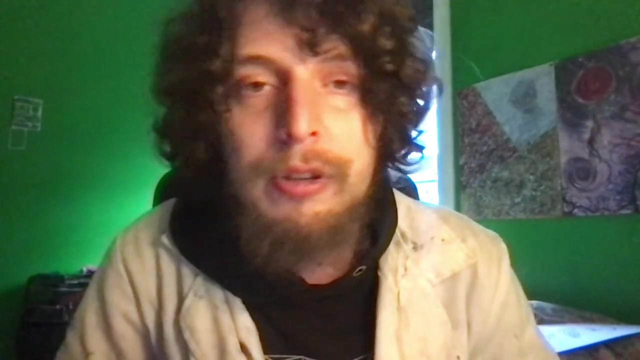 hyper 11s keep popping up, factorials and triangular numbers keep popping up, Threvens keep popping up, And so that's something I'll be taking some notes about in my writings. today is some ways of putting that in the context of other things, And it will show up in an episode before too long. 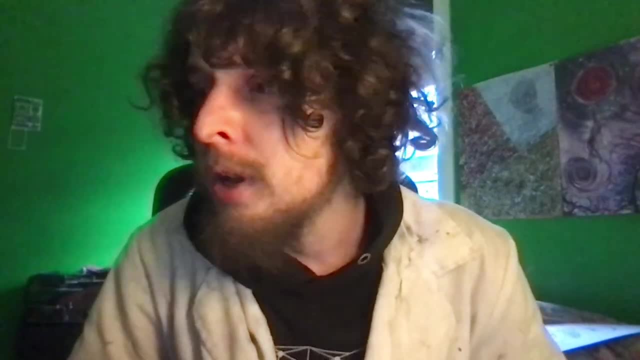 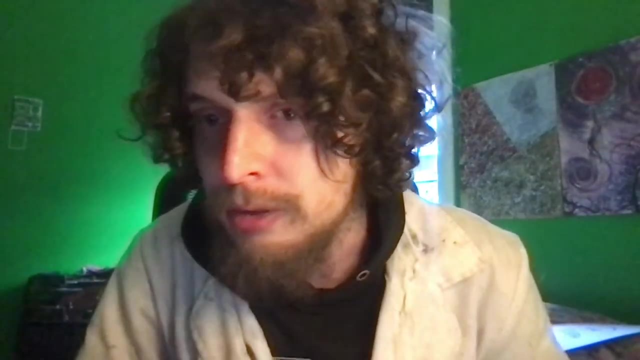 because there will be multiple episodes in grade negative two, probably a whole little separated mini series of them. that will be about polygonal and polyhedral numbers and in general what are known as figurate numbers. that are like that. A lot of interesting patterns there, similar. 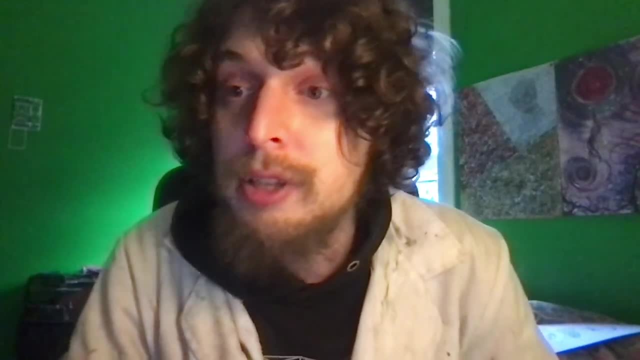 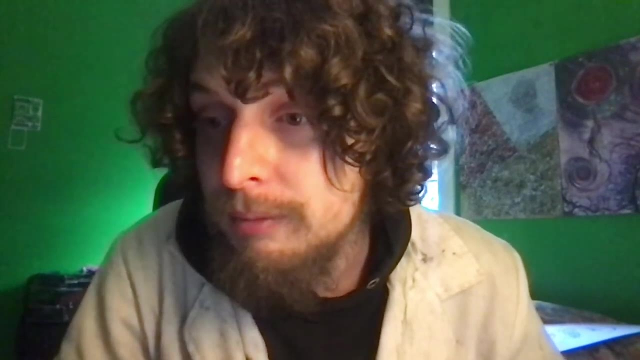 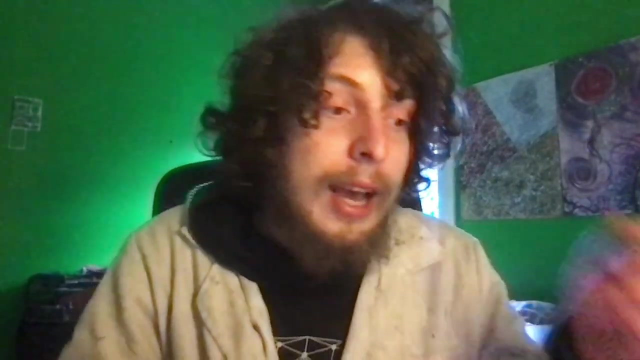 to this tetrahedral number sequence that was on the screen before and similar to what's really going on in those charts visually. So thank you all, and whoever said they barely understand, but still said thanks, that's okay. I like when people who don't understand the videos watch them too. 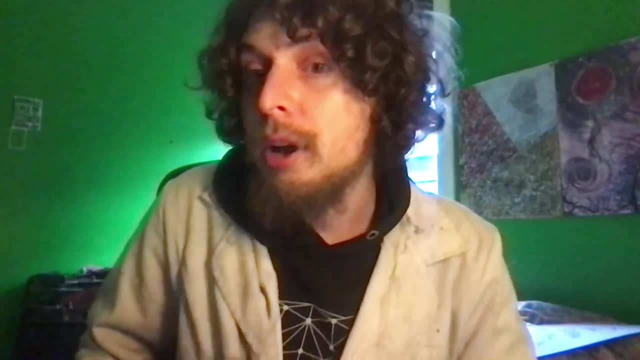 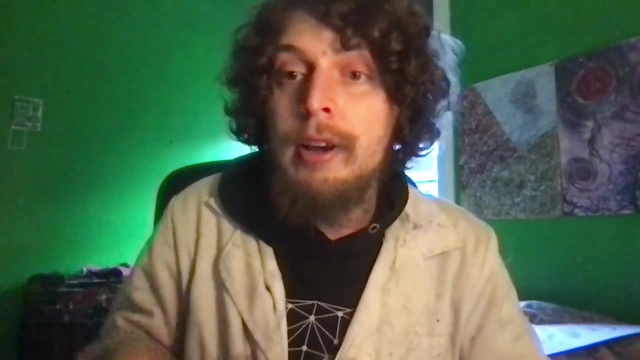 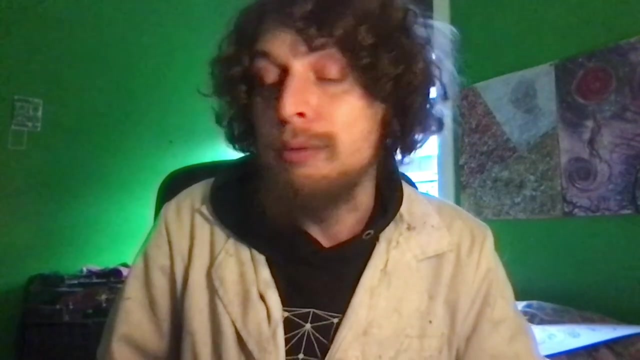 I think it's still good for your brain. I sometimes try and digest content that I find trustworthy and fun, That I don't fully understand. For example, there are some mathematical papers I try and read that are above the level I understand, that are just really deep into some field or another's language. 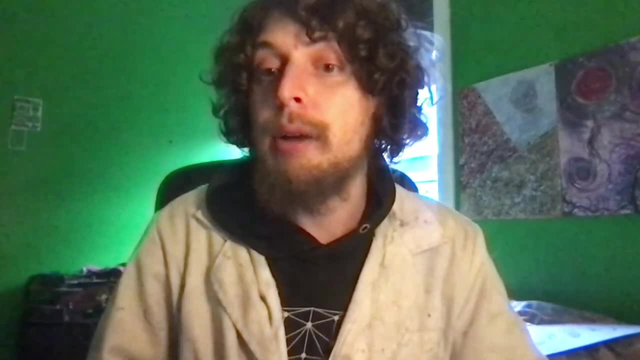 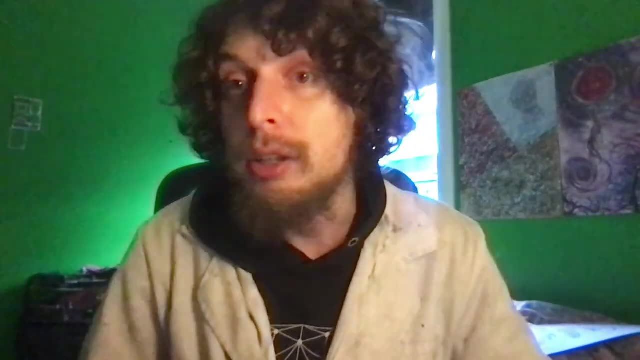 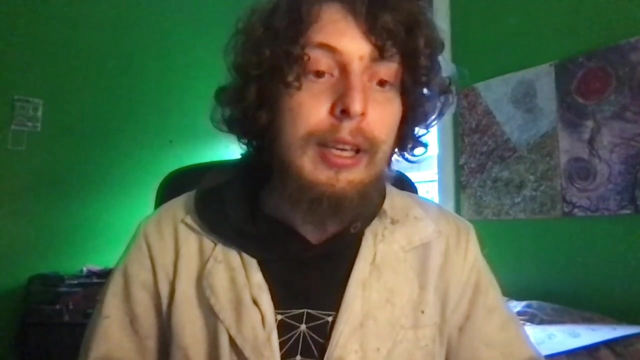 And I think it's still good for my brain. And when I was first getting into math, I remember watching a bunch of like videos on channels like 3Blue1Brown and Mathologer that I didn't fully understand. And now, going back, I love watching the videos and understanding them and thinking.